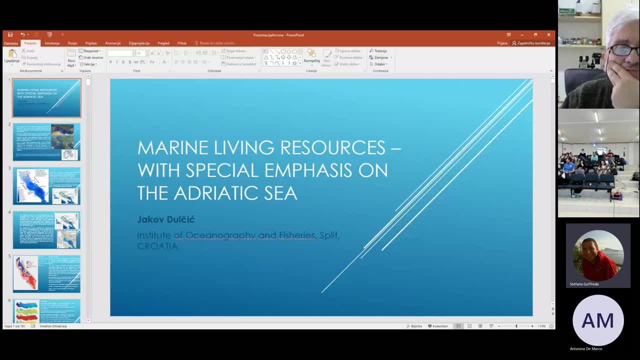 I'm glad to introduce you, professor Jakov Dulcic, from Croatia. Jakov is a member of our academic board since the beginning of this PhD program and he's the head of the laboratory of ichtiology and coastal fisheries at the institute of oceanography and fisheries in Croatia, And. 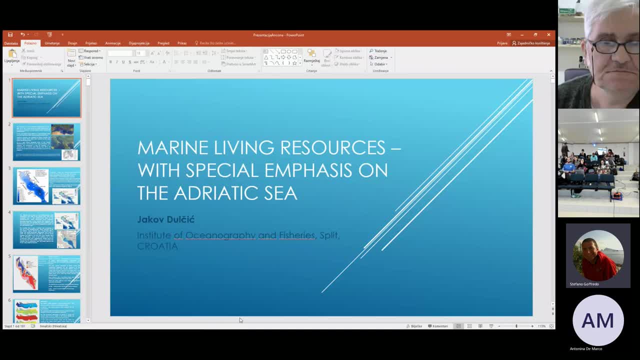 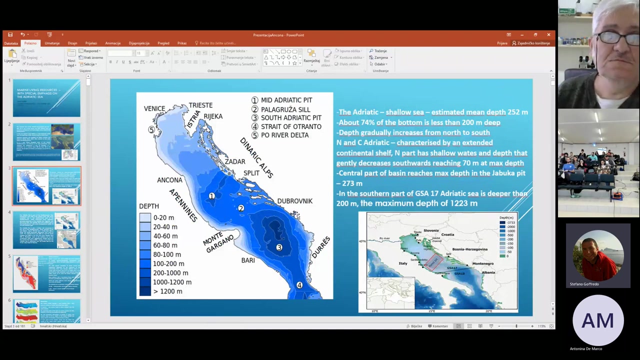 he is also a zoologist and, of course, a marine biologist and ecologist, and he's specialized in the Mediterranean problem and especially in his performing research in the Adriatic and along the Croatian coast, And he's working on changing in fishing and marine biology diversity during the last few years. So I'm glad to have with us Jakov. 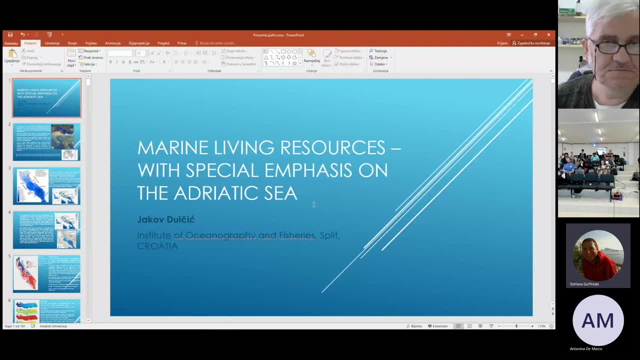 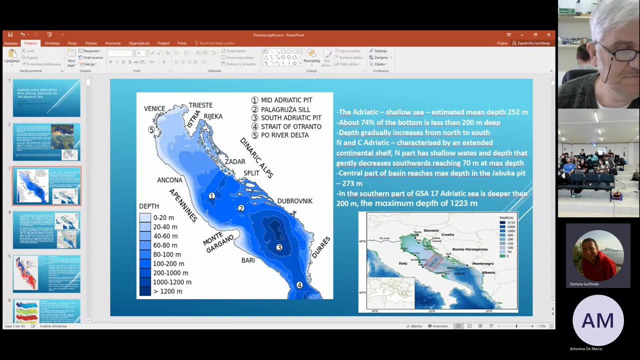 And I invite him to start his lesson. Thank you very much to everyone, To Mariana, for the technical assistance, which is not banal. Jakov, it's your stage. Okay, You for sure see my presentation on the board. Yeah. 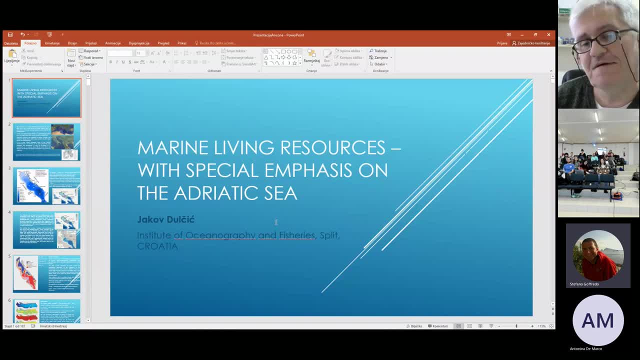 Bye, Bye, Bye, Stefano. My microphone, Yes, Yes, Yes, We see the presentation. Everything's working Okay. Thank you for your introduction and few words about me. I am working in the Institute of Oceanography and Fisheries in Split Spalato And, even though I'm currently in the 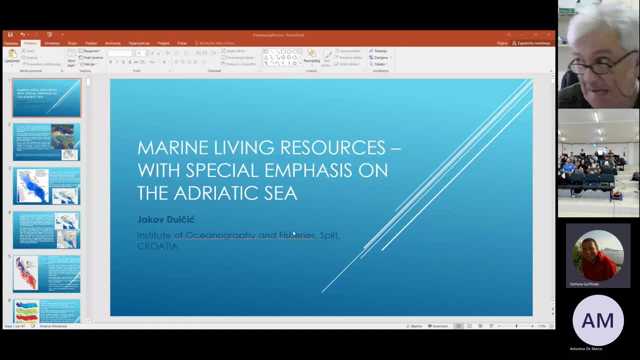 So Stefano said that I am a marine biologist. Yes, I mean, I am a marine biologist, but primarily I'm an ichthyologist, So my occupation are mostly fishes as the objects of my investigation. It means I'm trying to get much more information. 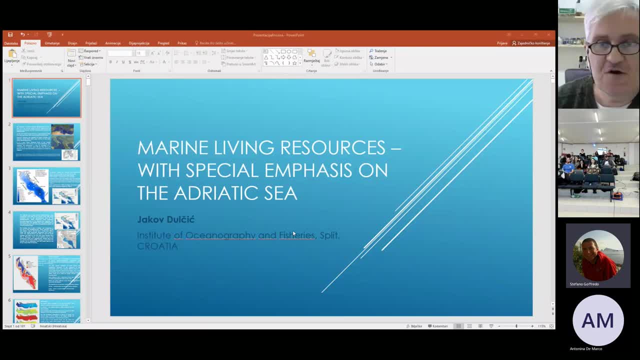 or my investigations about the biology and ecology of fishes And nowadays, especially, about the ongoing process of changing of ichthyofauna, not just of the Adriatic sea, even though the Mediterranean sea, And if we, I think that we will catch the time. 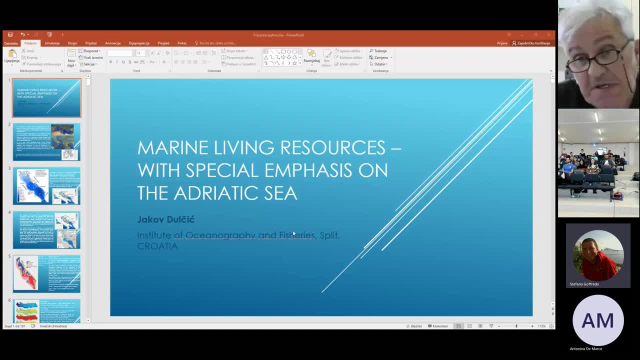 and I will show you at the end, or maybe earlier. it depends. It's on you and me, of course- to say a few words about the changes which are now going on in the whole Mediterranean era, especially in fish fauna, ichthyofauna, which are now, let's say, 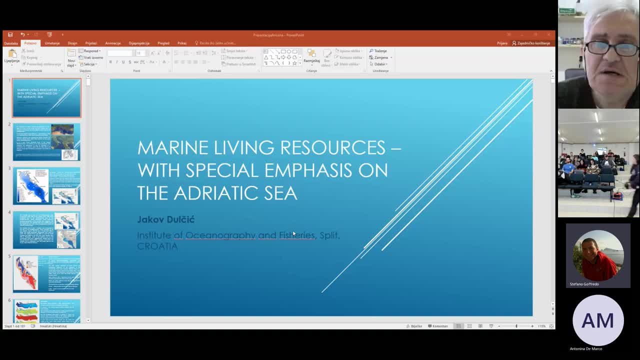 that today is huge. changes are happening, especially in the Mediterranean- Yes, Yes, Yes, Yes, In the eastern part of the Mediterranean Sea, And these changes makes some huge problems, especially if some of new invaders, a non-indigenous species, became invasive. 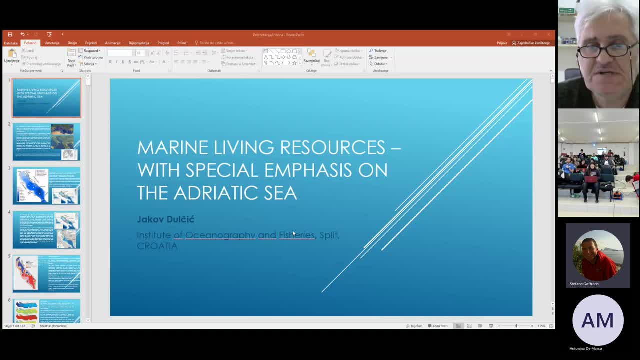 There are many cases of such changes, especially of some kind of species, And And I will try to show you very shortly about these changes, since I worked on the changes and entrance of new species, which mostly are coming from the Suez Channel. 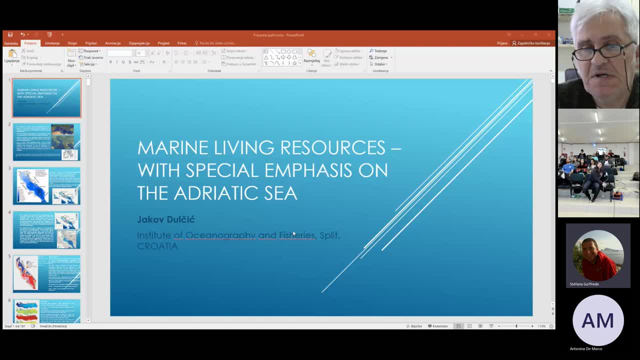 And such species became today members. such species became members of the Mediterranean ichthyofauna and they made some huge changes in food web. Okay, that's about my today occupations and what I'm going, what I'm trying to research. 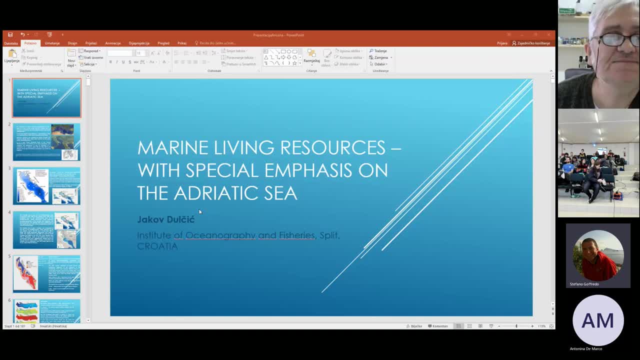 And now I will go back to the problem of which I'm teaching, trying to present you Okay. Okay, Since when I started, when I was younger and I was a professor on the University of Split, I had the Collegium Marine Biology Resources and I tried to present to my students much. 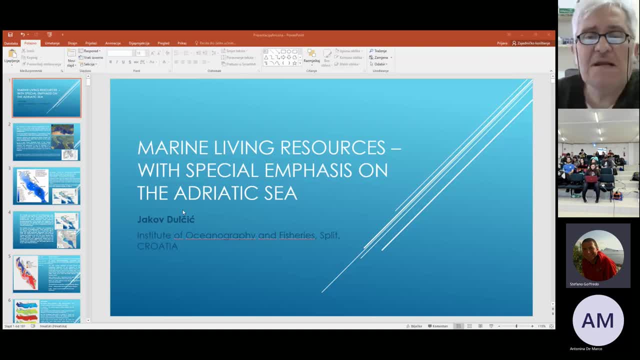 more information about the whole, about all the marine living resources. Now I will try to say about a few words about this, just for the Adriatic Sea. So most of my presentation is the is presented also in one monograph. The name of that monograph is recent state, especially for the Adriatic Sea. 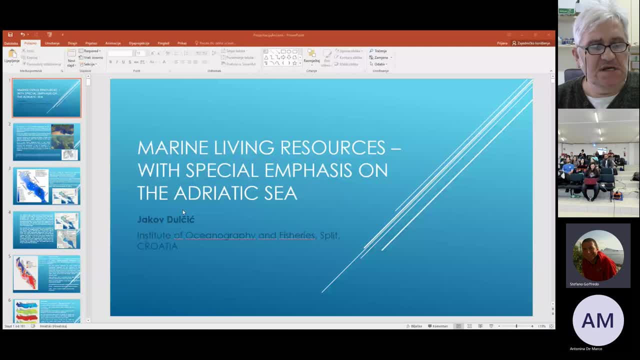 for the Mercer Resources- Recent State of the Mercer Resources in the Adriatic Sea And that monograph was published in Acta Adriatica Journal of the Institute of Oceanography and Fisheries, And authors of this monograph was Corrado Piccinetti. 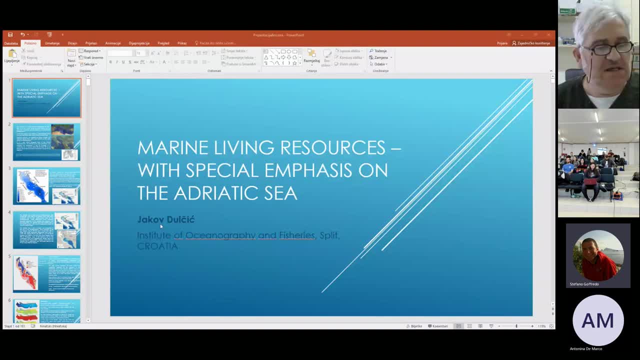 famous professor from Italy, Then Nedo Virgoc from the SPRIT Institute, Bojan Marčeta from Slovenia and Ms Chiara Manfredi. They prepared very nice monograph And practically I think that 60 or 70%. 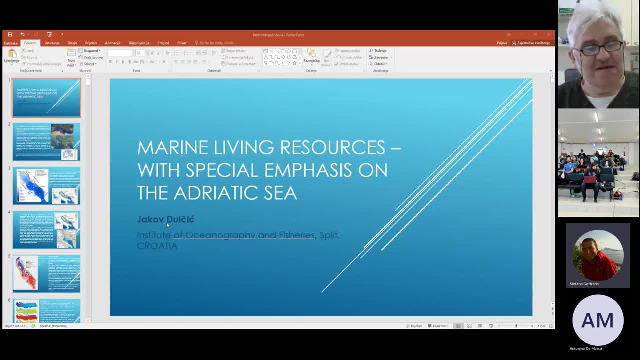 of this presentation is connected mostly with that monograph, Recent State of the Mercer Resources, And I will try to. I will try to say just much more words about the Pelagic resources which were prepared by most of the authors from both sides. 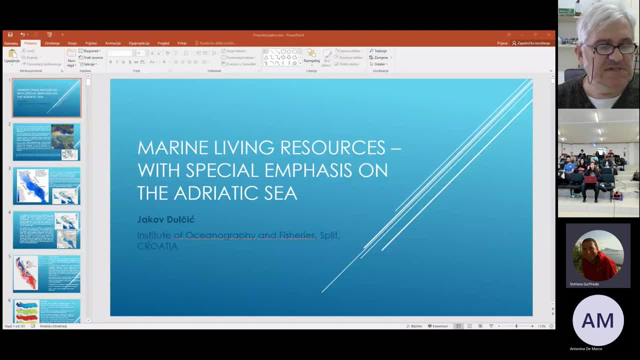 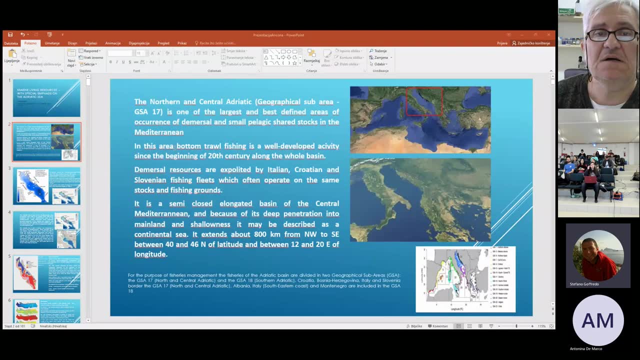 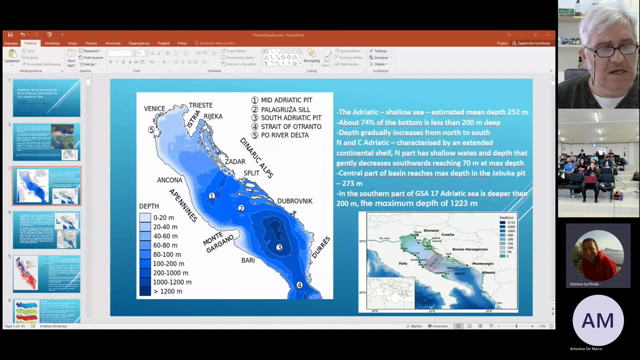 even though including experts from Slovenia. Okay, If we try to say generally about the Adriatic Sea, we could say that in general, Adriatic is a shallow sea. It's a semi-closed, elongated basin of the central Mediterranean And, because of its deep penetration into mainland, 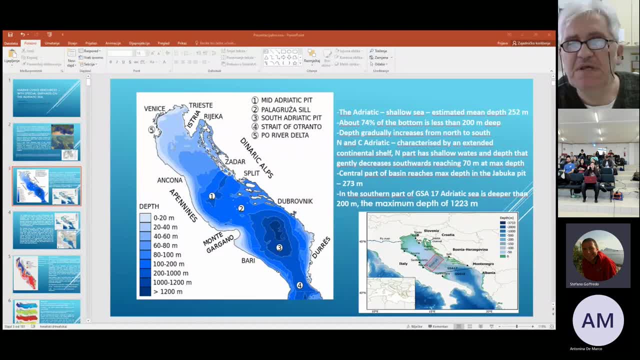 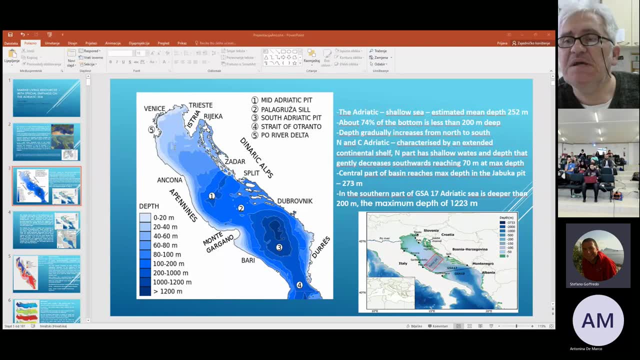 and the shallowness. practically it could be described as a continental sea. Estimated mean depth is about 252 meters. About 70% of the bottom is less than 200 meter deep And the depth gradually increases from north to south. 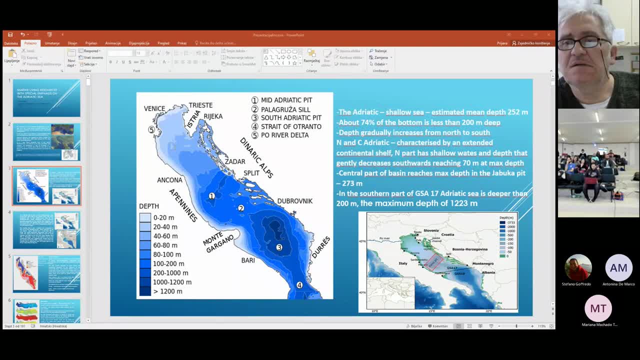 And it extends about 800 kilometers from northwest to the southeast, And its wide range is from, let's say, 90 to 220 kilometer. It is connected to the rest of the Mediterranean by the channel of Otranto, Let's say about. 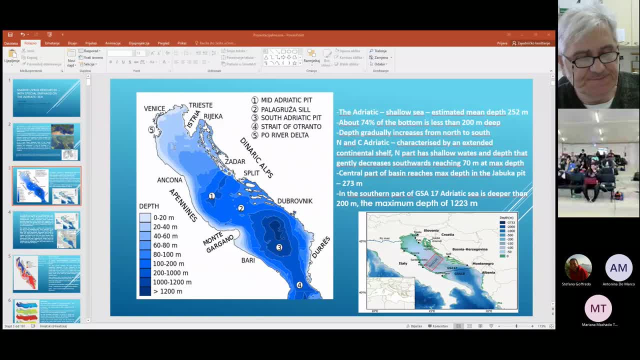 About 40 nautical miles wide and 780 meters deep, which plays a very important role in the circulation and exchange of water masses between the Adriatic and the Ionian Sea On this place. at this time, I just I would like to mention that there are some theories. 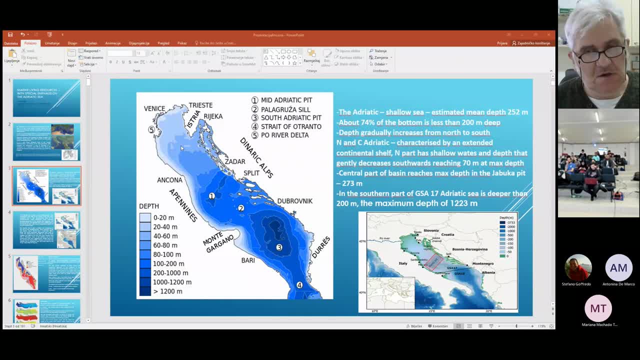 between old theory about the ingressions of waters from the Ionian Sea into the Adriatic And such water is, as I learned about it was much more warmer, Warmer part of the Mediterranean than Adriatic. So the input of warmer water and et cetera. 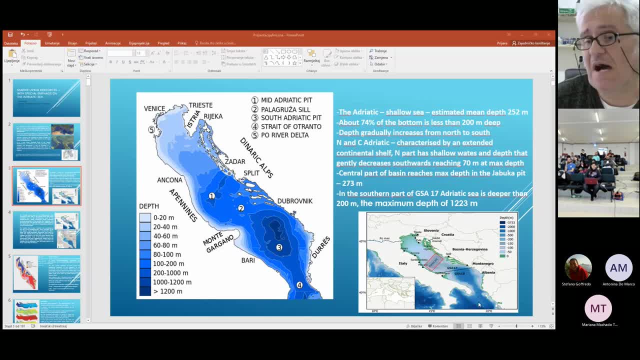 increase the primary production And after that of course secondary. And nowadays there is some kind of new, let's say, reconstruction of that theory. It is about the theory about the bimodal oscillation. It is also in general some parts of the old theory. 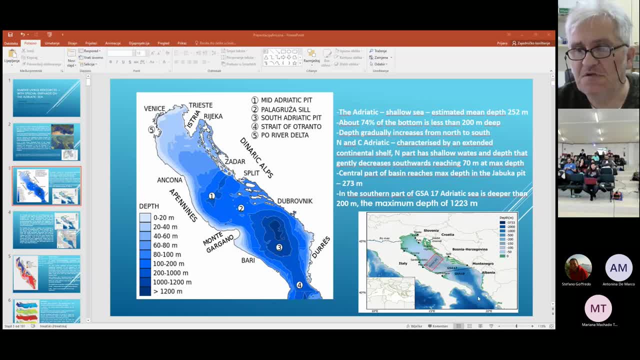 about the ingressions from the Ionian to the Adriatic Sea. It has some kinds, let's say small modifications And there are now theories of bios, bimodal oscillations, bimodal oscillation system, which is in general same as, like it was, the theory of ingressions of waters. 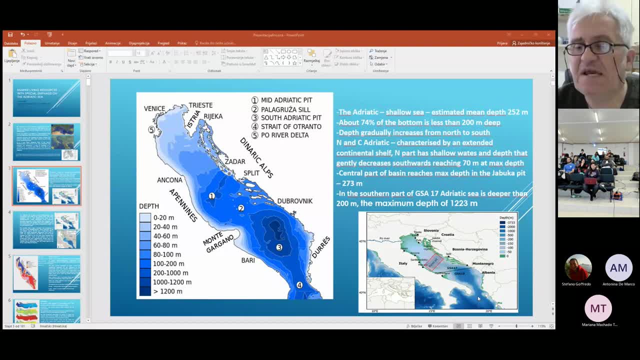 Why am I speaking about this? Because it is nowadays very important to know the circulation and impact of Ionian Sea to the Adriatic Sea And, in very simplified to say, there are now two types of gyres in the Ionian Sea: when it is connected with the eastern part. 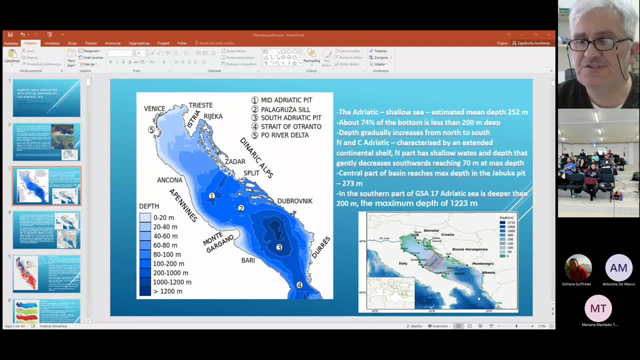 of the Mediterranean And during such gyres which are in the Ionian Sea. there are some parts of the year when this type of waters which are entering there are some part of the effect of the levantine And in some time it is connected with the impact. 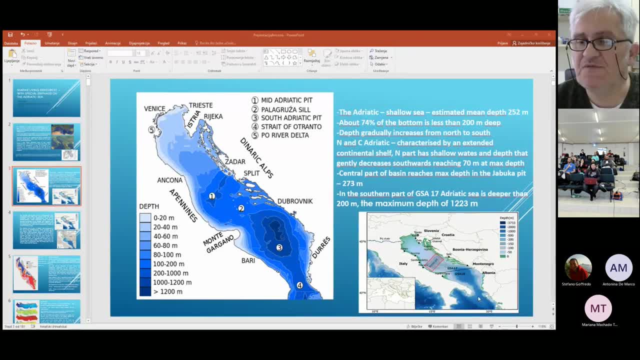 of the waters which are coming from the Atlantic Ocean, or let's say much better, to the western part of the Mediterranean. So such two types of waters are entering in the Adriatic Sea, changing the hydrographic moment And, according to that, biota moments of the Adriatic Sea. 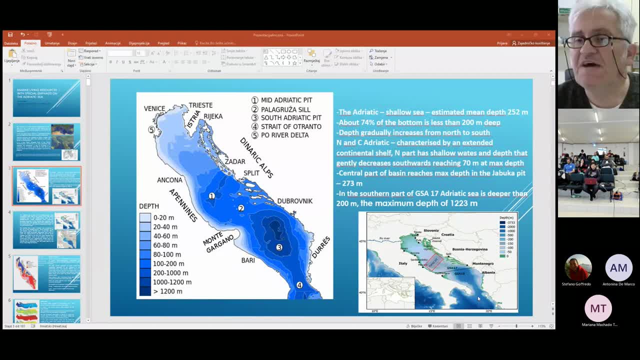 And during the entrance of the levantine water. it is possible that in some part of the period that some organisms which are coming from the Suez Channel are also entering during that time into the Adriatic Sea And when this type of waters are stopped. 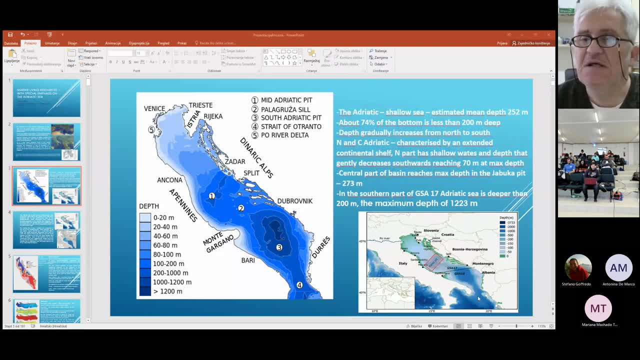 and when started another part. it is part when the waters from the waters from the western side of the Mediterranean, let's say Atlantic waters, there are impacts of the organisms which are entering through the Gibraltar area or from the or from the Mediterranean part. 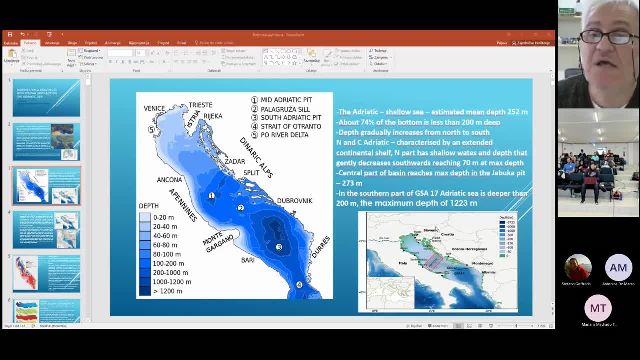 western Mediterranean part of the sea. So what to say again? Central part of basin reaches maximum depth in the Yabuka or let's say Pomo pit. It is the deepest part- I'm mentioning this very important part- of the of the Adriatic. 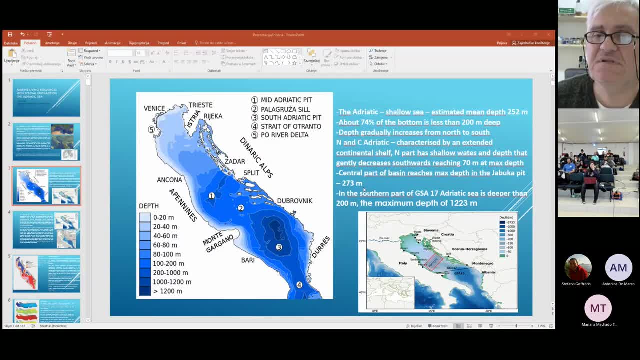 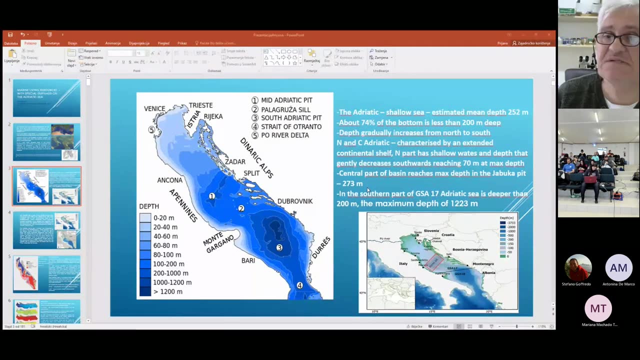 It is Yabuka or Pomo pit, And with the depth of 273 meters, because you will see in the next presentation parts of that very important place which are mostly spawning area of very important demersal resources and very important demersal species. 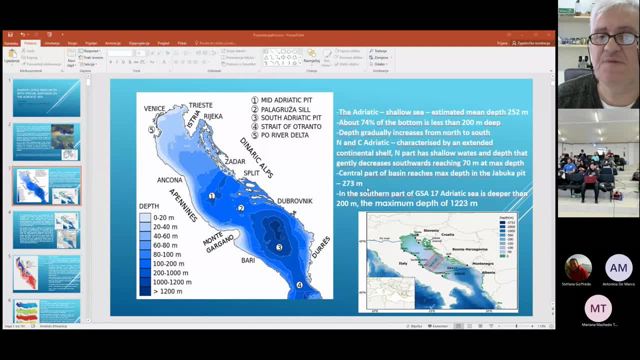 which are the part of the main parts of the catches which are which are happening, especially the demersal demersal of trawl, demersal resources by trawls In the southern part, this, let's say, sub-regional area 17,. 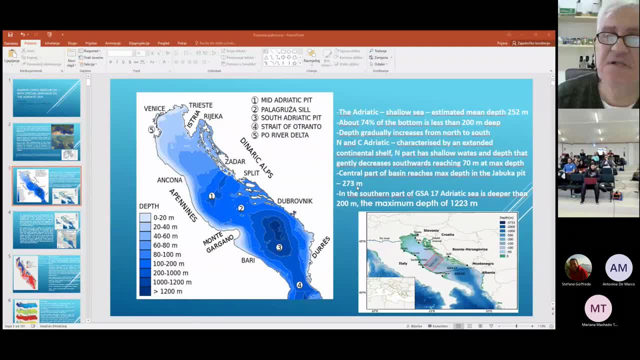 GCA 17,. Adriatic Sea is deeper than 200 meters and the maximum depth is about about 1,223 meters. This is, I think, the deepest, the deepest point of the of the Adriatic Sea. You will see here on this picture that 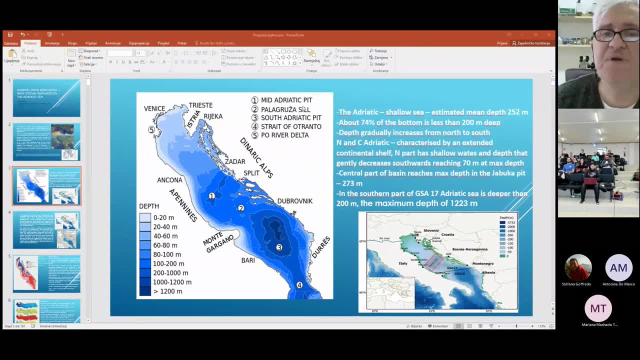 that what I already said: mid Adriatic pit, or let's say Pomo pit, Yabuka pit, Then it is Pala Gruža sil, South Adriatic pit, straight of Otranto, And very important, very important for the northern part. 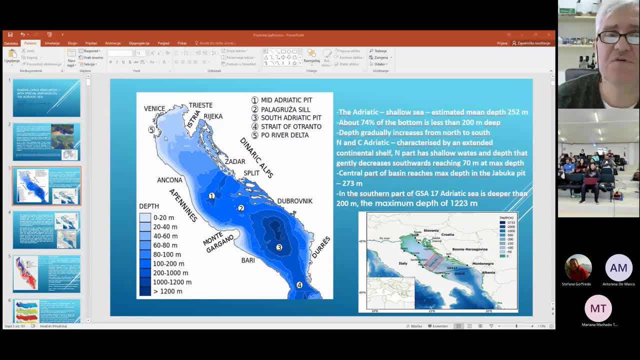 not just for the northern part, but for the whole Adriatic Sea. Just to be back, I forgot to say that northern and central Adriatic geographical subarea, GCA 17, is, is, is, is, is, is. 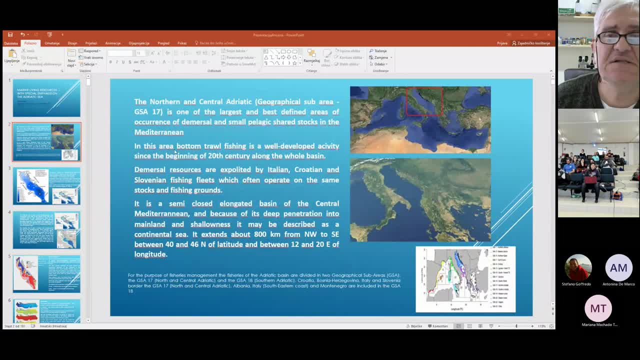 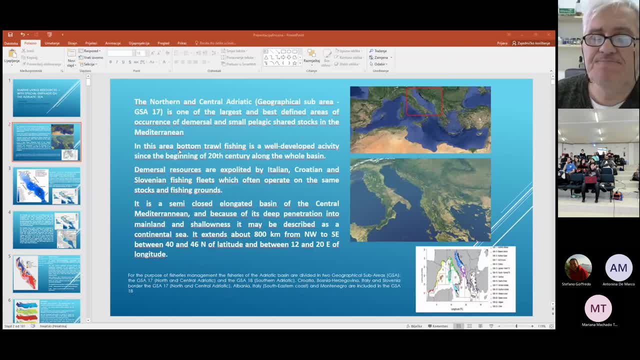 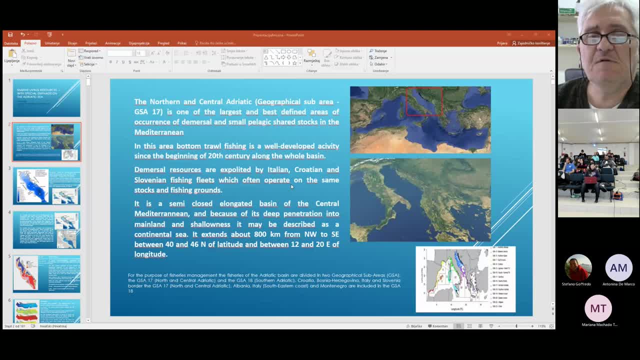 It is what I already say. if you see, for the purpose of fisheries management, the fisheries of the Adriatic is divided into two geographical subareas: 17,, which include north and central Adriatic, and GSE A 18, the southern part of the Adriatic and the countries which are included in GSE 18 is Montenegro and Croatia. Bosnia, Herzegovina, Italy and Slovenia bordered practically the area, subarea 17.. 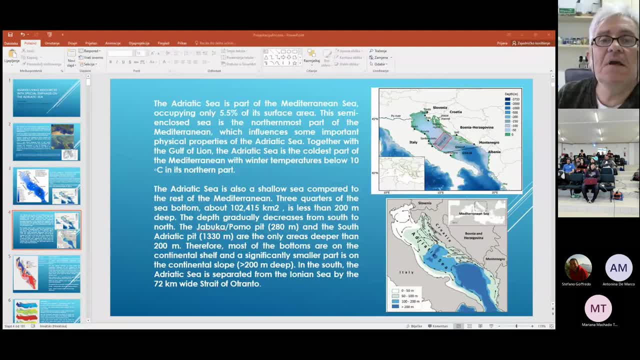 Okay, So we are in. the Adriatic Sea, together with the Gulf of Lime, is the coldest part of the Mediterranean wind, with the winter temperatures below 10 degrees of Celsius in its northern part. This is very important to know because if you already know that the northern part of the Adriatic Sea is very cold, 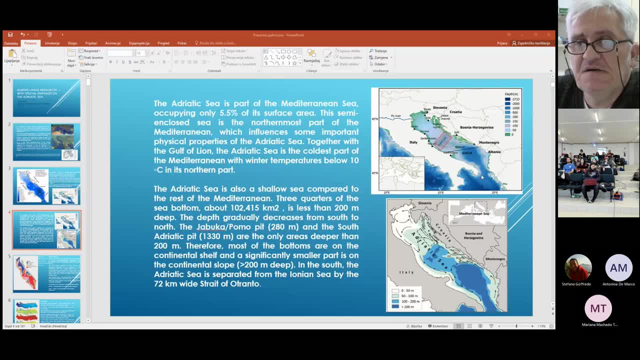 Okay, Okay, Okay, Okay, Okay, Okay Okay. part of the diatic is very, very interesting. It means that one great man from from split, professor from the other part of them, was other speedy on Bruce in made it in 19th century a. 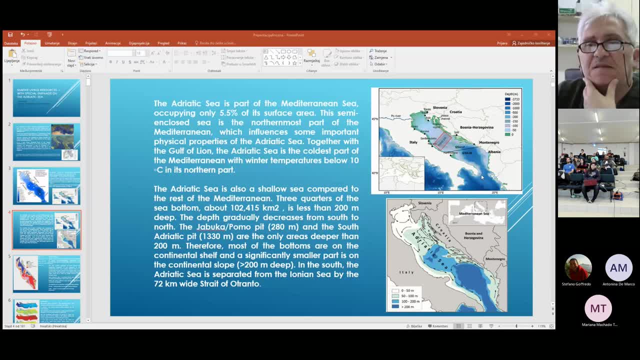 theory of boreal. boreal theory that in the Adriatic Sea, the only part of the Mediterranean, exists a boreal fauna, So practically it. his theory, was very important because we know now that such kind of species, fishes and other organisms are. 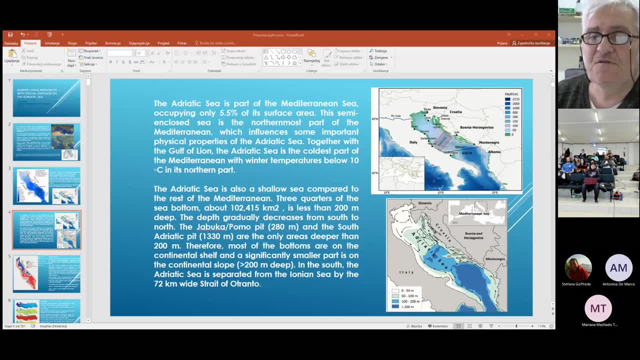 existing as boreal fauna in the northern part of the of the Arctic Adriatic. This this will be seen. This is very important because if you see in the marzell catches there are differences in catches in the marzell in trouser for example. 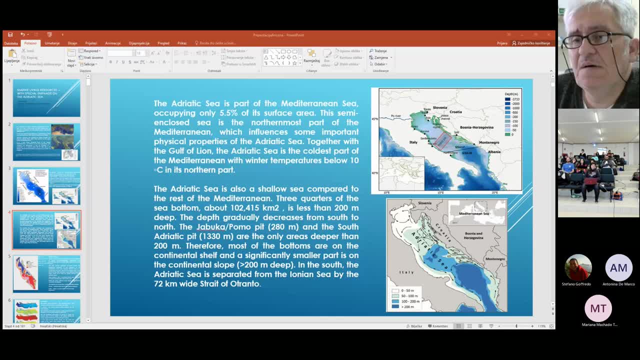 between the northern and the southern part, center and southern part, because complete fauna is according to to to to that theory is practically made it completely different. For example, main, main catch in the marzell, in trolls, in central and the southern part is cake for. 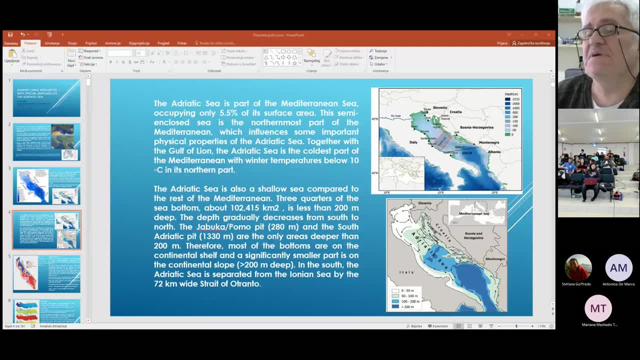 example, and in the northern part, for example, is the software- was me notice my language and I guess a typical types of organisms which are connected with the with the colder, colder, what a colder temperature. And the Atlantic Sea is also a shallow sea compared to the. if 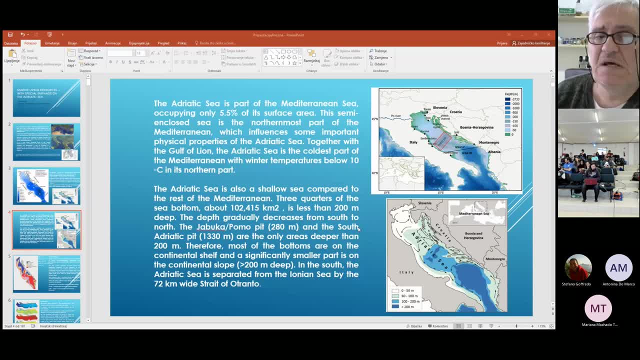 compared to the other parts of the Mediterranean. three quarters of the sea bottom is less than 200 meter depth. the depth- what I already said- gradually decreases from south to the north. in the Yabuka Pomo pit, 280 meter 205.. And the South Adriatic pit is the only. 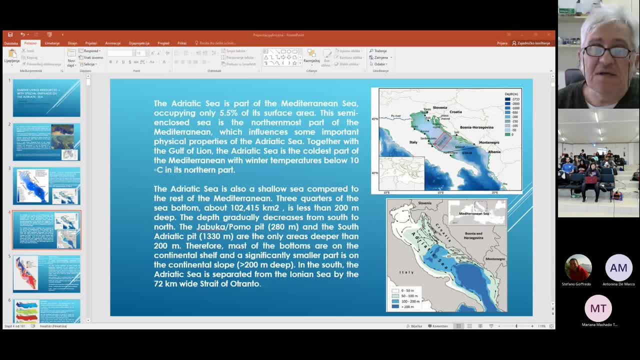 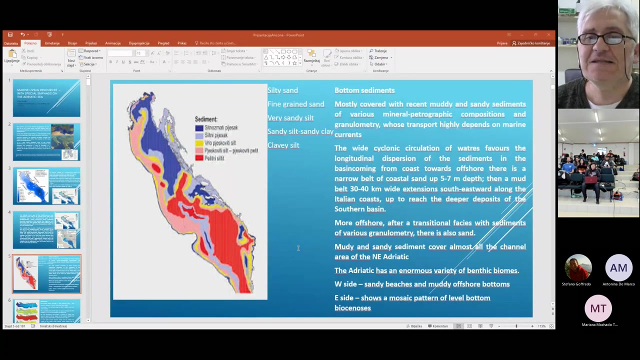 areas deeper than 200 meter. there, Therefore, most of the bottoms are on the, let's say, the part which we call continental shelf, and significantly smaller Part is on the continental slope, which are less than 200 meter deep. He, I think that is all for this. let's say some characteristics. 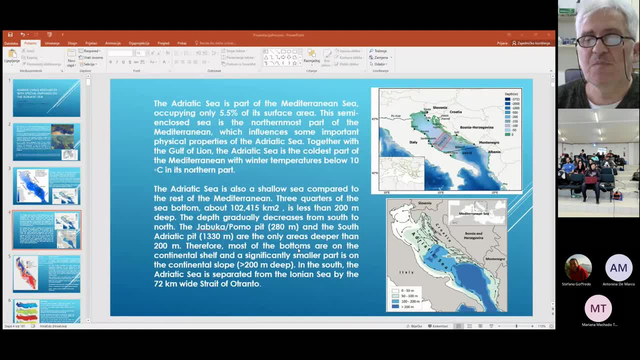 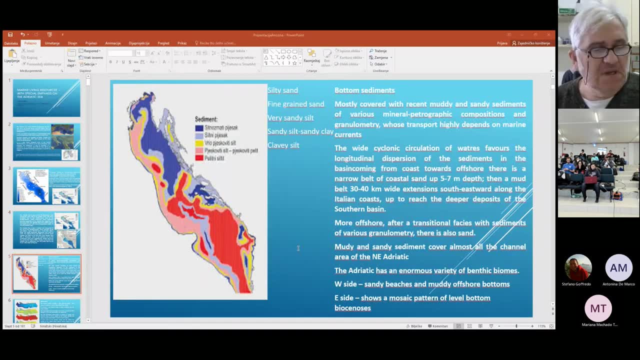 about the, let's say, most important parts of the characteristics of the Adriatic. just few words about the bottom sediments, which are mostly covered with the recent muddy and sandy sediments of different mineral petrographic compositions, and the gondolometry. 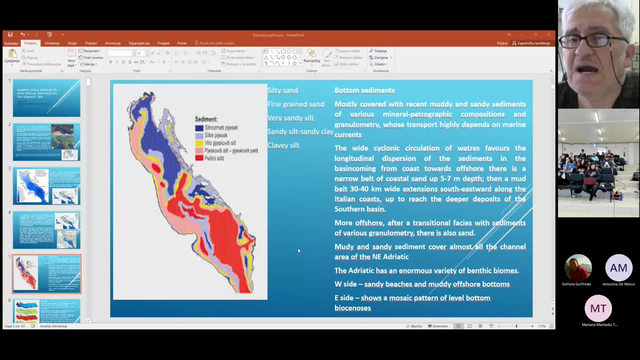 which transport highly depends on marine currents. The wide cyclonic circulation of waters favourise the longitudinal dispersion of the sediments. in basing, coming from coast towards offshore, there is, let's say, a narrow belt of coastal sand up to five or seven meter a meter depth, then a mud belt 30 to 40 kilometers wide extensions. 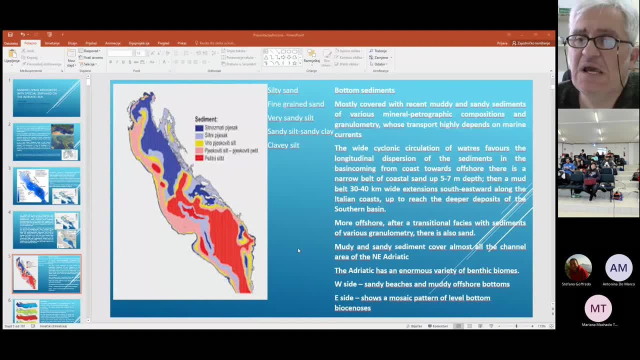 southeastward along the italian coast and up to reach the deeper deposits of the southern basin, most more offshore after transitional phases, with sediments of various granulometry. there is also sand, muddy and sandy sediment cover almost all the channel area of the northeast adriatic and the adriatic has enormous variety of benthic biomes. 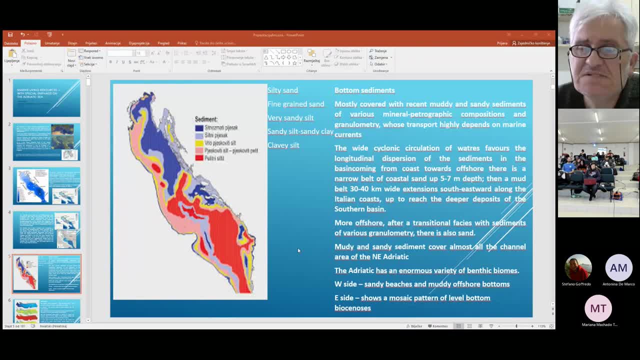 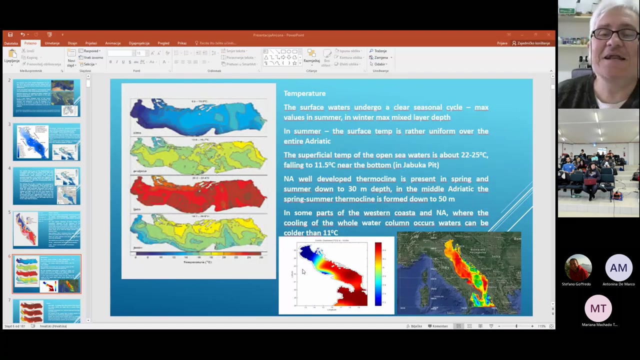 uh, let's say that western side is mostly covered by sandy beaches and muddy offshore bottoms and eastern side shows, uh, let's say, more different types of level bottom biosynosis. okay, i know this is very boring, but i need to to mention because it is connected with 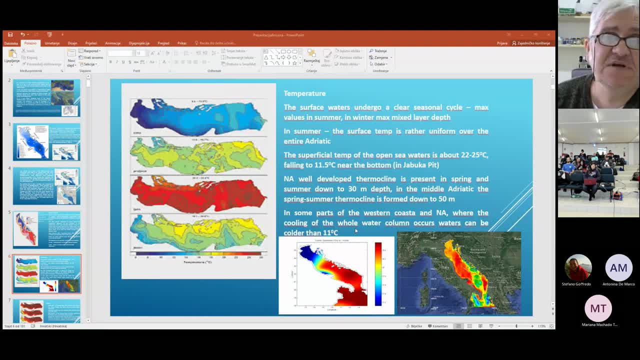 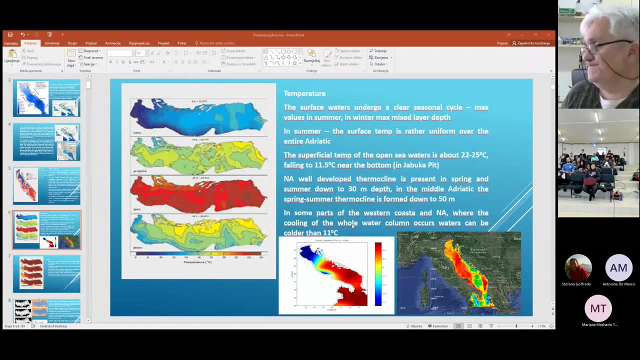 the living resources, because it is very important to know which kind of species are connected which with which kind of sea bottom. okay, now we came to. very important factor is temperature, because the temperature regulate practically almost biological cycloses, life cycloses of, let's say, most, most, except the mammals, of marine organisms. 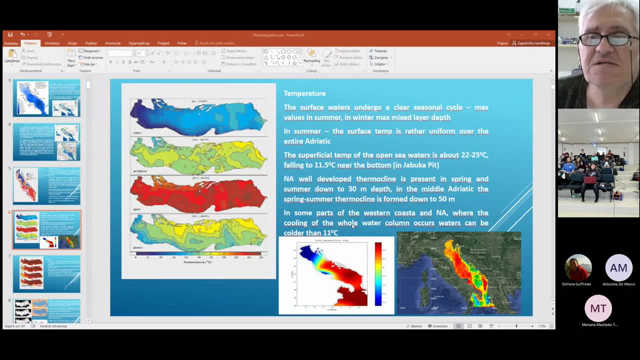 the surface waters and there got clear seasonal cycle cycle because maximum values are in summer in in winter, maximum mixed layer depth in summer. the surface temperature is rather uniform over the complete over the complete adriatic. the superficial temperature of the open sea waters is about 22 to 25 degrees celsius falling. 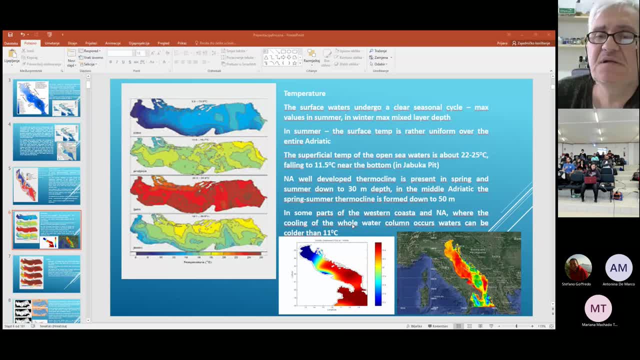 to 11.5 degrees near the bottom, let's say in the yabuka, in the yabuka pit or pomapit north at north adriatic. uh, it is in. it is in that part, a well-developed thermocline and it is present in the spring and summer down to, let's say, about 30 metro depth in. 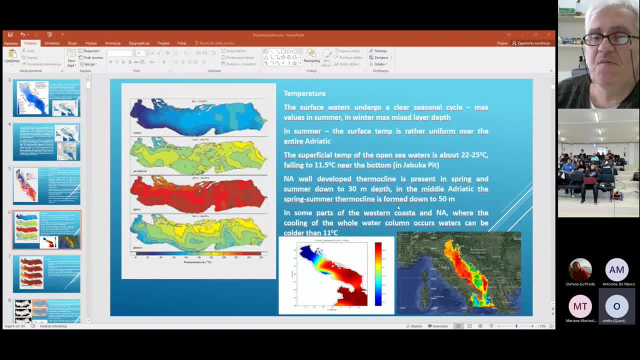 the middle adriatic, the spring summer thermocline is, let's say, formed down to 50- 50 meters depth in some parts of the western coast and in the northern adriatic, where the cooling of the whole water column occurs, waters can be colder than 11. what i already uh said in in one part of. 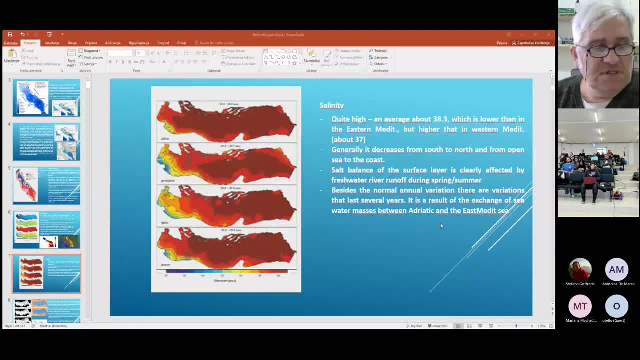 my presentation. let's say a few words about the salinity uh in general. uh, if we, if we uh see, uh the adriatic salinity, it is, in general, quite like we could say quite high and average about uh 38.3, which is lower than in the eastern mediterranean, but uh of 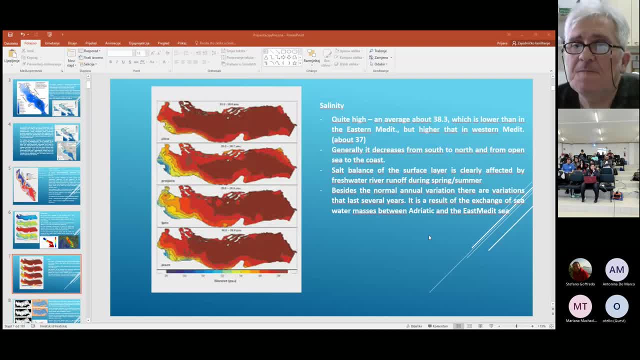 course higher than in the western part of the mediterranean. where is about, let's say, 37.. uh, generally, we could say, uh, it decreases from south to north and uh, from open sea to the coast. uh, south balance, or let's say, balance of salinity. uh, the servers layer is clearly affected by. 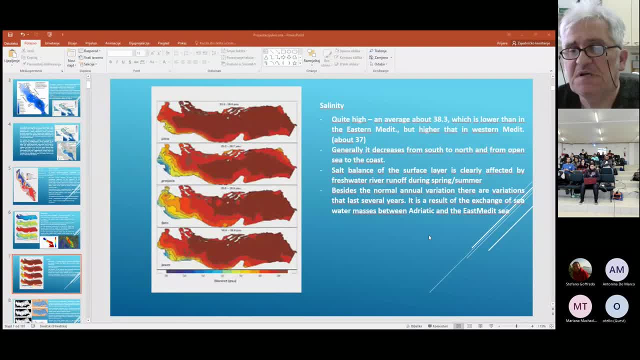 freshwater river runoff during the spring summer. of course, of course there is. there is the huge rivers from both sides, especially, let's say, river po, and from the southern part, from the eastern part, uh, uh. that is the river narrative, and the effect is, of course, much more. 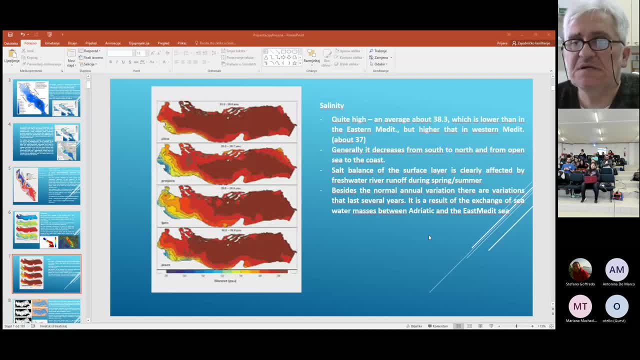 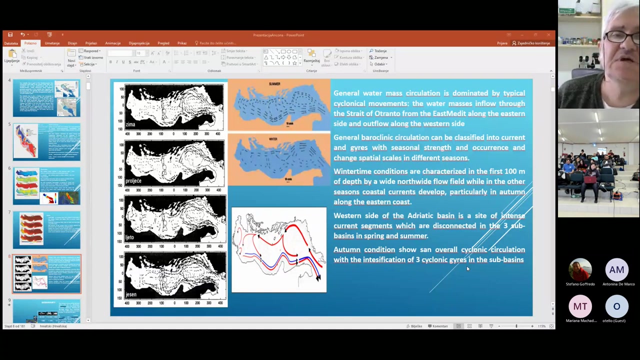 exposed about in the in the surface area, and there is a huge impact of freshwater river runoff. besides the normal annual variation, there are variations that last uh, uh, uh, uh uh several years, and it is this is a result of the exchange of seawater masses between uh the attic and uh eastern mediterranean sea. uh, i think that uh very important. what? 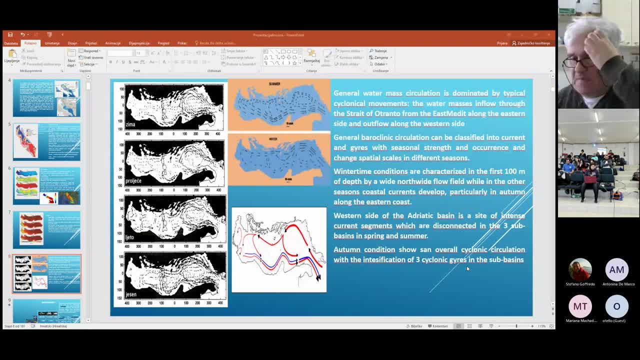 i already said about my uh, about the mentions about the uh ingressions and and and and now bios bimodal oscillation system- general water masses circulation in the Adriatic Sea is dominated by typical cyclonical movements. The water masses inflow through the Strait of Otranto from the eastern Mediterranean. along the eastern side and outflow along the western side. The general barocline circulation can be classified into current and gyres, with seasonal strength and occurrence and change spatial scales in different seasons. The wintertime conditions characterized in the first period by an open sea with a depth of 100 meters, by a wide northward flow field associated. 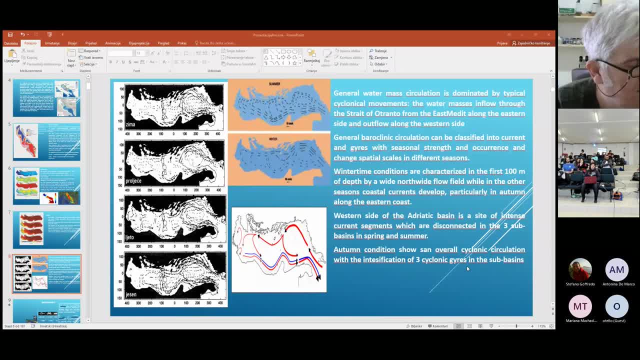 with intense but shallow returns. yet jets along the western coastline, while in the other seasons coastal currents develop, particularly in the autumn, along the eastern coast. The western side of the Adriatic Sea is known as the Adriatic Sea basic, is a site of intense current segments which are disconnected in three. 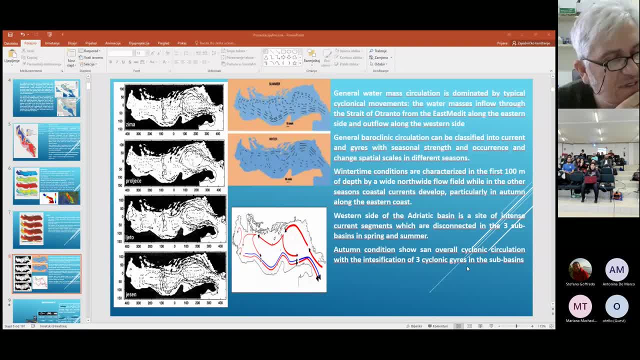 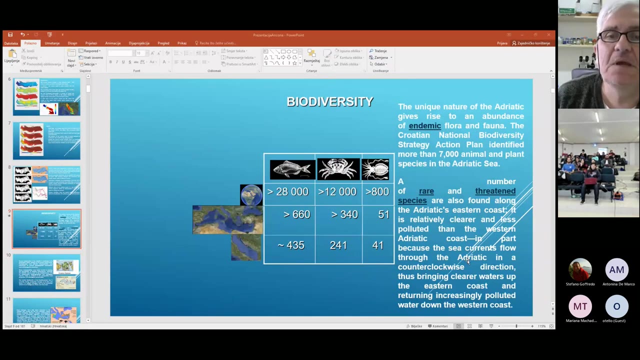 in three sub bases in spring and summer. the autumn condition shows an oral overall cyclonic circulation with the intensification of face iconic gyres in the sub base. sorry, now we should say about few words about the sorry biodiversity of the Adriatic Sea. you can see here fishes, crustaceans and cephalopods for the whole world you see. 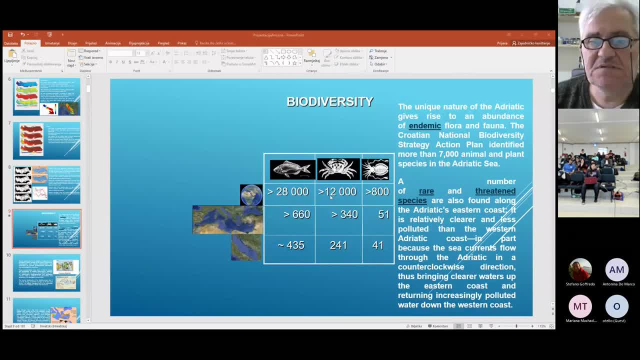 more than 28,000 species, for crustaceans more than 12,000, and from for for mollusks more than 80 800. I think that of course, this changes, or a all the time uh, for the whole mediterranean, it's uh about six 660 species for for fish. 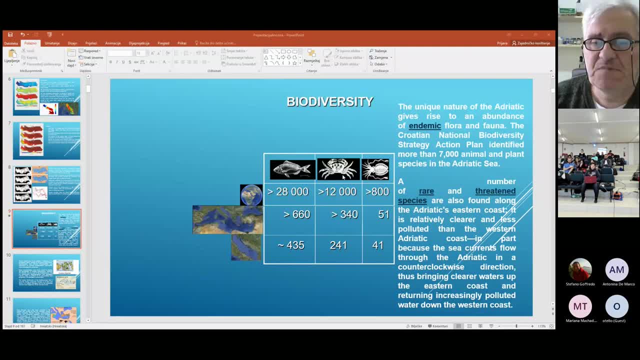 about 340 for the, for the crabs, and 51 for for cephalopods, mollusks and for the adriatic. you can see here this. this number is always exposed to changes, of course, especially nowadays when, when new species enter or some new is described for the first time, but it is around. let's say 440. 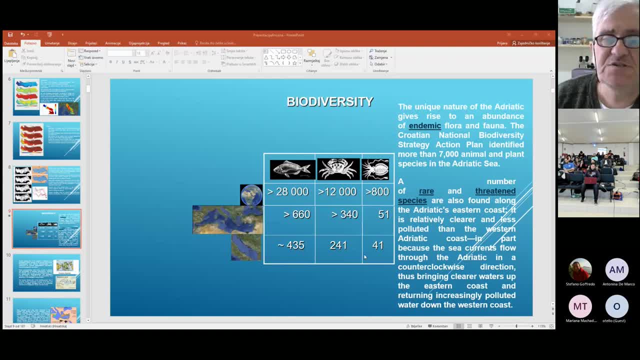 species today about a bit connected with the fish species. the crabs is about 200, 41 and 41 for the cephalopods or mollusks. special, or let's say better to say, the unique nature of the adriatic gives rise to an abundance of endemic flora and fauna. 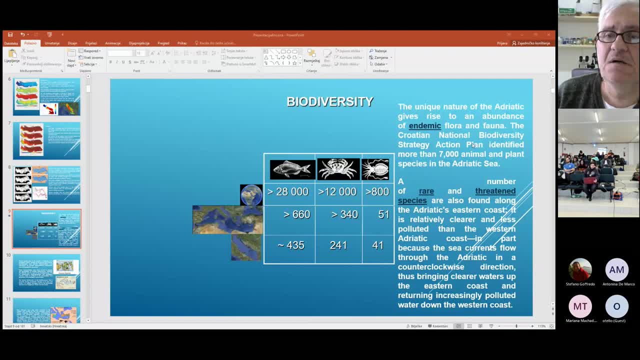 the data from the croatian national biodiversity strategy action plan. they they identified more than, for example, more than 7 000 animal of and plant species in the adriatic sea. also some rare and treatment species found along the adriatic, especially eastern coast. 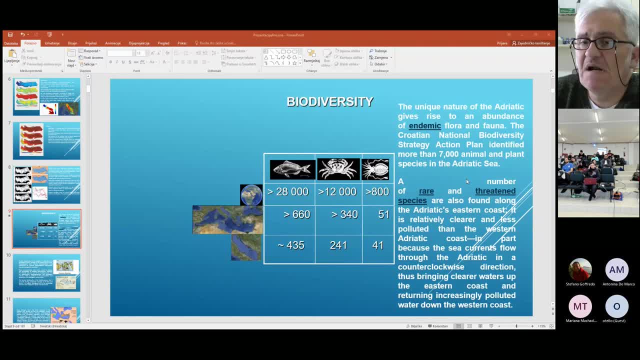 adriatic's eastern coast it is, since it is a relatively clearer and less polluted than the western- uh uh adriatic coast. in part, in part because what i already said, that because the sea currents flew flow through the adriatic in a counterclockwise direction. 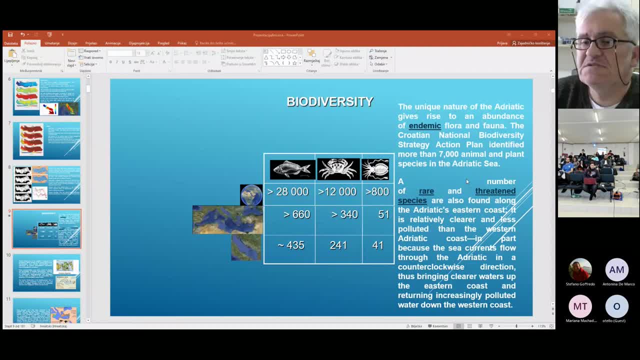 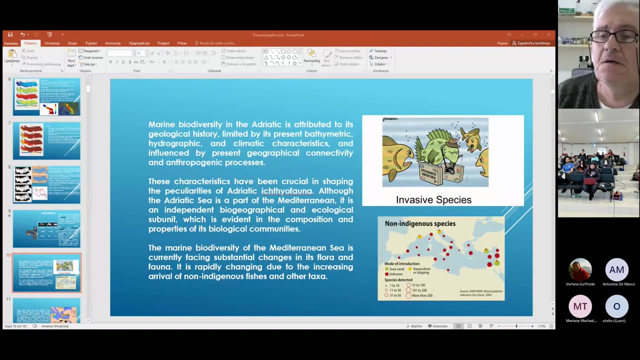 but bringing uh according to that up the eastern coast and returning increasingly polluted water down the western coast. In general, marine biodiversity in the Adriatic is attributed to its geological history, limited by its present bathymetric, hydrographic and climatic characteristics. 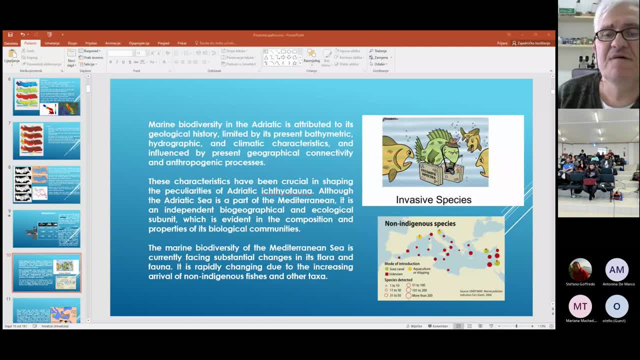 and influenced by present geographical connectivity and anthropogenic processes. These characteristics have been crucial in, for example, in shaping the peculiarities of the specialities, so let's say, of Adriatic ichthyophytes, although it is a part of the Mediterranean. 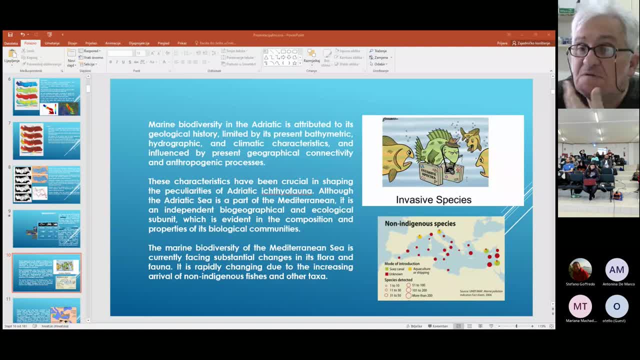 the Adriatic Sea is an independent- we could say is an independent- biogeographical and ecological subunit of the Mediterranean, which is evident in the composition and properties of its biological communities. In general, we could say that the Mediterranean Sea is a hotspot in everything. 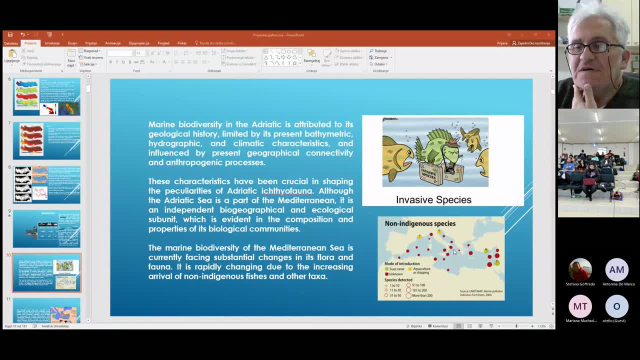 let's say the impact of fishing gears, the impact of tourism, especially during the summer time, the impacts of huge rivers, especially Po, for example, and Nile in Egypt, etc. So, practically in general, the marine biodiversity of the complete Mediterranean Sea. 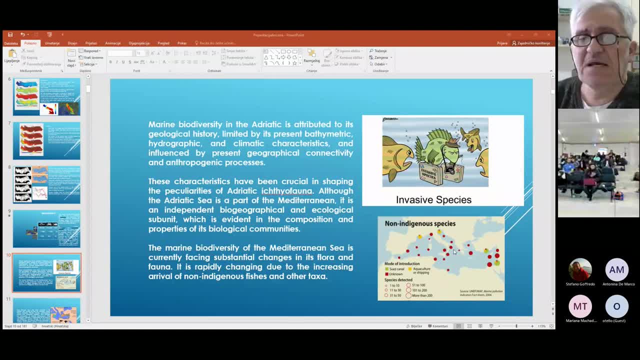 and including, of course, of the Adriatic, is currently facing to substation changes in its flora and fauna, And it is rapidly changing due to the increasing arrival of non-indigenous fishes and other taxa, and especially if such species became invasive And most of 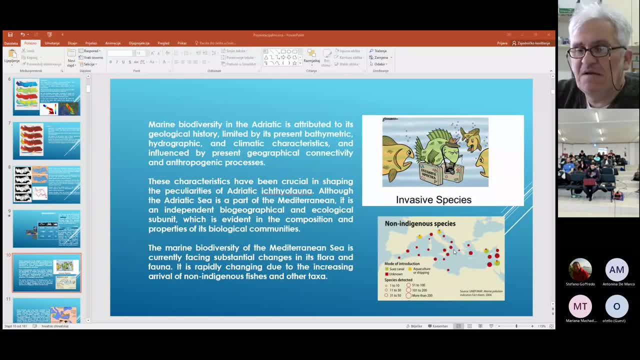 especially fishes which came to the Mediterranean area, became invasive. because this is the what we say, the problem with the changing in food web, because when some kind of species which had some special type of adaptation and biology, for example high, 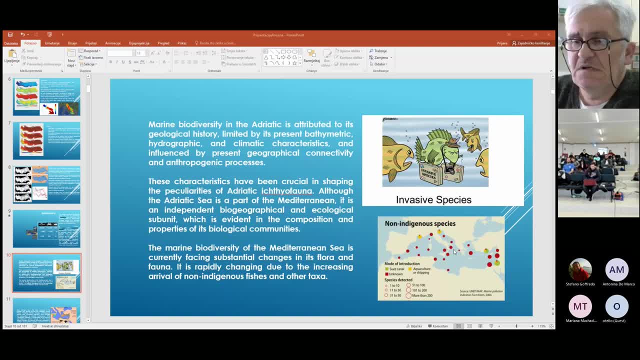 very high fecundity. it is poison it completely. it is, for example, poison fish or whatever. And such type of characteristics support, for example, species which became, in the areas of the Mediterranean, invasive. It means it could be dangerous for consumption. 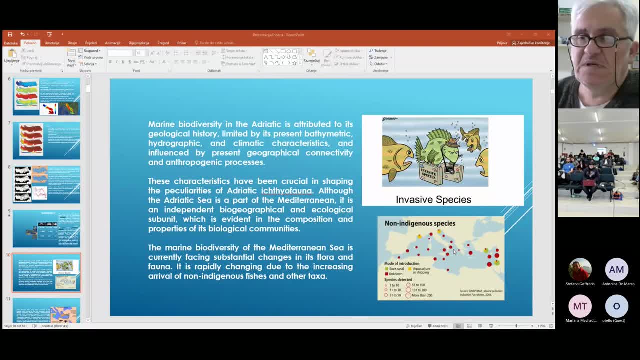 it could be dangerous in fishing industry. it means especially in where is the when a fisherman is taking net from the sea. it can be touched, or it could be touched some kind of species which has a problem with the poisoning in the skin. 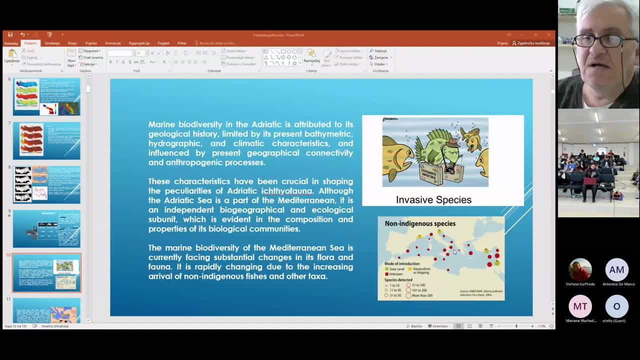 or whatever. For example, Lagocephalus, some kind of species which is poison, is full of poison and even though if you touch the skin you can be dangerous to die. So such changes are very rapid and some of the species entered into the 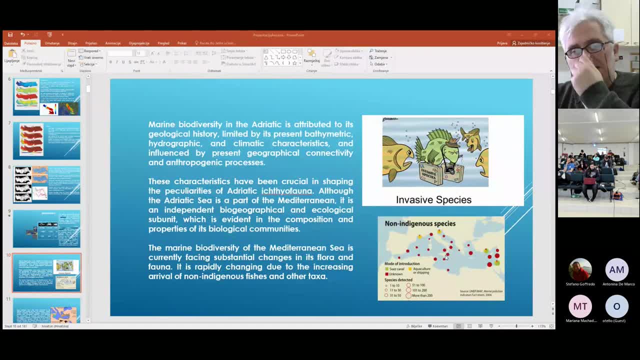 also into the Adriatic and we always said some, some notes to the, to the community to be in danger, to be in preparation for such possibility, and we will try to get much more info and about the species and we'll try to investigate. 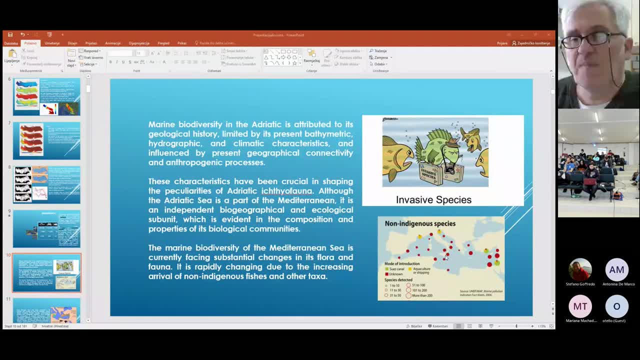 if we will be in possibility to investigate the biology of such invasive species which uh in new area, especially in the new, new new habitats, And we'll see what will be on and I'll try to show you some in the next presentation. 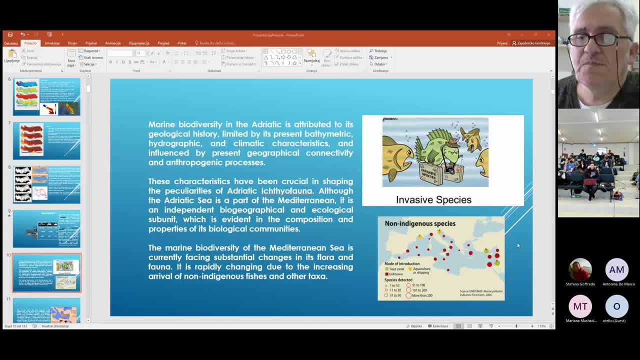 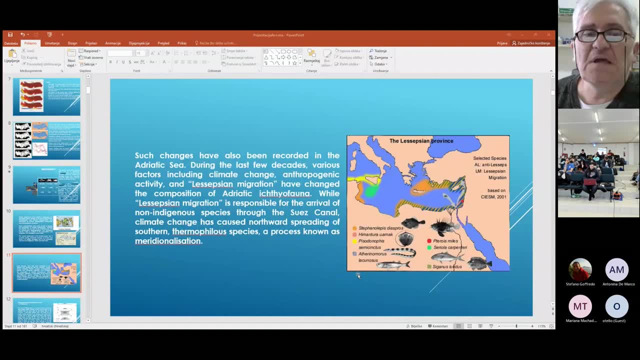 if we will have enough time to to present it some kind of such fish species. Let's say that. But during the last few decades some different factors, including climate change, anthropogenic activity and the Celsium migration, have changed the composition, not just Adriatic. 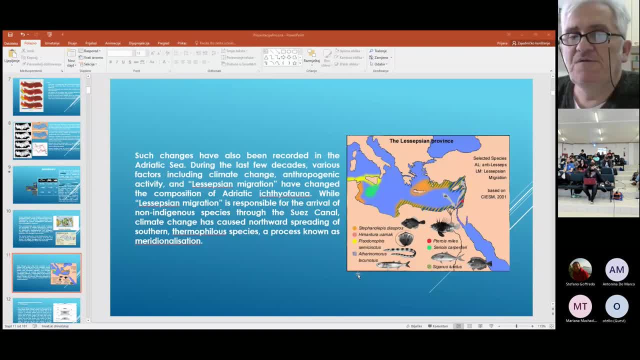 ichthyo fauna, but complete fauna of the especially eastern part of the Mediterranean, but also of complete fauna of the Adriatic. While this here you can see Licepsian migration, for example, it is responsible for the arrival of non-indigenous species through the Suez Channel. 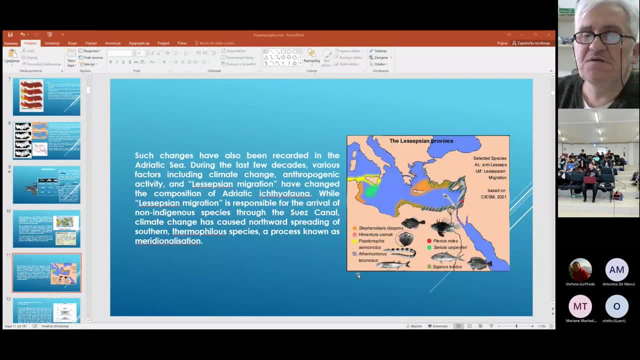 And climate change, for example, has caused northward spreading of southern thermophilus species, a process known as meridionalization. Such these two types of processes could affect the fauna also, not just fauna but also flora of species. So this is an example of the areas you see here, the Suez Channel, and there is also 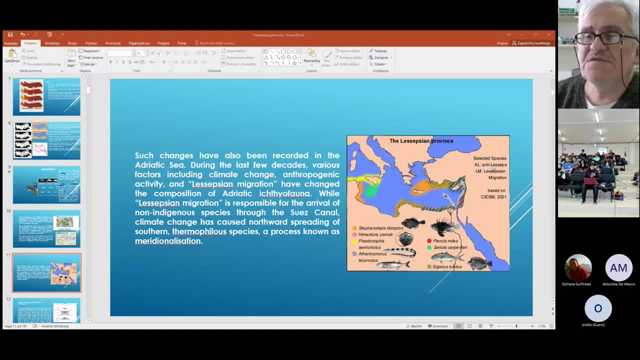 a process of anti-Liceps migration, but it is not so hard. it means that it is not so evident. transport of species from the eastern part of the Mediterranean into the Red Sea. a huge number of species, All the member of the fauna, is going from the Suez Channel to the eastern part. then 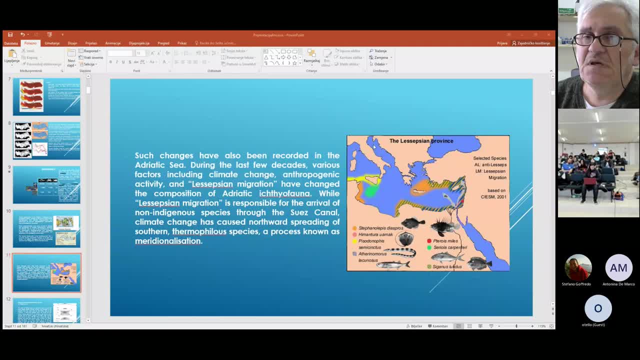 to the Union Sea and then enter to the Adriatic. Here is one kind of barrier between the, let's say, eastern and the western part of the Mediterranean, and most of these invasive species pass this path, Okay, And also enter into the western part, western part of the Mediterranean. 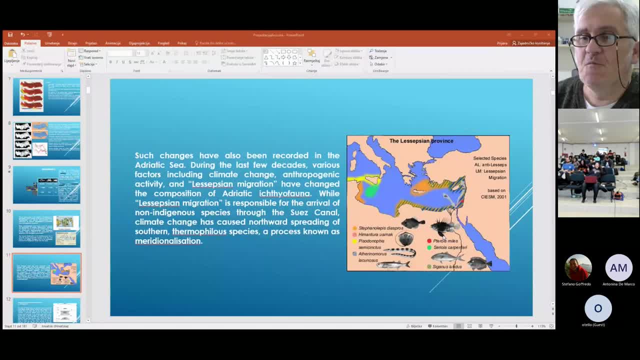 One of the most recent new members of the Adriatic Sea is species which I'm showing now just a moment: Pteris, smilis, any devil, fish or whatever. It is, Wow, Very aggressive kind of species which now occupy all the eastern part of the Mediterranean. 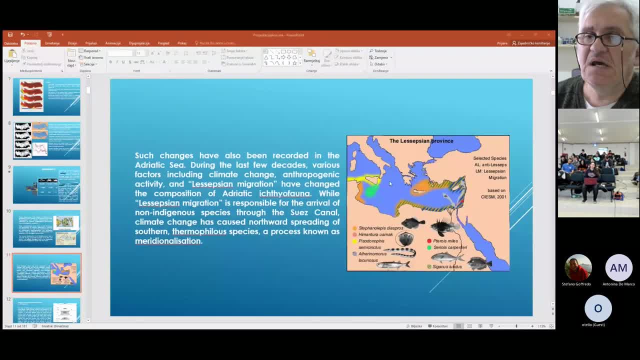 also pass this barrier between the eastern and the western side, And there are now, I think, one, two, three, four, five, five specimens found in the Adriatic. One was found here, Okay Okay. One was found here nearby the island of Vis. 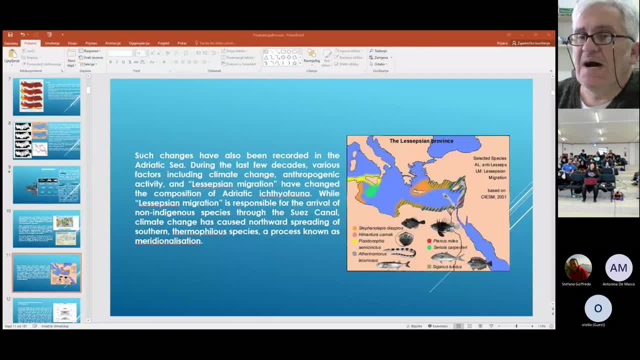 And two were found down there near Bari And one was found also in Albania and one was found in Montenegro coast. So practically if this species enter through the old parts it could make a huge chaos in fauna of the Mediterranean And the Aegean Sea now has a lot of domestic species because it is very aggressive. 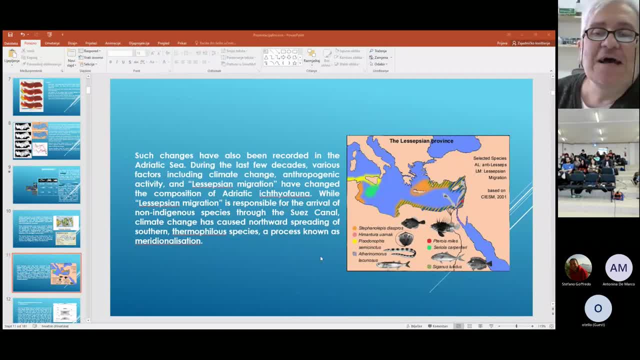 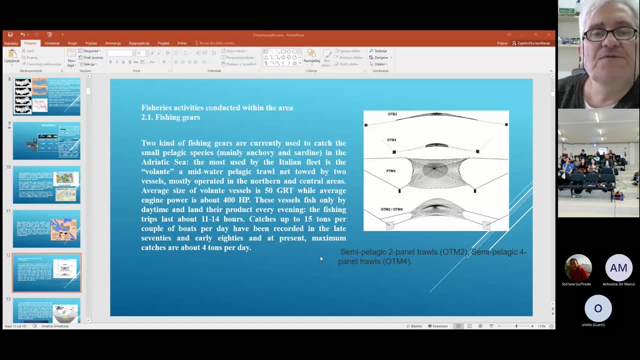 And I will stop now here about that. Okay, we must go on A few words about the fisheries activities which is conducted within the area of the of the Adriatic Sea sea, If we touch the fishing, type of fishing type, gears, for example, two kind of fishing. 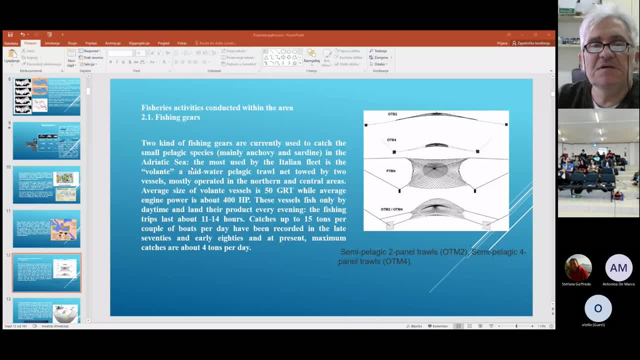 gears are currently used to catch the small pelagic species. It mainly it is anchovy- and in the Adriatic Sea, And the most used by the Italian fleet is the domestic name Volante midwater pelagic trawl net, towed by two vessels mostly operated in the northern and central 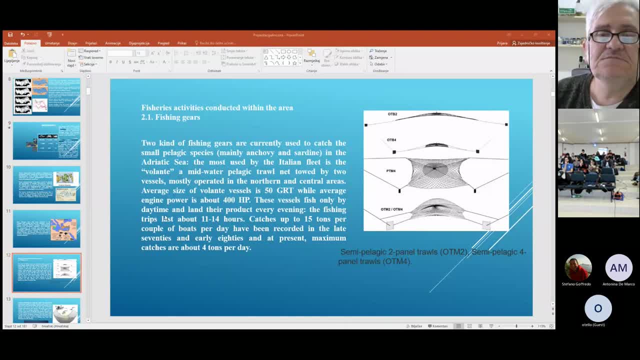 areas of the Adriatic. These vessels fish only by daytime and land their product every evening. The fishing trips last about 11 or 14 hours. Catch is up to, for example, about 15 tons per couple of boats per day. what was recorded? And in the late seventies and early eighties these vessels 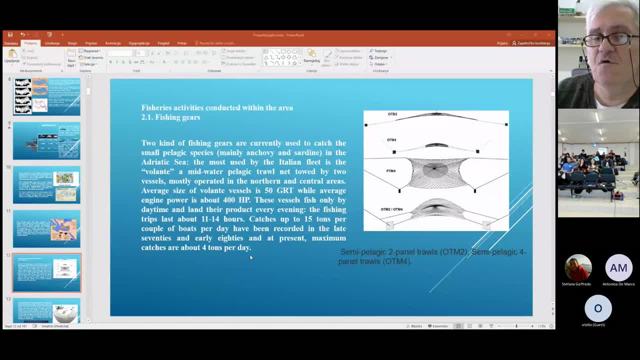 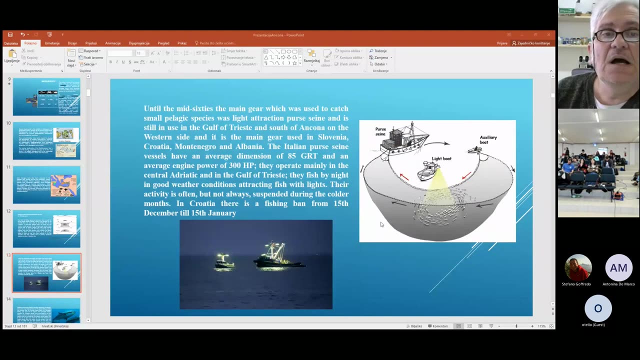 at present maximum catches about four tons per day. You see here the construction of this type of pelagic trawl net. Until the mid sixties, the main gear which was used to catch small pelagic species was a light attraction, Wurzane. 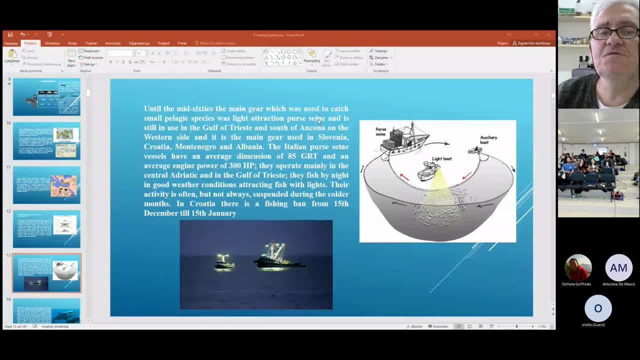 And it is still in use in the Gulf of Trieste and much more south of the Ancona on the western side, and it's the main gear used in Slovenia, Croatia, Montenegro and Albania. The Italian Pursin has an operate mainly in the lower regions. 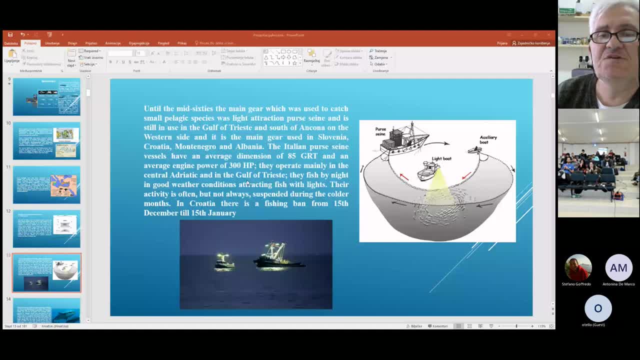 central Adriatic and in the Gulf of Trieste. They fish by night in good weather conditions, attracting fish with lights. Their activity is often, but not always, suspended during the colder months. In Croatia, there is a fishing ban from 15 December till the 15th January. It depends also. when these main species is spawning, and it could be changed this period, But mostly it's from 15 December till the 15th January, And I think that now, according to- I didn't check it, but I'm sure that they made it a new fishing ban for the for the period when. 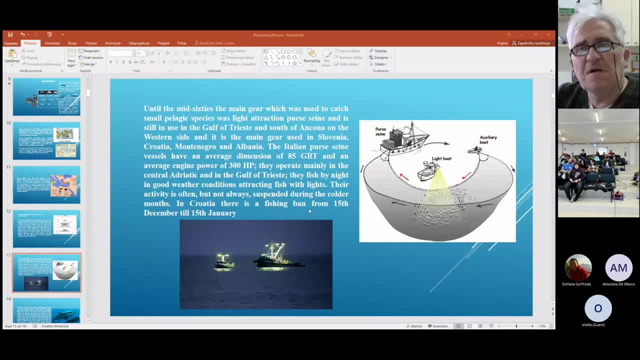 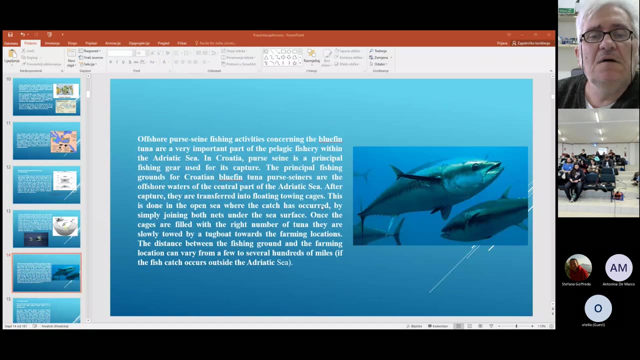 anchovies are spawning. I think that it started in May. I think it started in May. We have a question. We have fishing activities which are concerning the bluefin tuna, which is offshore. poor seine fishing activities is a very important part of the pelagic fishery within the Adriatic Sea. 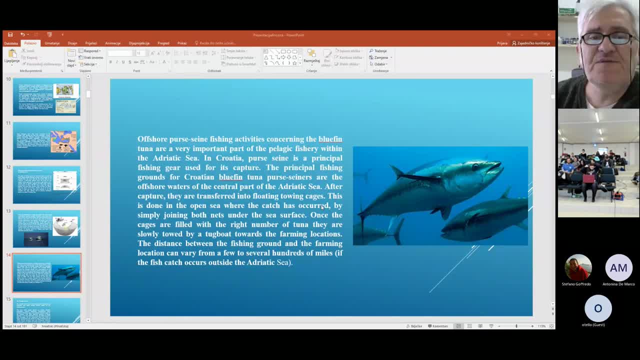 In Croatia. poor seine is a principal fishing gear Used for its capture, And the principal fishing grounds for Croatian poor seiners are the offshore waters of the central part of the Adriatic Sea, And after capture, they are transferred into floating towing cages. This is done. 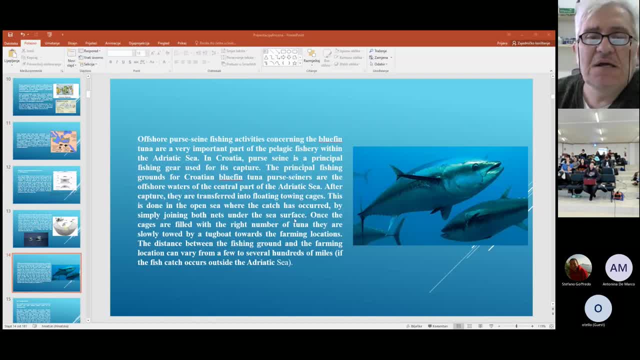 in the open sea where the catch has occurred by simply joining boat nets under the sea surface. Once the cages are filled with the exactly number of tuna, they with the right, let's say, number of tuna. they are slowly towed and tugged both towards the farming locations. The distance between the fishing ground and the farming location can vary. The distance between the fishing ground and the farming location can vary From a few to several hundreds of miles. if the fish catch occurs outside the Adriatic sea, Okay, We could say that the Adriatic sea is one of the largest. sorry, is the largest. 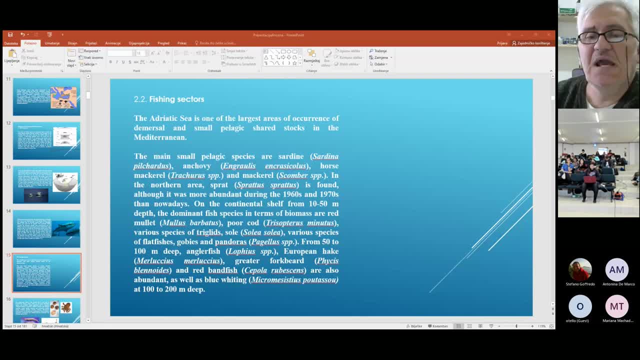 is the largest area of occurrence of the myrtle and small pelagic shared stocks in the whole Mediterranean And we could say that the main small pelagic species are the sardine, sardine afilhardo, jenchovii, engraurius and gracichoris, horse mackerel, trahurus, mackerel-scomber, and in. 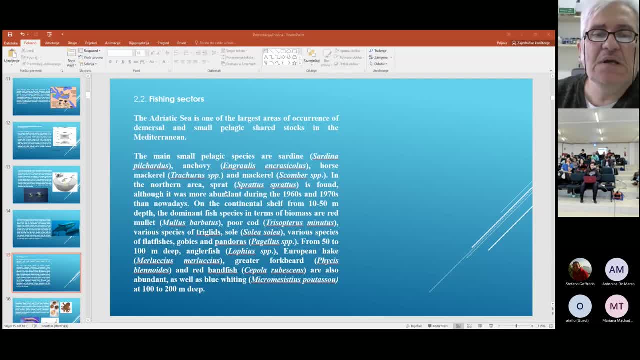 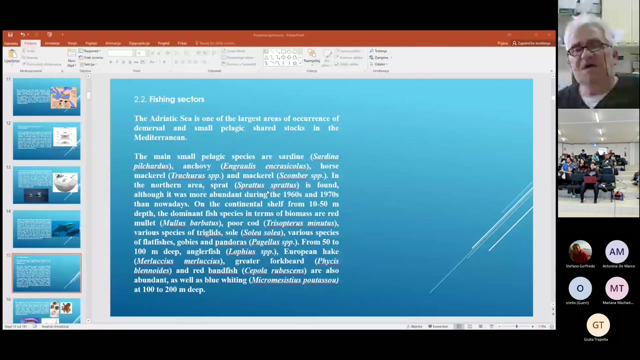 the northern area sprattus is found, although it was much more evident during the 60s and 70s than nowadays. Mostly, sprattus is collected from the eastern side, catched in the eastern side, and it is still present on the fish markets in the northern part, northeastern part of the Adriatic Sea. 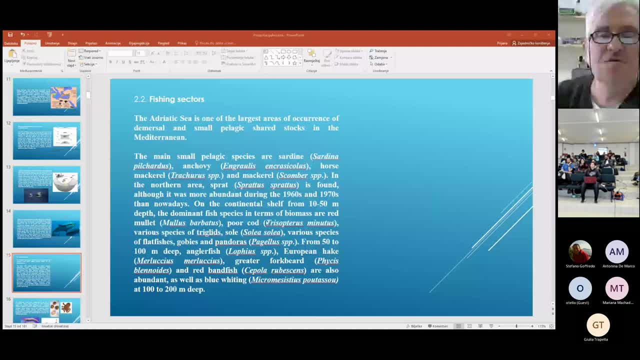 It lives on the continental shelf from 10 to 50 meter depth And it is, I think, according to my knowledge, is the only area in the Adriatic where Spratus is spawning So, practically in front of Kvarner region and islands in the and islands in the northern part of the Adriatic from the eastern side. 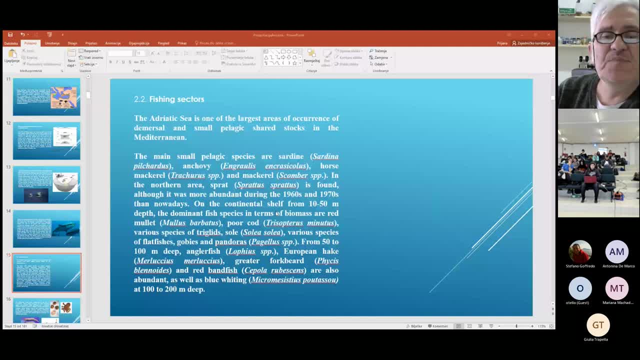 The dominant fish species in terms of biomass on the continental shelf, completely in the Adriatic, are, let's say, red mullet, Mulus barbatus, poor cod, Trisopterus minutus, some various species of triglitz, then Solea solea. 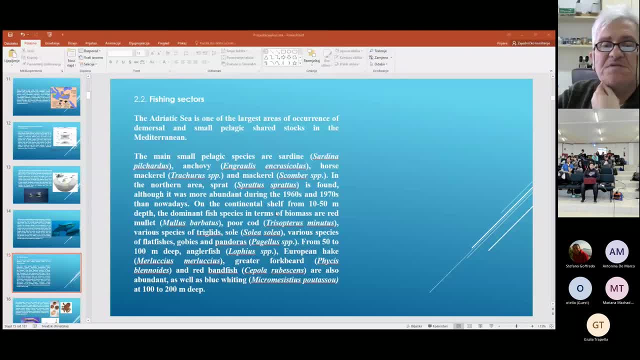 various species of flatfishes. gobies and pandoras means pagelus From 50 to 100 meter depth. there are anglerfish: lofius, European hake, Merlucius merlucius. 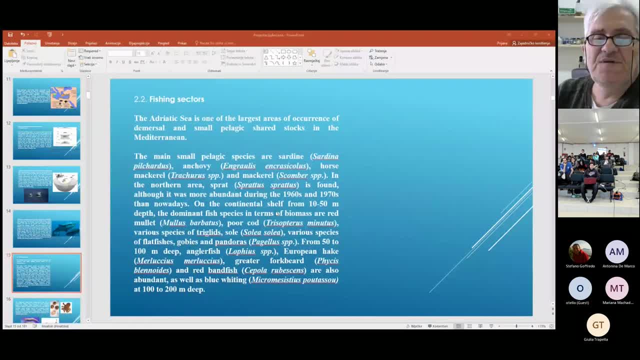 greater four-beard fetus Brenoides and Cepula red bandfish, Cepula rubenscens. I think they always change the name, Latin name, Cepula rubenscens, to Cepula macroftalma. 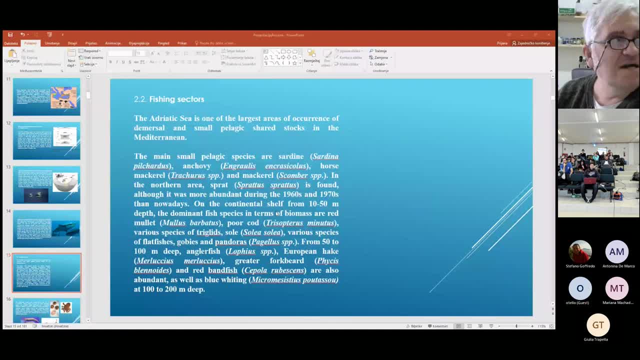 It depends on the results of taxonomists, Also evident, as another type of fish is, let's say, the red bandfish. Another type of fish is, or let's say target species is, blue whitening Micromecystis poutasso at 100 to 200 meter depth. 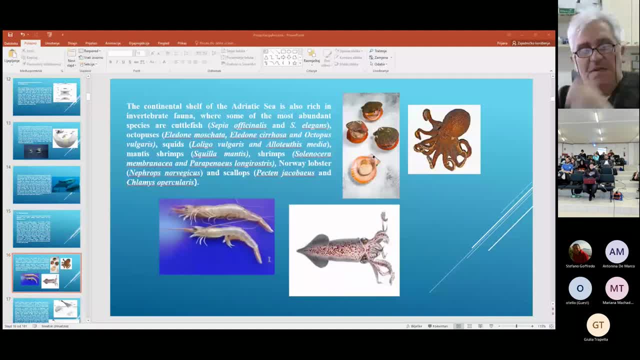 The continental. we could say that the continental shelf of the Adriatic Sea is also rich in invertebrate fauna, where some of the most evident species are cattlefish. Two type of species dominate: Sepia officinaris and Sepia elegans. 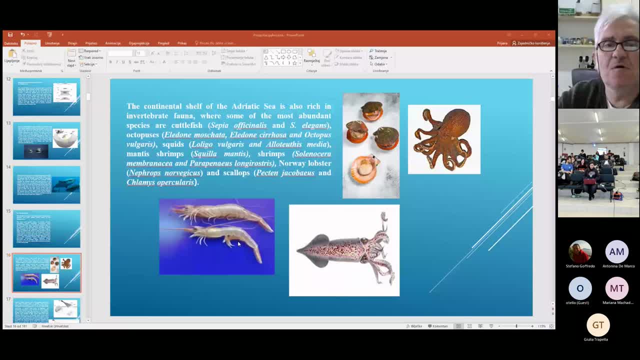 Octopuses, that's Ledona moshata, Ledona eziroza and Octopus vulgaris, Squids, Loligovulgaris And Aloteutis media, Mantis shrimps, for example Squillamantis. 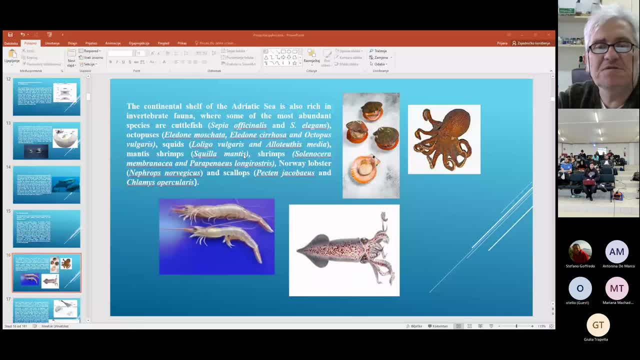 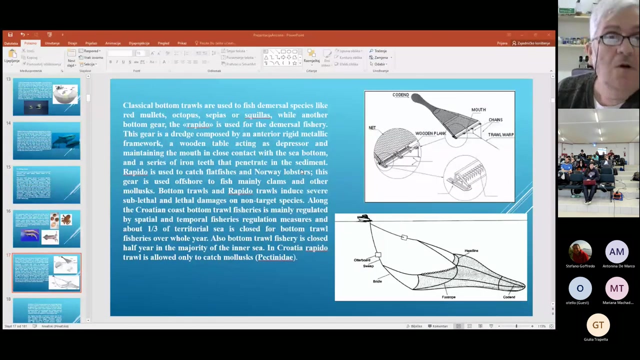 And Parapenaeus longirostris, Then Norway lobster, Nephrops norwegicus And some scallops, Pecten jacobeus and Chlamys opercularis. So we have come back on the type of fishing gears. 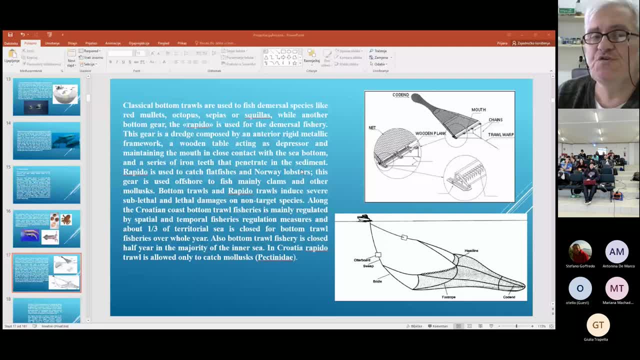 Classical bottom trawls are used to fish demersal species like red mallets, like octopuses, sepias, squillas, While another bottom gear the name is Rapido- I think that most of you knows that type of gear. 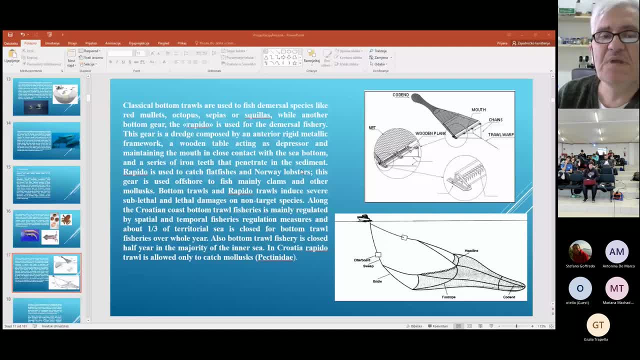 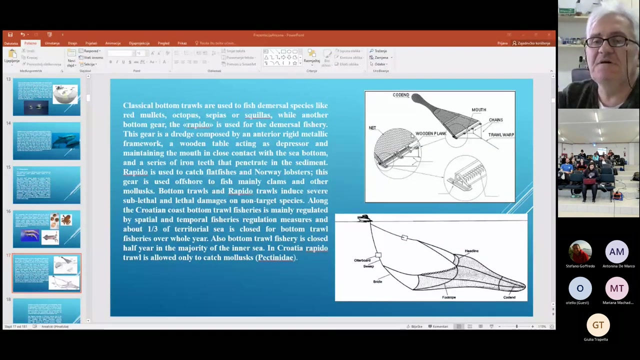 And it is used for the demersal fishery. Practically, this gear is dredged, composed by an anterior rigid metallic framework, a wooden table acting as a depressor and maintaining the mouth in close contact with the sea bottom, And the series of iron teeth that penetrate into the sediment. 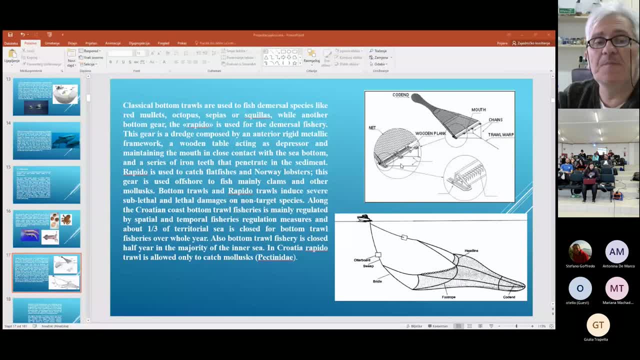 Rapido is used to catch flatfishes and Norway lobsters. This gear is used offshore to fish mainly clams and other mollusks. Bottom trawls and Rapido trawls induce several different species. It induces several subletal and lateral damages of non-target species. 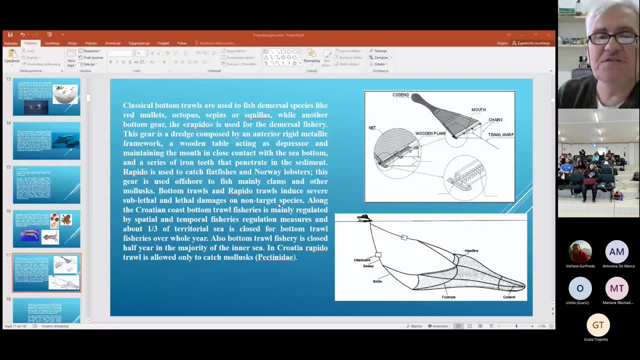 On the Croatian side. along the Croatian coast, bottom trawl fisheries is mainly regulated by special and temporal fisheries regulation measures, And about one third of territorial sea is closed for bottom trawl fisheries over the whole year. Also, bottom trawl fisheries close half year in the majority of the inner sea. 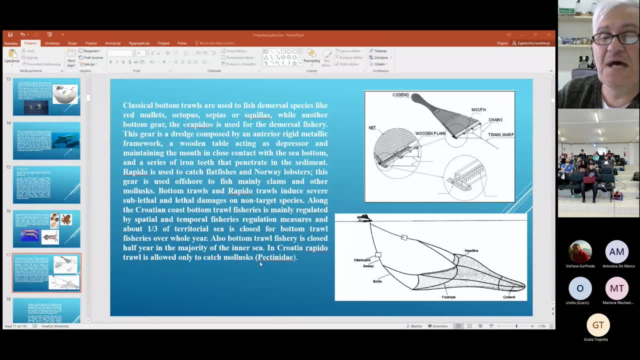 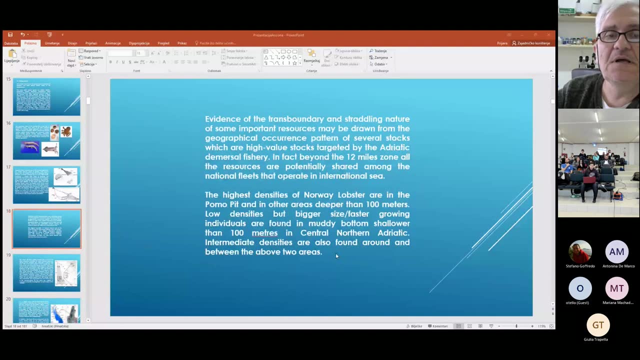 And on the Croatian side, Rapido type of Rapido trawl is allowed only to catch mollusks, Practically one family, pectinidae. So this is the case. Now let's go to the next part. 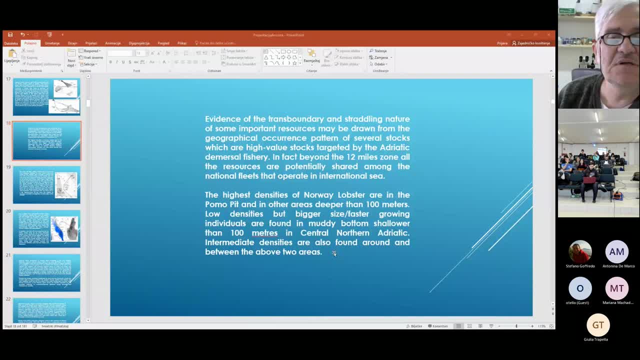 Evidence of transboundary and the straddling nature of some important resources may be drawn from the geographical occurrence pattern of several stocks which are high, very targeted by the Adriatic demersal fishery, In fact beyond the 12 miles zone. 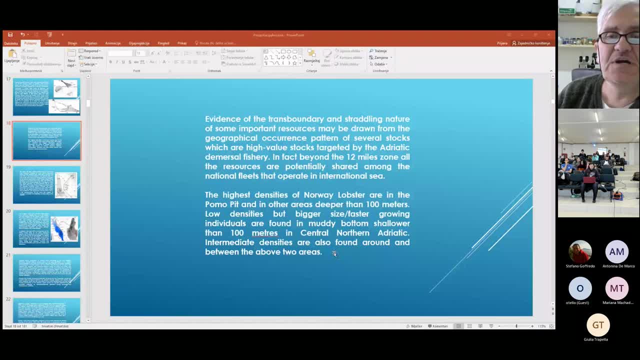 all the resources are potentially shared among the national fleets that operate in the international sea. The highest densities of, for example, Norway lobster are in the Pomo pit and in other areas deeper than 100 meters. Low densities but bigger size. 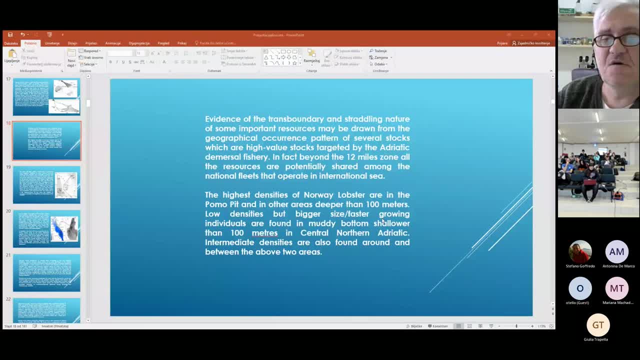 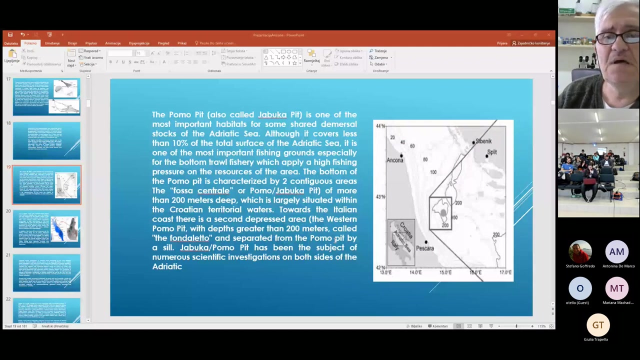 growing individuals. faster growing individuals are found in muddy bottom shallower than 100 meters in the central north part of the Adriatic, And intermediate densities are also found around and between the above two areas. We now come to the one of the most important. 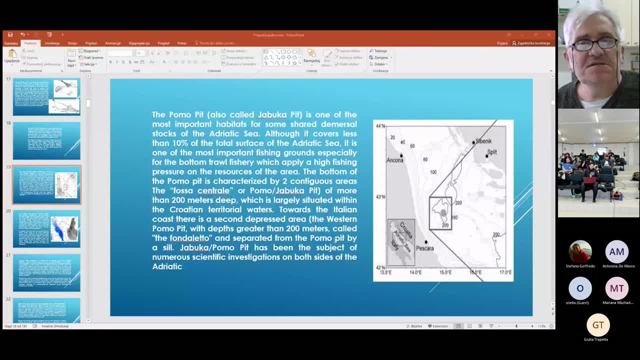 what I already mentioned, areas and habitats for some shared demersal stocks of the Adriatic Sea. Even though it covers less than 10% of the total surface of the Adriatic Sea, it is one of the most important fishing grounds, especially for the bottom trolleys fishery. 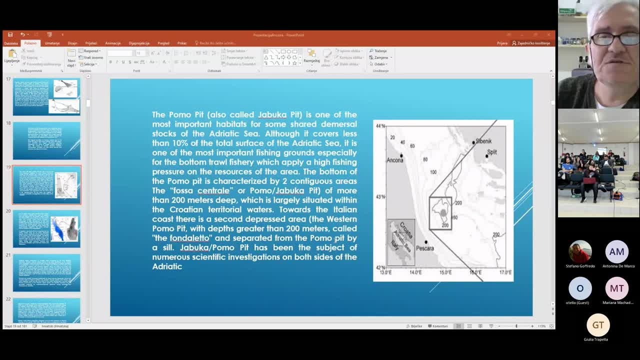 which apply a high fishing pressure on the resources of the area. The bottom of the Pomo pit is characterized by two contiguous areas: The fossa centrale or Pomo-Javuka pit of more than 200 meters depth, which is largely situated within the Croatian territorial waters. 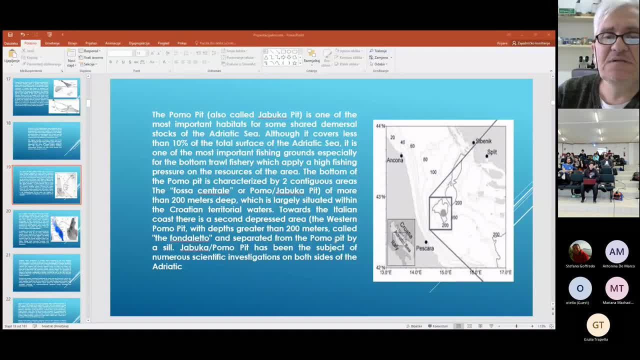 Towards the Italian coast, there is a second depressed area, the western Pomo pit, which, with depths greater than 200 meters, called the Fondaletto and separated from the Pomo pit by a silt, And, for example, Pomo pit has been the subject. 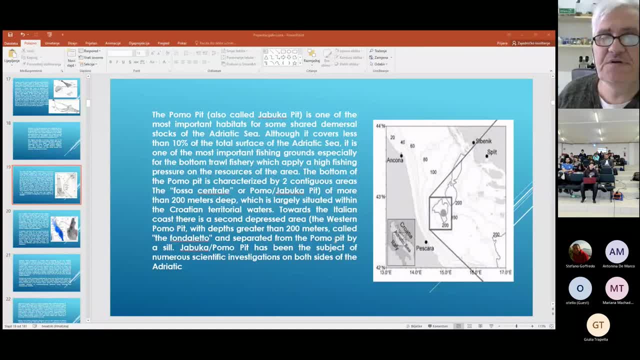 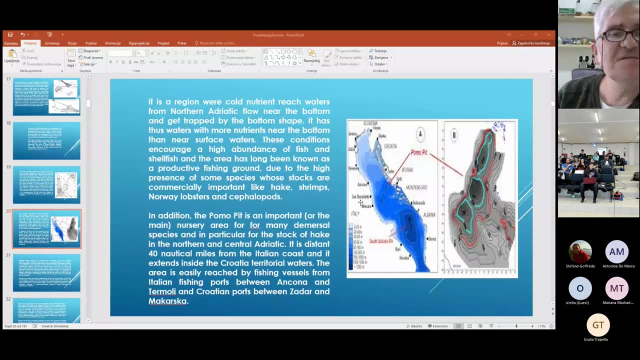 especially nowadays, the subject of numerous scientific investigations on both sides of the Adriatic. The Pomo pit is a region where cold, nutrient-rich waters from the Northern Adriatic flow near the bottom and get trapped by the bottom shape. It has thus waters with more nutrients. 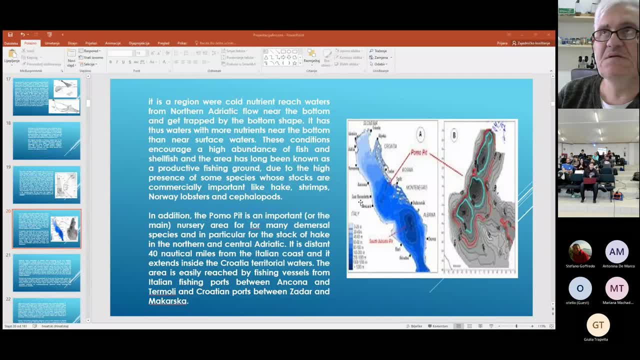 near the bottom than near surface waters. These conditions encourage a high evidence of fish and shellfish, and the area has long been known as a productive fishing ground due to the high presence of some species whose stocks are commercially important, such as hake. 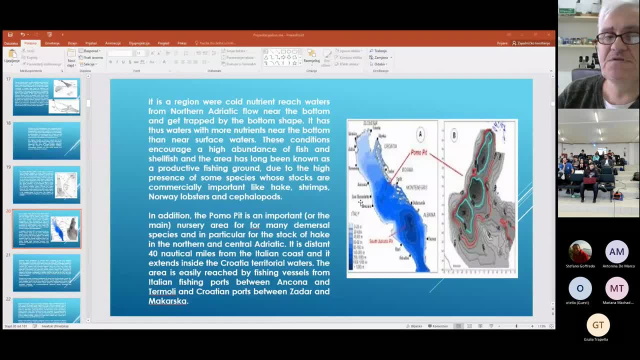 merlucius shrimps, Norway, lobsters and cephalopods. In addition, we could say that the Pomo pit is a very important or the main nursery area for the many dinosaur species and, in particular, for the stock of hake. 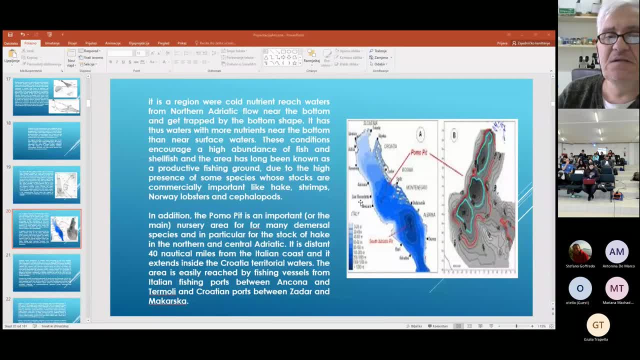 in the Northern and Central Adriatic. It is distant 14 nautical miles from the Italian coast and it extends inside the Croatian territorial waters. The area is easily, for example, reached by fishing vessels from Italian fishing ports between Ancona and Termali. 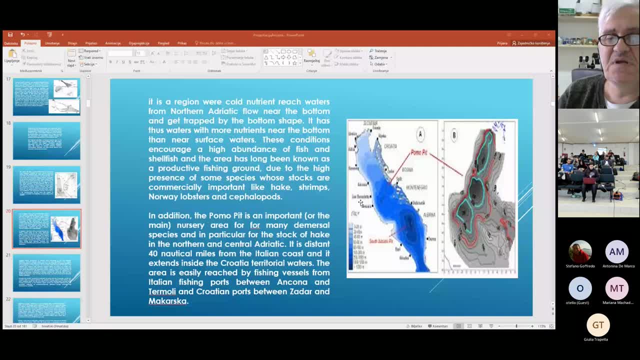 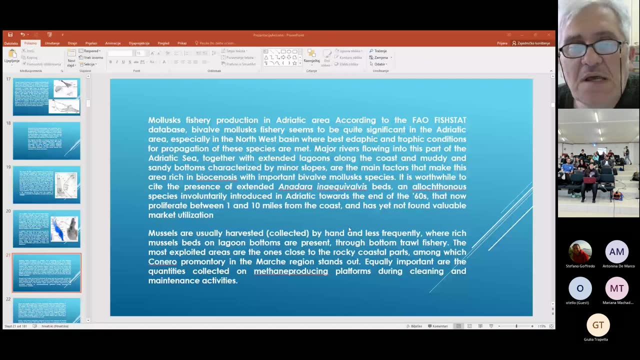 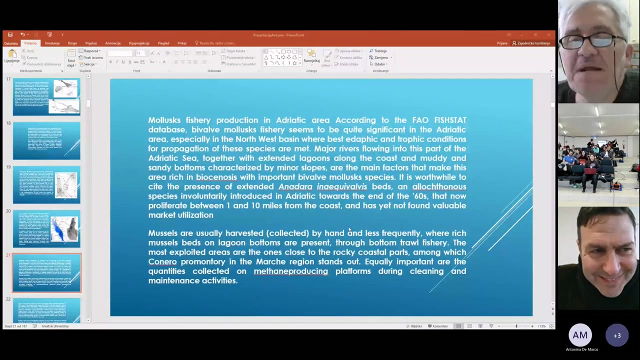 and from the Croatian side, from ports between Zadar and Makarska. Okay, I am suggesting now 10 minutes of break, because my lips and my mouth need some water. Okay, Okay, Jakub, See you in 10 minutes. 10 minutes, please. 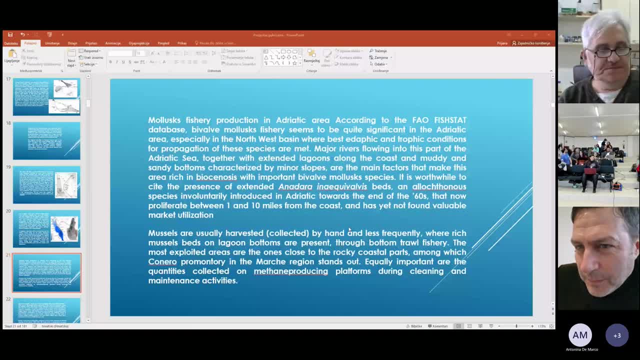 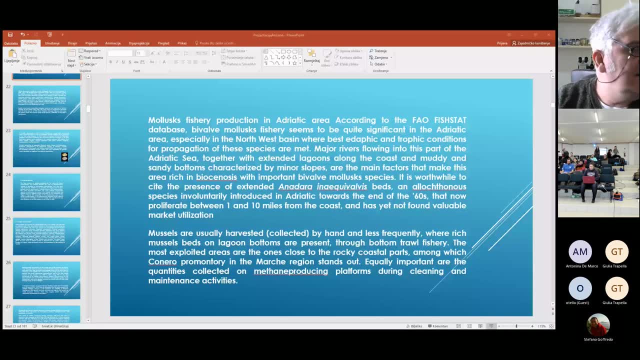 Thank you, Yes, Thank you. Bye, Okay, We will stop now. I need to say a few words about the mollusks fishery production in the Adriatic area. According to our fish stock database, bivalve mollusks fishery. seems to be quite significant in the Adriatic area, especially in the northwest basin, where best, best and the traffic conditions for propagation of these species: Major rivers flowing into this part of the of the of the Adriatic Sea, together with extended lagoons along the coast. 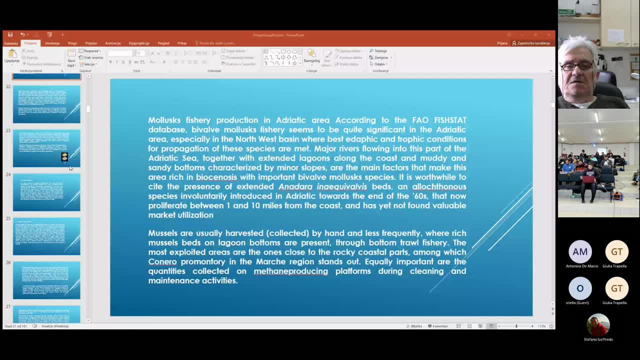 and the muddy and sandy bottoms. So these are the main factors which are characterized by minor slopes and are the main factors that make this area rich in biosynosis with important mollusks, bivalve mollusks species, For example, in this: 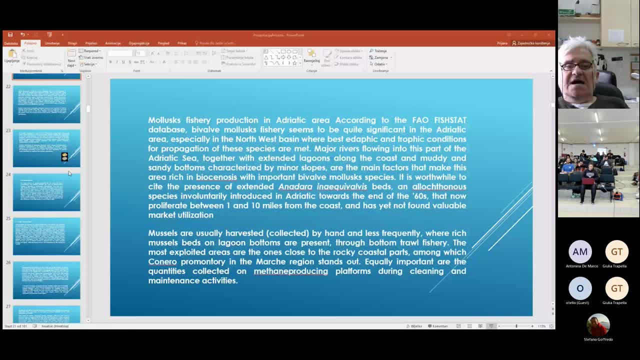 it is worthwhile to to cite the: the presence of extended the anandara in equi- bivalves, The beds on our loctonus site. the presence of the extended anandara in equa, which were involuntarily introduced into the Adriatic. 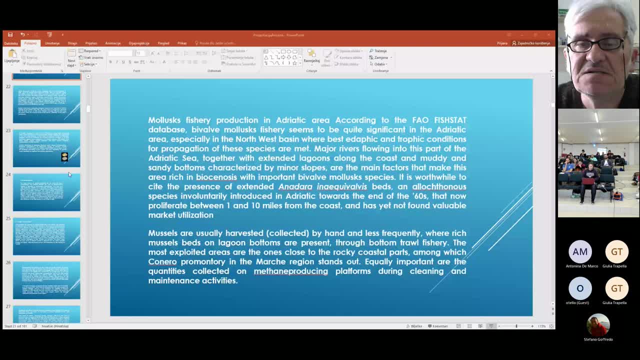 towards the end of the sixties, that now proliferate between the Central and Central Atlantic Fossils. They are still not found in a valuable market utilisation. Mossels are usually harvested, collected by hand, and less frequently in rich mossels które lagoon. 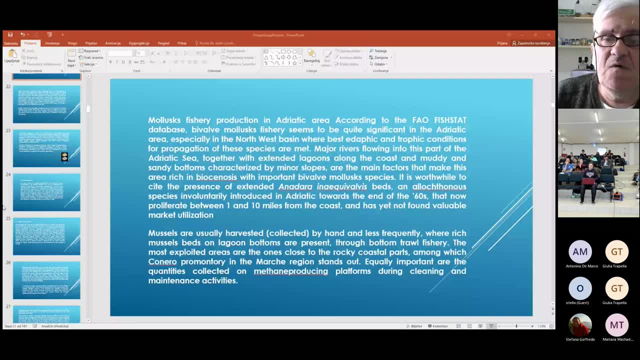 Marce region stands out. Equally important are the quantities collected of methane producing platforms during cleaning and maintenance activities. Clumps are usually caught by vessels equipped with hydraulic dredge. In 2000,, for example, out of 728 dredge boats. 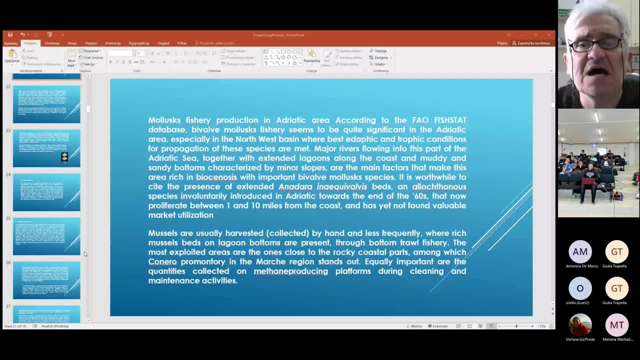 registered in Italy. 685 were operative along the Adriatic Coast. This fishery system operates on seddy bottoms with one mile from the coast. Normative applied to this capture system contains the following indications: Gears dimensions, catches limit, vessels dimensions, engine power clamp. 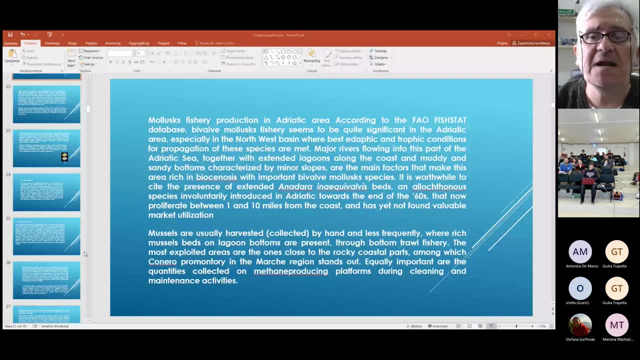 size, etc. Fishing areas are managed by compartmental management consortiums to which all fishermen are affiliated. Some of these vessels are used or other be well mollusks fisheries as well, such as smooth Calista, Calista Hione and other claims. 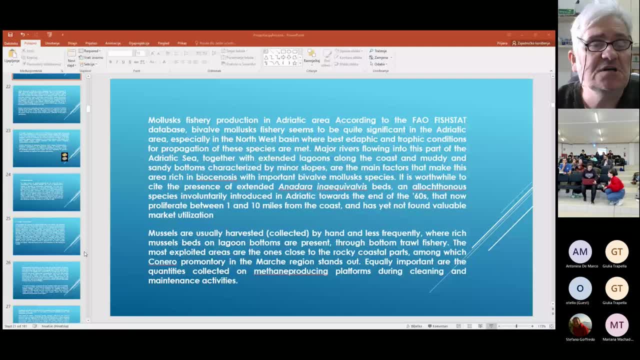 for example, Solon and Ensis Production is around 30,000 tons per year. Eastern coastal clams production is only reported for Albania, Albania referring to the period from 1987 to 1996.. The trend shows a progressive decrease from the initial amount. 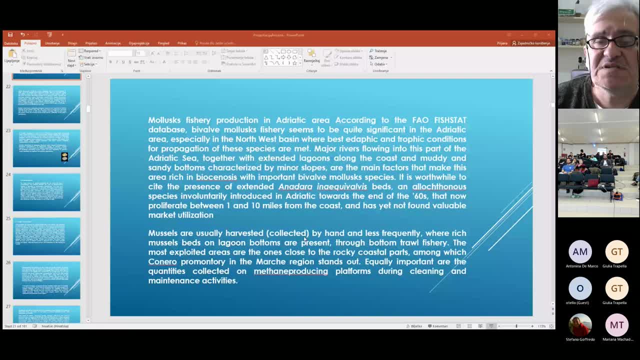 of 700 tons, according to Fao Fishtat. Although reduced clam beds are present along the northern coast of this country, collection of any kind is not allowed In Croatia, for example, particularly in the Northern Adriatic along the Istrian Peninsula coast. very important. 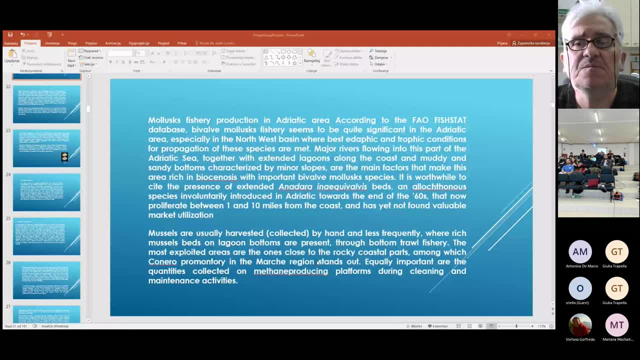 species is pectinia cobales, targeted by a good part of the fleet using dredges. In other areas, the capture fisheries of pectinidae has nowadays become marginal. In the past, pectinidae species were collected in the Northern Adriatic with the 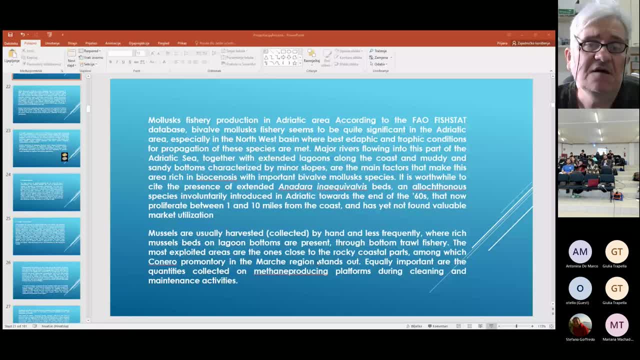 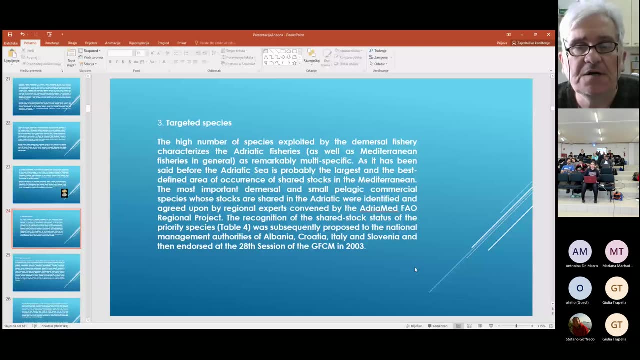 bottom trawl gears, called rapidi, rapido vessels equipped with the fixed dredges, originally constructed firstly for the flat fish fisheries, That there is a high number of exploited, of number of species exploited by the demersal fishery. What does it mean? 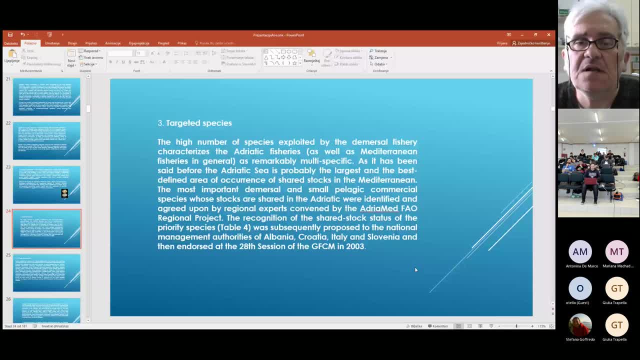 That means that it the number of the high number, characterize the Adriatic fisheries as well as Mediterranean fisheries in general, And that makes exploitation as or let's say the demersal fishery is remarkably multi-specific. As it has been said before, the Adriatic is probably the largest and 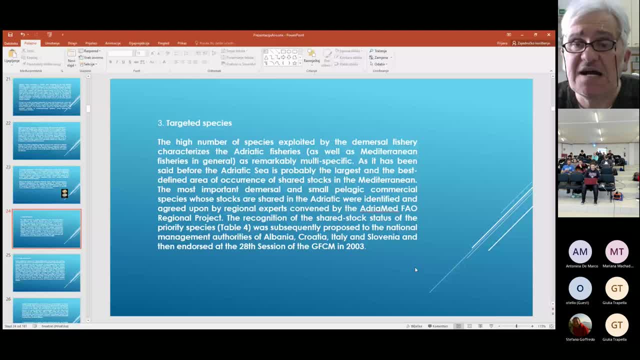 the best defined area of occurrence of shared stocks in the whole Mediterranean area. The most important demersal and the small pelagic commercial species whose stocks are shared in the Adriatic were identified and agreed upon the regional by the regional experts convened by the Adriamed FAO regional project. 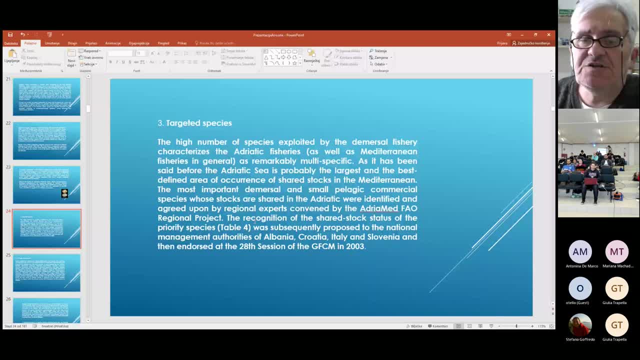 The recognition of the share stock status of the priority species was subsequently proposed by the national management authorities of Albania, Croatia, Italy and Slovenia, and then endorsed at the 28th session of GFCM General Fisheries Council for the Mediterranean in 2015.. 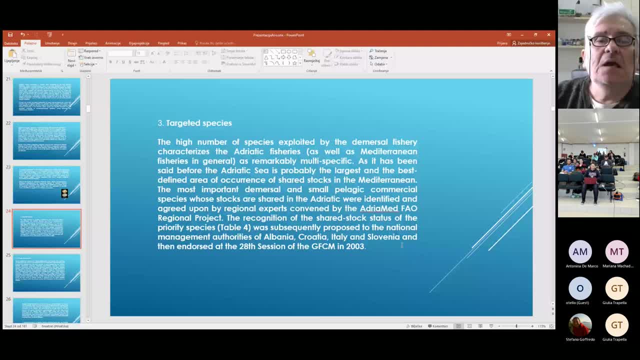 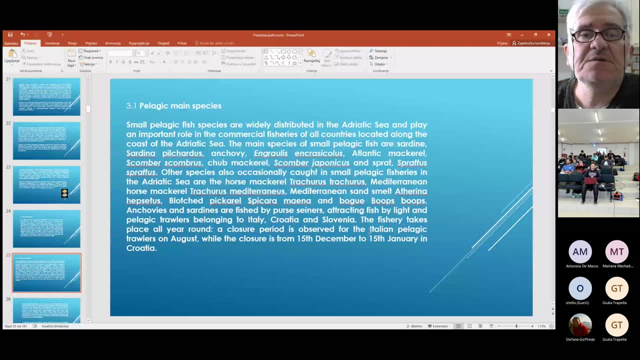 In 2015. 2003.. Now we will say about few words about the pelagic main species, Small pelagic fish species widely distributed in the Adriatic Sea and play an important role in the commercial fisheries of all countries located along the coast of the Adriatic Sea. The main species of small pelagic are sardine, sardinia pergados, anchovy and growlis, and crassiholus Atlantic mackerel, scomber, scombrus, chub mackerel. 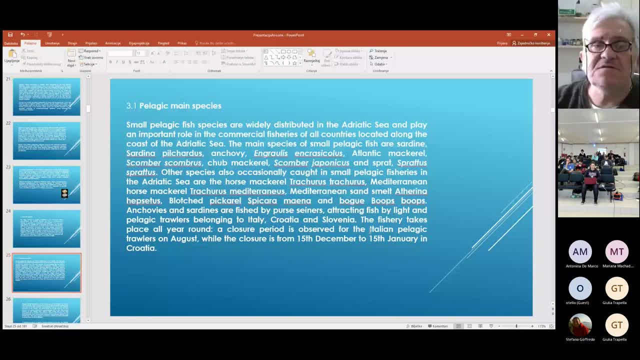 scomber japonicus and the sprat spratus spratus. Other species also occasionally caught in small pelagic fisheries in the Adriatic are the horse mackerel trahurus trahurus, then trahurus mediterraneus sand smelt- Mediterranean sand smelt. 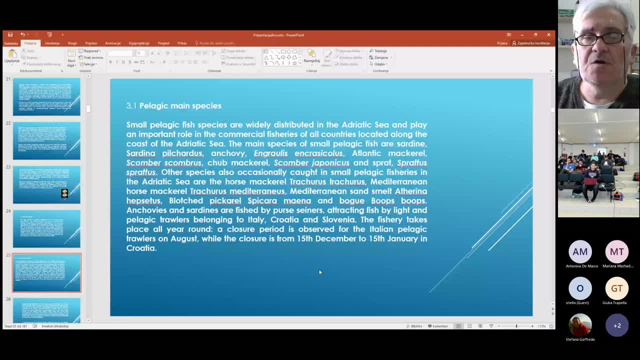 Atherina hepsaetus, pitcherer, blotched pitcherer, picara, maena and bug bups. bups, Anchovies and sardines are fished by poor sails attracting fish by light and pelagic trawlers belonging to Italy, Croatia and Slovenia. The fishery takes place all year around. Closure period is observed for the Italian pelagic trawlers on August, while the closure is from 15, what I said already- December to 15 January. in Croatia, Pelagic fishing fleet activity on the eastern part of the 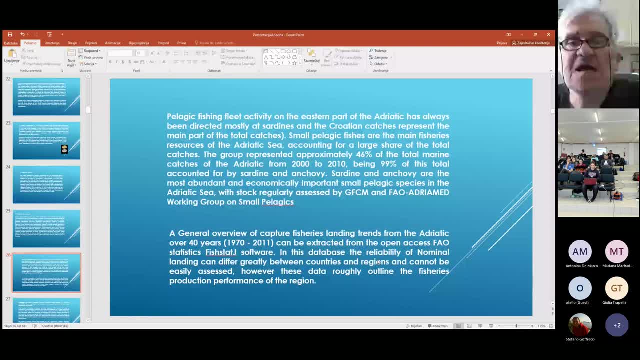 Adriatic has always been directed mostly at sardines, and the Croatian catches represent the main part of the total catches. Small pelagic fishes are the main fisheries resources of the Adriatic Sea, accounting for a large share of the total catches. The group represented approximately 46% of the total marine catches. 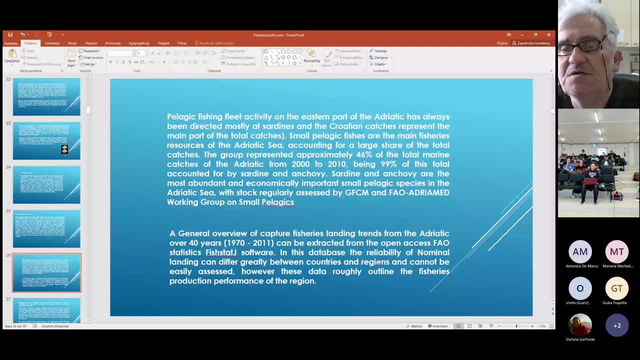 of the Adriatic, for example, for the period from the 2000-2010, being 99% of this total accounted for by sardine and anchovy. So sardine and anchovy are the most abundant and economically important. 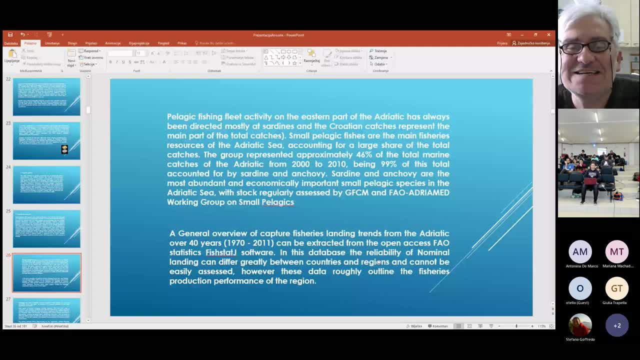 small pelagic species in the Adriatic Sea, with stock regularly assessed by GFCM and FAO AdriaMed working group on small pelagic fishing. For example. I was that the member of the AdriaMed working group, but not in previous times. 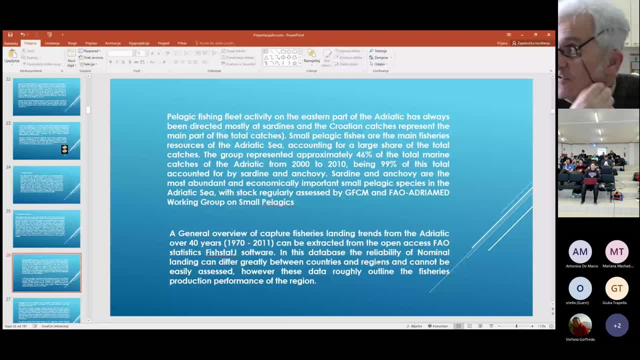 I was on that small pelagics, but now I'm from the coastal resources, So I was the member of the FAO AdriaMed working group, but in previous times for small pelagics, But now I think that part of the 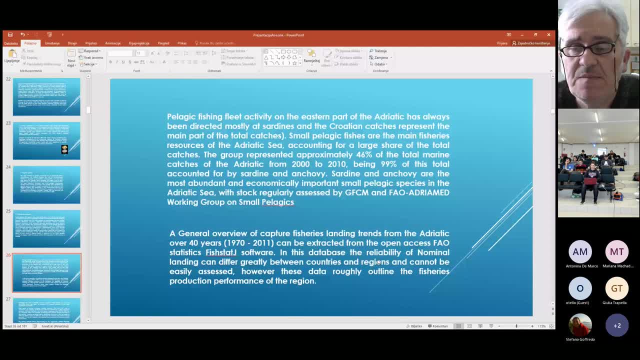 AdriaMed group is finishing there. I think that, finishing now their activities, Let's go on. a general overview of capture fisheries landing trends from the Adriatic over 40 years, from 1970 until 2011, can be extracted from the open assets. 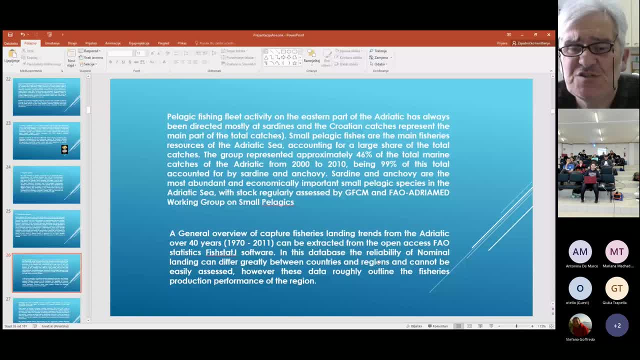 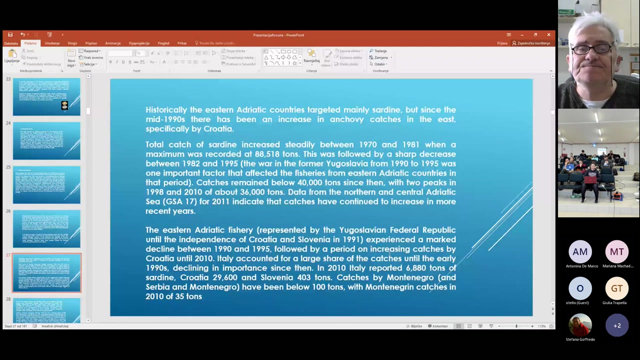 So FAO statistics, fish stats software in this database. The reliability of nominal landing can differ greatly between the countries and regions. It cannot be easily assessed. However, these these data roughly outline the fisheries production performance of the complete region. Historically, the Eastern Adriatic countries targeted mainly sardine. but since the mid 90s there has been an increase of anchovy catches in the East, specifically by by Croatia. Total catch of sardine increased steadily between 1970 and 1990.. When the maximum was recorded at around the 90,000 tons. This was followed by a sharp decrease between 1982 and 1995.. The war in the former country Yugoslavia from 1990 to 1995 was one important factor that affected the fisheries from the Eastern part of the Eastern Adriatic countries in that period. Catches remain below 40,000 tons since then, with two peaks in 1998 and 2010 of about 300,000 tons of sardine. So the average catch of sardine in the Eastern part of the Eastern Adriatic countries. 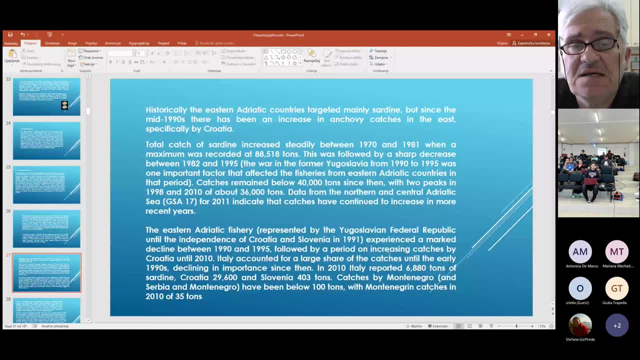 Tons 36,- sorry tons. data from the Northern and Central Adriatic, from the area sub-region and area 17 for 2011,. indicated catches have continued to increase in more more recent years. The Eastern Adriatic fishery, which was represented by the Yugoslavia. Republic until the independence of Croatia and Slovenia in 1991, experienced a marked decline between 1990 and 1995, followed by a period of increasing catches by Croatia until 2010.. Italy accounted for a large share of the catches until the early 90s, declining in importance since then. 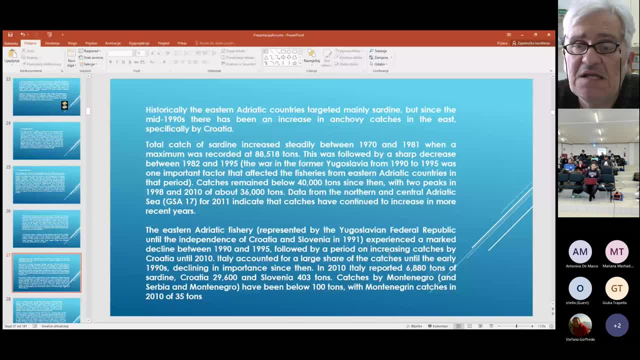 And in 2010,, Italy reported 688 tons of sardine, Croatia 29,600.. And Slovenia 403 tons. Catches by Montenegro and what was before Serbia and Montenegro as it represents ex-EU Yugoslavia, one part of Yugoslavia. have been below 100 tons, with Montenegro catches of 35 tons in 2000 and 2010.. For example, in 2011, the closure season for the Italian fleet was extended to 60 days. August and September, A large catch dominated the marine fish landing. particularly in the east And part and in the East Coast fishery, even though from the mid-80s the contribution of pelagics of total fish landings decreased remarkably as a consequence of the Sussexing downsizing of the anchovy and sardine stocks. and, more recently, of the economic changes which took place in the eastern coastal countries. Anchovy catches increased between the 70s and 1970s- This was in 1597 and 1784, reaching about 42 and 900 tons, decreased to 18100 tons in 1977. Increasing sharply in the following two years. the fishery attained its maximum historical level in 1979, when 62. 223? The fatty caught Box- Yes, two tons landed Catches- collapsed afterwards, reaching the historical minimum in 1987, 755 tons. The collapse of fishery. was followed by a period of relatively stability in catches, which oscillated around 10,000 tons per year from 88 to 92. The fishery experienced a recovery since then, reaching the peak of in 2006.. Catches declined after that, being about 46,000 per year. 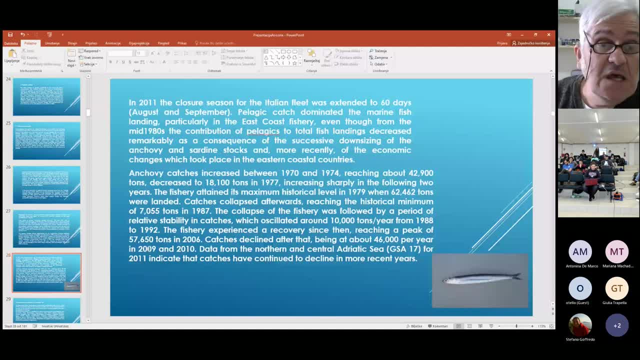 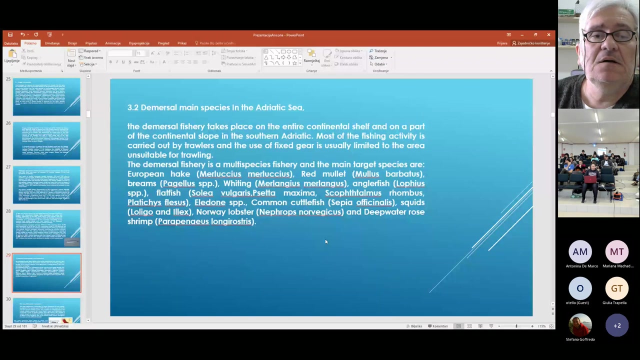 in 2006.. In 2009 and 2010.. Data from the Northern and Central Adriatic for 2011 indicate that catches have continued to decline. That is important to remember. The Merzelman species: It fishery: the Merzel fishery takes place on the entire 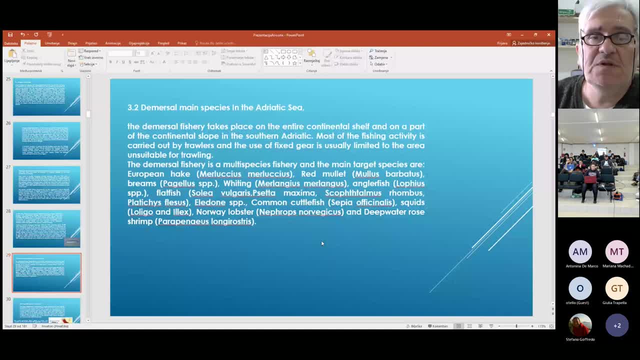 continental shelf on the part of the continental slope in the southern part. Most of the fishing activities carried out by the trawlers and the use of fixed gear is usually limited to the area unsuitable for trolling. The Merzel fishery is multi species fishery and the main target species are European. 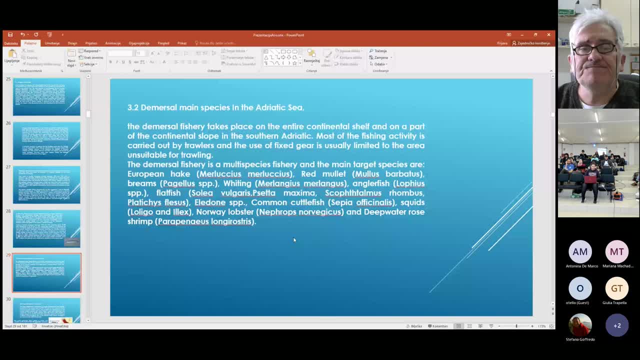 hake. Merlucius Red mullet. Murus barbatus, Pagelus breams, White-nig, Melangius melangus, Anglerfish, Lophius Flatfish, Solia vulgaris, Pseta maximus, Cotanus rhombus Patectis flesus. 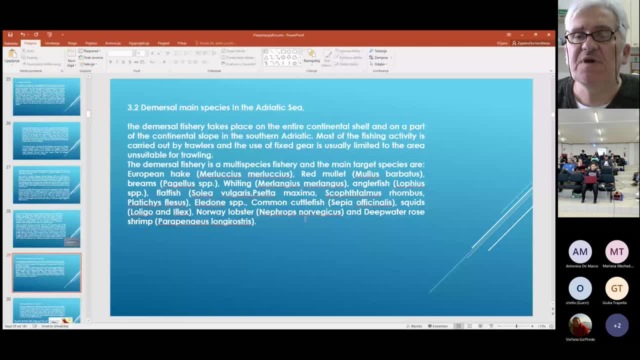 Eredonae, common catfish, Sopia ficinaris, squids, Norway lobster and deepwater roe shrimp, Parapenaeus longirostris, The Merzel fishery. what I said, I think, in the previous presentation, part of 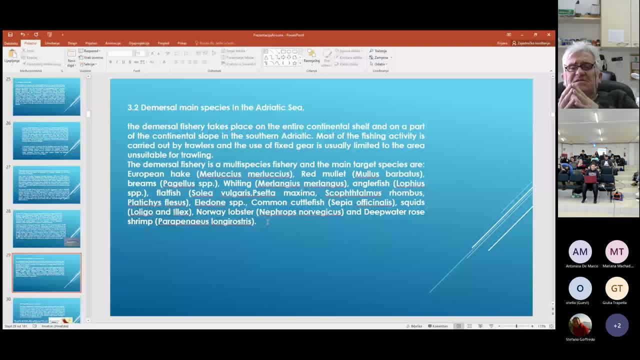 the presentation was this difference between the trawl catches and the Merzel fishery and the main main species which were inside, So practically more in the part of more southern than the northern part, so practically central and the southern part, the catches are. 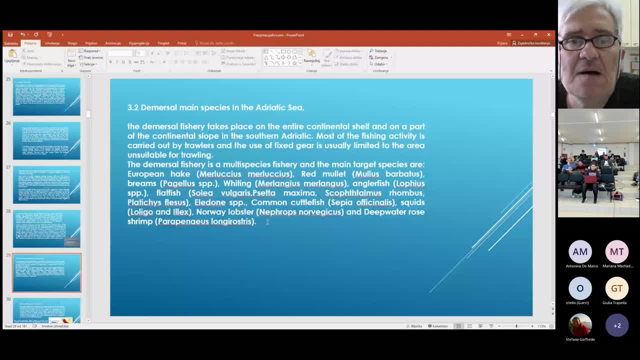 mostly by the main catches are mostly connected with the Merlucius and Mulus, for example, and the northern part is connected with the Merlangius and White-nig, Meami Official and Flatfish Solia. Practically that was connected with the, of course for the. 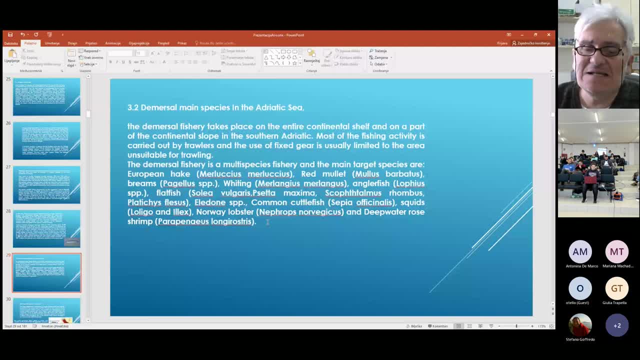 southern and Afros. so, practically, that is the that is connected with the, this difference between the boreal fauna which, for example, the member of the boreal is Melangius melangus, and, for example, more southern part, which 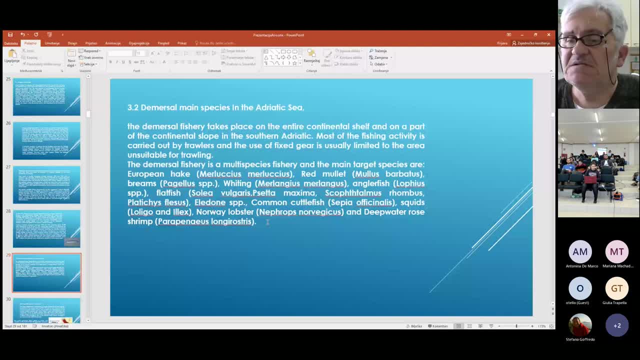 is connected with the Merlucius. So practically that is that theory of boreal existence of boreal species in the Adriatic Sea. So there is a difference between inside the Merse fishery, between northern and the southern part of the Adriatic. 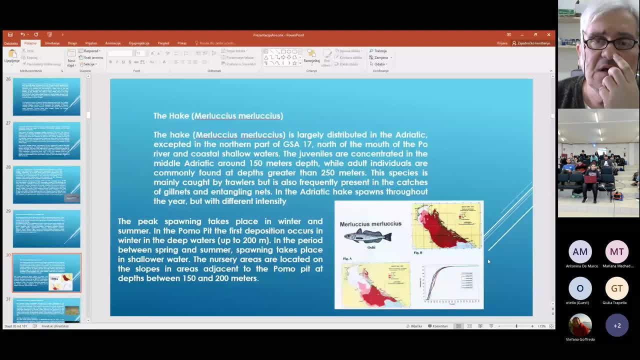 The hake is largely distributed in the Adriatic, excepted in the northern part of GSEA 17, north of the mouth of the poris And, of course, the shallow waters. The juveniles of the hake are concentrated in the middle Adriatic around the 150 meters depth. 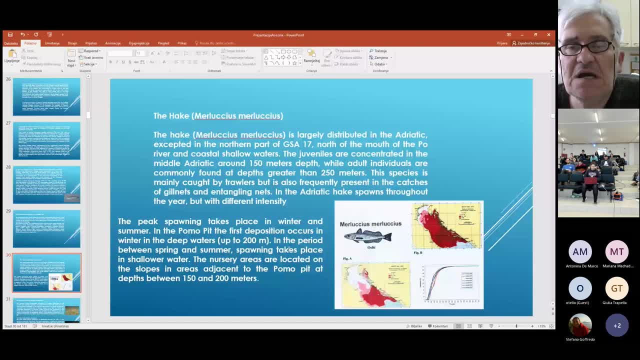 while adult individuals are commonly found at the depths greater than 250 meters. This species is mainly caught by trawlers, but it is also frequently present in the caches of gill nets and entangling gnats In the Adriatic practically hake. Adriatic hake spawns throughout the year, but with a different intensity, So the peak spawning takes place in winter and summer. In the Pomo pit, the first deposition occurs in winter, in the deep waters up to 200 meters And in the period between spring and summer. spawning takes place in shallower water, According to the nursery areas. the nursery areas are located on the slopes, in areas against to the Pomo pit and depths between 150 and 200 meters. Another species is Norway lobster- Nephrops norwegicus. 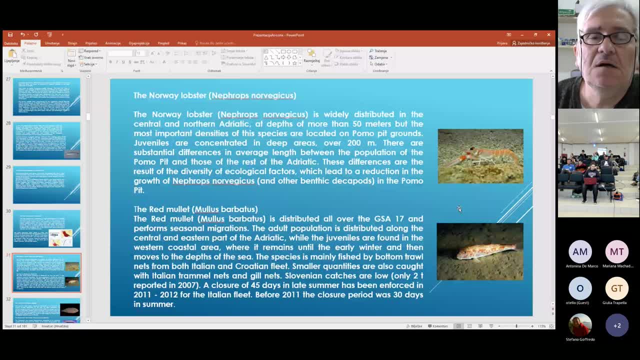 It is widely distributed in the central and the northern Adriatic at the depths of more than 50 meters, But the most important densities of this species are located on Pomo pit grounds. Juveniles, Juveniles, Juveniles. 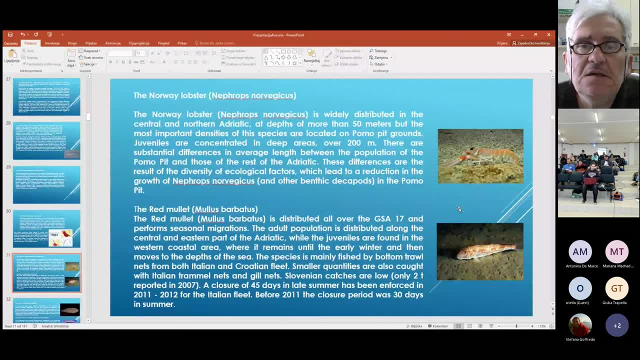 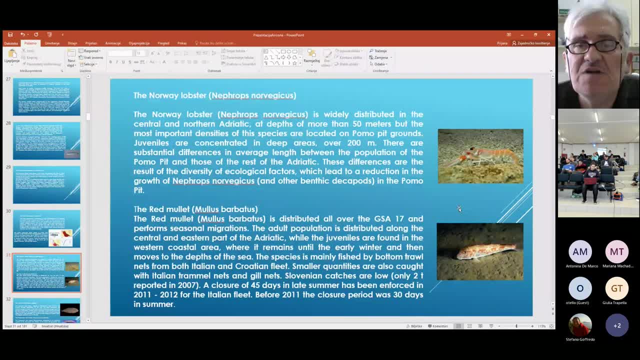 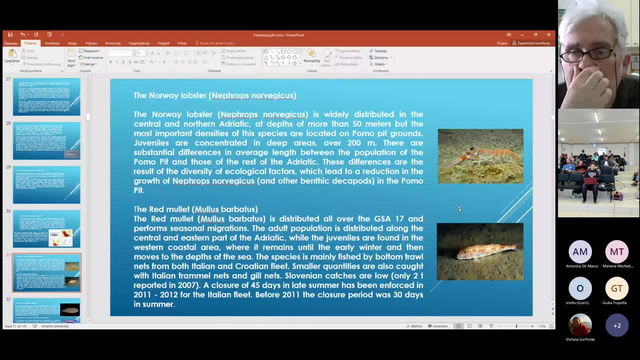 Juveniles. Another species is the red mullet. Mullus barbatus is distributed all over the GSEA 17 and performs seasonal migrations. The adult population is distributed along the central and eastern part of the Adriatic, while the Juveniles are found in the western coastal area, where it remains until the early winter and then moves to the depths of the sea. 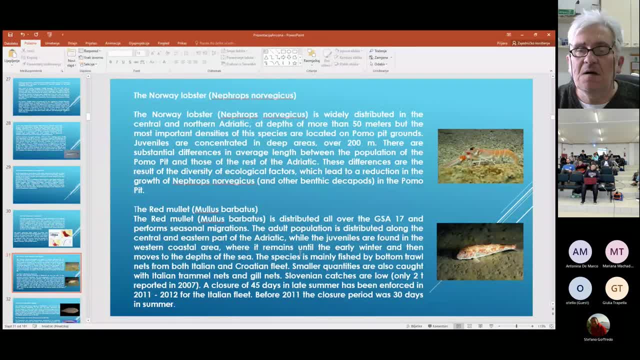 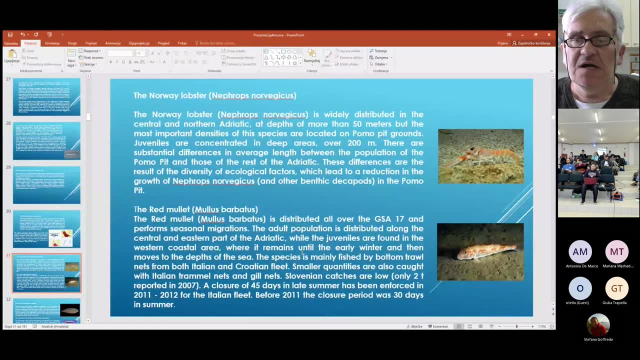 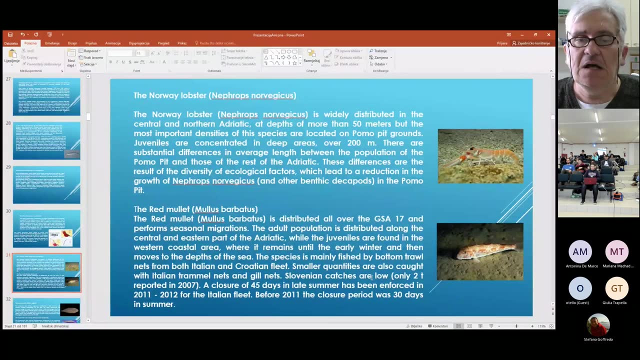 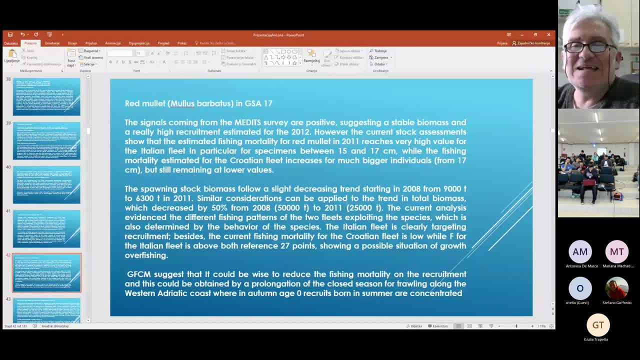 The sprouting stock biomass follow a slight decrease in trends starting in 2008. The sprouting stock biomass follow a slight decrease in trends starting in 2008 from 900 tonnes into Jazz 6,300 tonnes in 2011.. Similar considerations can be applied to the trend in total biomass. 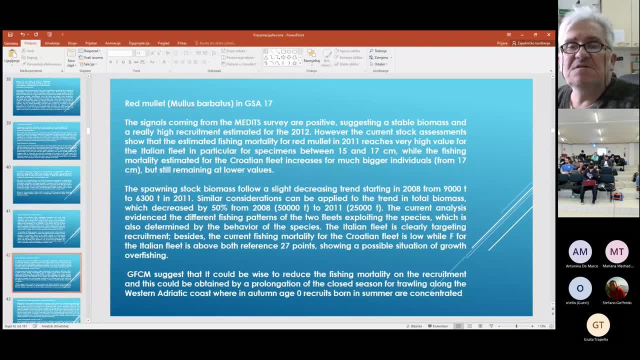 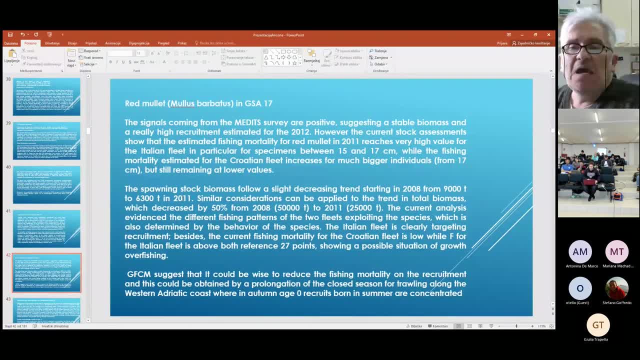 which also determined by the behavior of the species. The Italian fleet is clearly targeting recruitment. besides the current fishing, mortality for the Croatian fleet is low, while mortality for the Italian fleet is about both reference points showing a possible situation of growth over fishing. GFCM suggests that it could be wise. 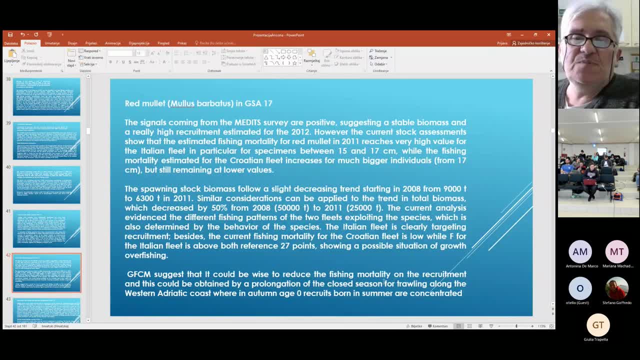 to reduce the fishing mortality on the recruitment and this could be obtained by a prolongation of the growth season for trolling along the Western Adriatic coast, where in autumn age zero recruits born in summer and where is the concentrated Parapenemus longirostris in GFC 18.. 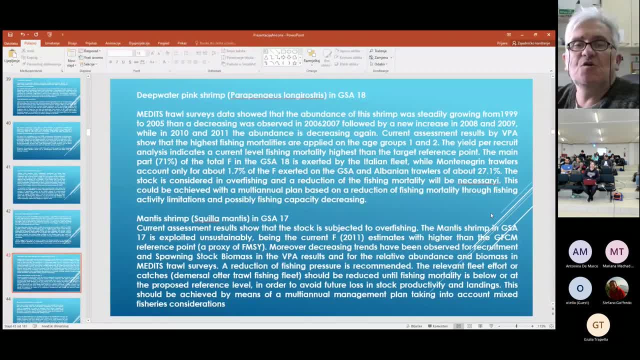 Meditz trolling surveys, data show that the abundance of this shrimp was steadily growing from 1999 to 2005.. The increasing was observed in 2006,, 2007,, followed by a new increase in 2008 and 2009.. 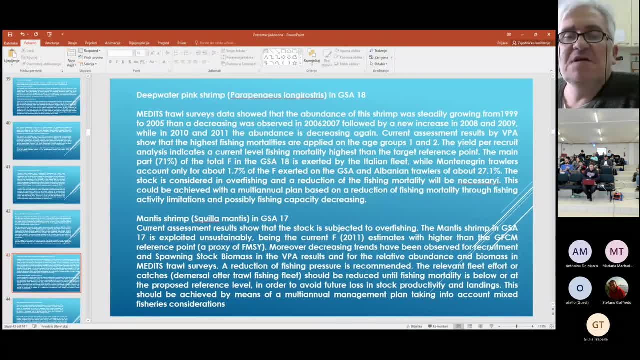 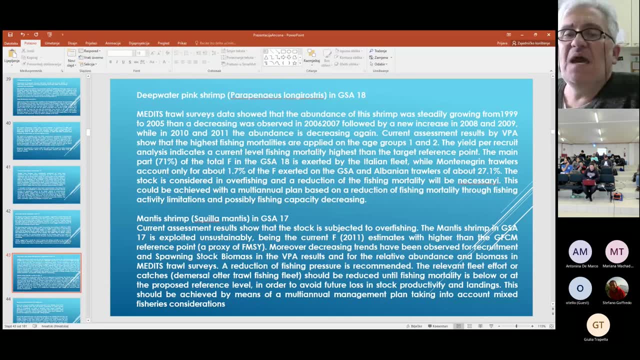 While in 2010 and 2011, the evidence is decreasing again. Current assessment: Current assessment Results by VPA virtual population analysis show that the highest fishing mortalities are applied on the age groups 1 and 2.. The yield per decruit analysis indicates a current level fishing mortality highest than the targeted reference point. 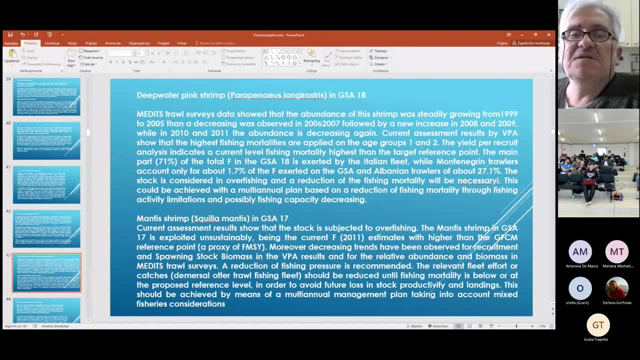 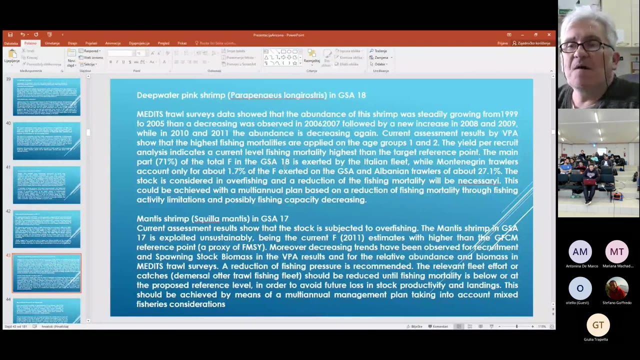 So the main part- 71% of the total mortality in the GSEA 18 is exerted by the Italian fleet, while Montenegrin trawlers account only for about 1.7% And mortality exerted on the GSEA and Albanian trawlers of about 27.1%. 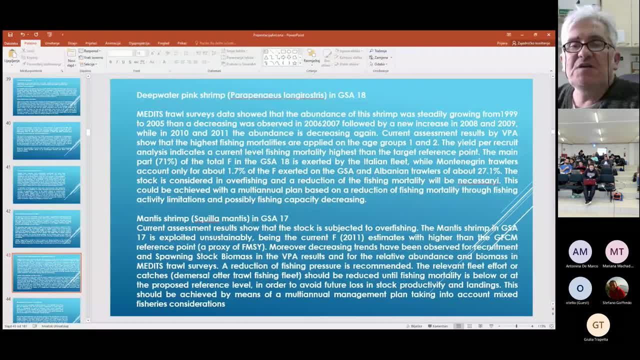 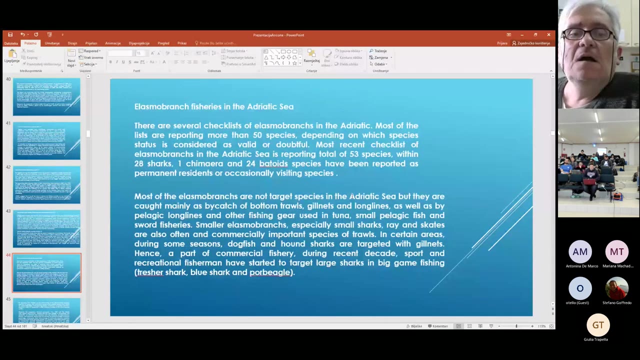 The stock is considered In overfishing and a reduction of the fishing mortality will be necessary. This could be achieved with the multi-annual plan based on a reduction of fishing mortality through fishing activity limitations and, possibly, fishing capacity decreasing. Squillamantis in GSEA 17.. 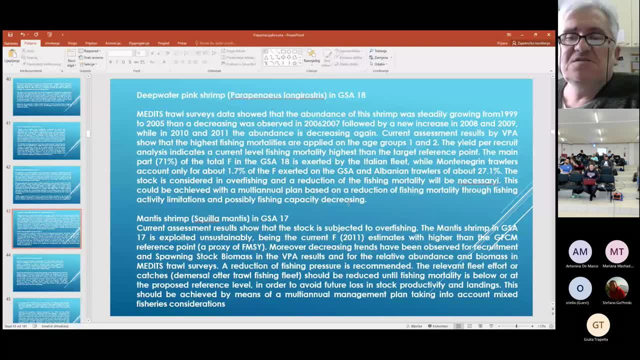 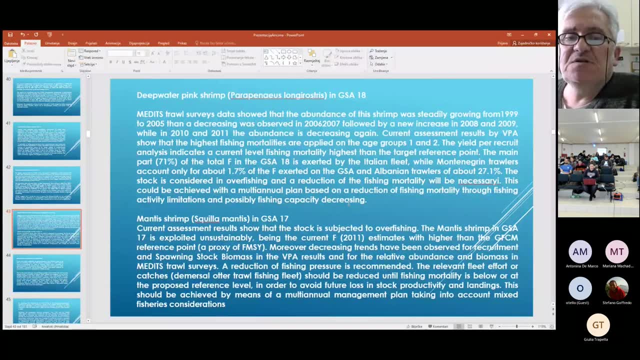 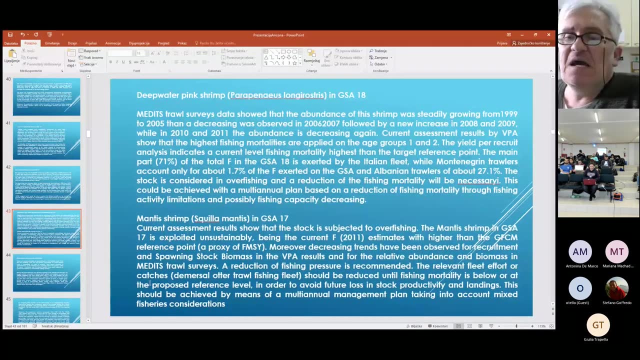 Current assessment results show that the stock is Subjected to overfishing. The main and the mantis shrimp in GSEA 17 exploited unsustainable, Being the current fishing mortality in 2011 estimates with higher than GSEA reference point. Moreover, decreasing trends have been observed for recruitment and spawn stock biomass in the VPA results. 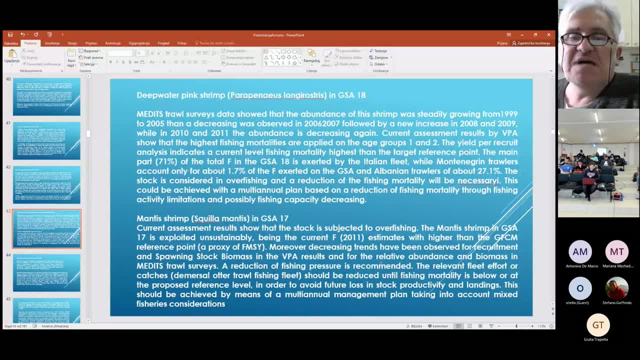 And for the relative evidence and biomass in Meditstroll surveys. A reduction of fishing mortality. A reduction of fishing mortality, A reduction of fishing pressure is a recommended. The relevant fleet effort or catches should be reduced until fishing mortality is below or at the or at the proposed reference level, in order to avoid future loss in stock productivity and landings. 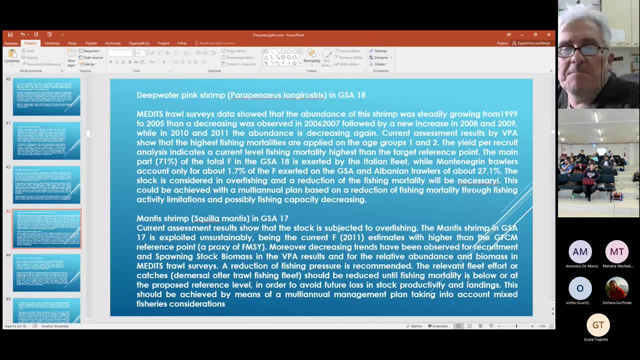 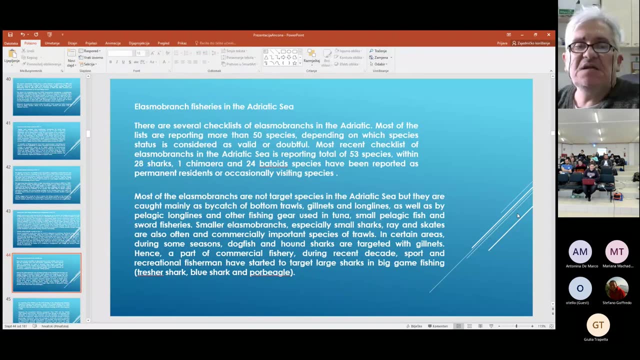 This should be achieved By means of multi-annual management plan taking into account mixed fisheries considerations. By means of multi-annual management plan taking into account mixed fisheries considerations. By means of multi-annual management plan taking into account mixed fisheries considerations. Few words about the elastobranch fisheries in the in the Adriatic sea. 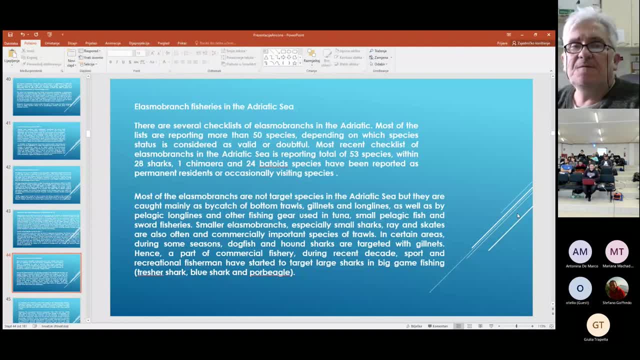 Several checklists of the elastobranchs in the Adriatic. Most of these- Most of these Are lists- are reporting more than 50 species, depending on Which species status is convenient, considered as valid or adaptable. most recent checklists of the elasmobranchs if the adriatic 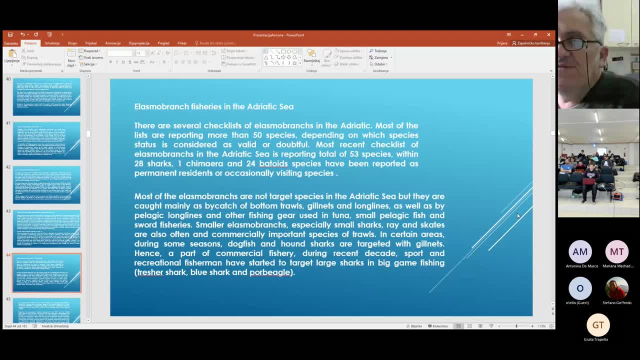 sea is reporting total of 53 species within 28 sharks, one himera and 24 battery species have been reported as the permanent residents or occasionally visiting species. uh, most of the elasmobranchs are not target species in the adriatic sea but they are caught. 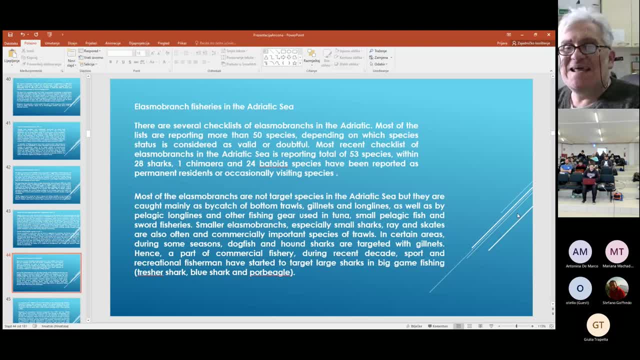 mainly as bycatch of bottom trolls, gill nets and long lines, as well as by pelagic long lines and other fishing gears used in tuna, small pelagic fish and sword fisheries. smaller elasmobranchs, especially small sharks, rays and skates, are also often and commercially important. 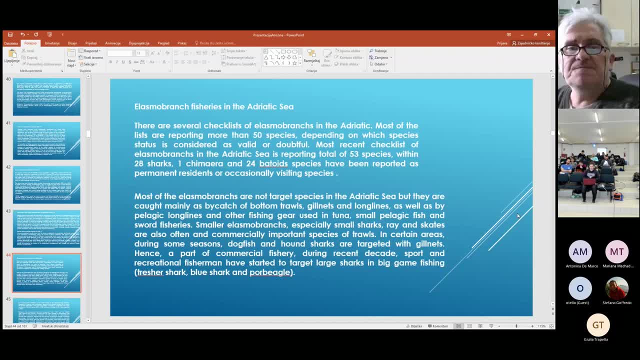 species of trolls in certain areas during some seasons, dogfish and hound sharks are targeted with gear nets as a part of commercial the fishery. during the recent decade, sports and recreational fishermen have started to target large sharks in big game fishing, so practically this type of fishing, including big game. it has now also has a part. 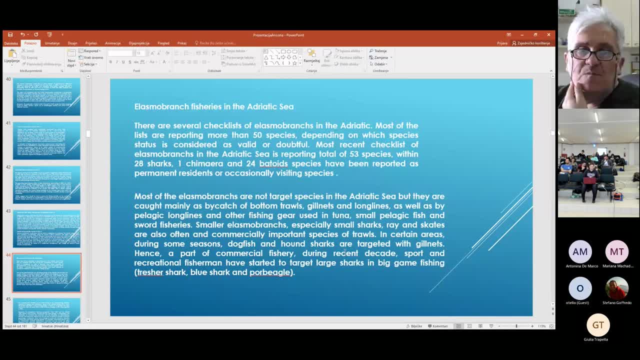 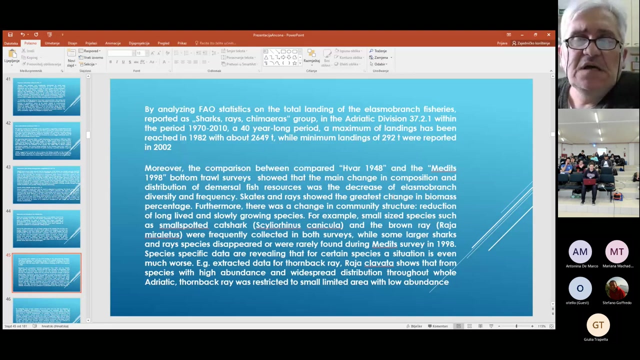 as a target species. for example, treasure shark, blue shark and poor beagle in big game fishing are the targets also from the elasmobranch and we could include it in elasmobranch fisheries and if we analyze uh fao statistics and the total landing of uh of elasmobrand fisheries. 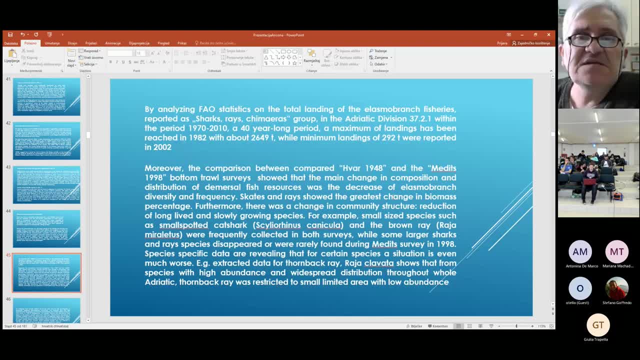 reported, as in false statistics, sharks, rays and hymeras group in the adriatic division within the period 1970- 2010, a 40 year long period, the maximum of lending has been reached in 1982 with about 2600 249 tons, while minimum landings of just 292 tons were reported in 2002.. 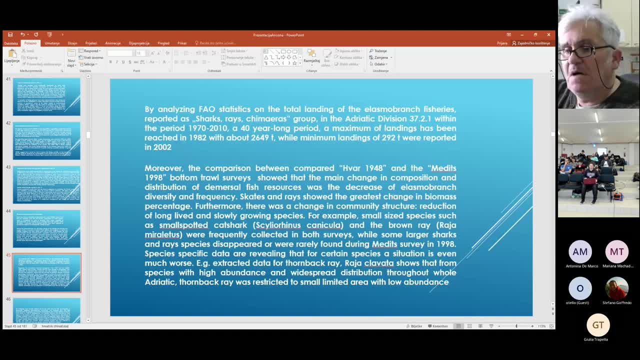 If we compared expedition, one of the most important expeditions in the Adriatic Sea which were connected with the Mars resources- practically there is a sentence here in the institute that was expedition which targeted the virgin populations in 1984, because the year suggests that it was almost immediately after the Second World War. 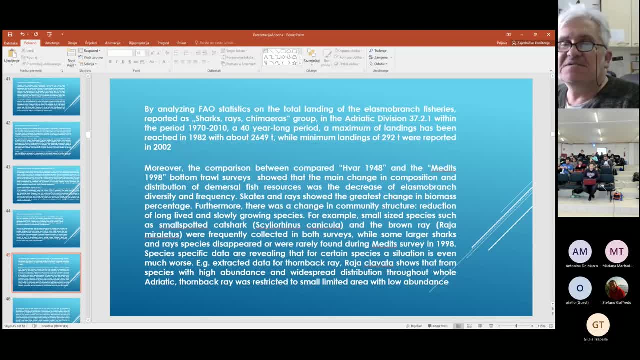 And practically represents the virgin situation of stocks in the Adriatic according to the Mars resources and the another one on which base this report, which I mentioned the recent state of the Mars resources in the Adriatic Sea and called the Medici 1998, and the bottom. 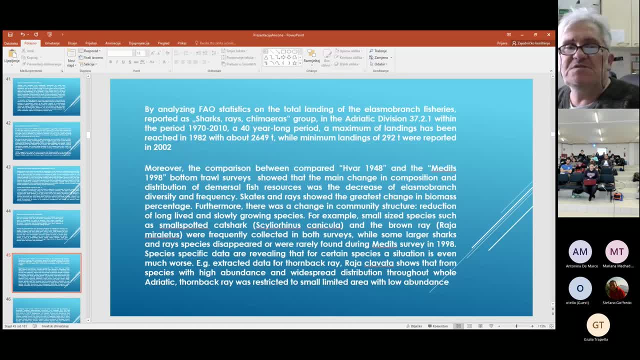 draw service Showed that the main change in composition and distribution of the Mars and fishery sources was the decrease of Elas-Mobrang diversity and frequency. Which parts of Elas-Mobrang show those great, great change in biomass, the skates and rays? 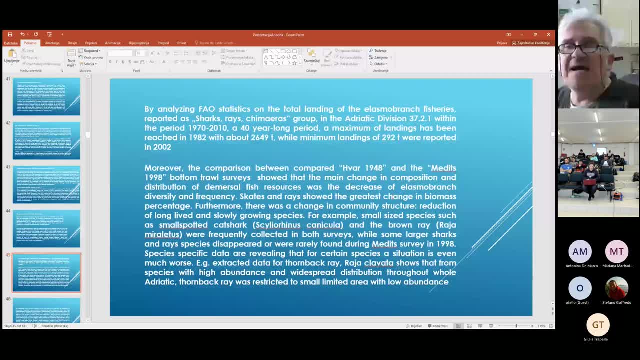 So practically those two groups show the greatest change in biomass percentage. Furthermore, there was a change in community structure: reduction of long lived and slowly growing species. For example, small sized species such as such as small spotted cat sharks and the brown ray were frequently collected in both surveys, while some larger sharks and race species. 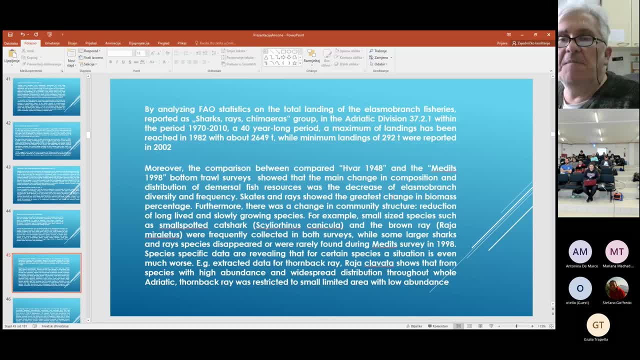 disappeared over a rarely-funded period of time, And this was a significant change in population structure. Furthermore, there was a change in community structure And this was a significant change in population structure. They are因 разы хcalled species with high evidence and widespread distributions throughout the whole area. 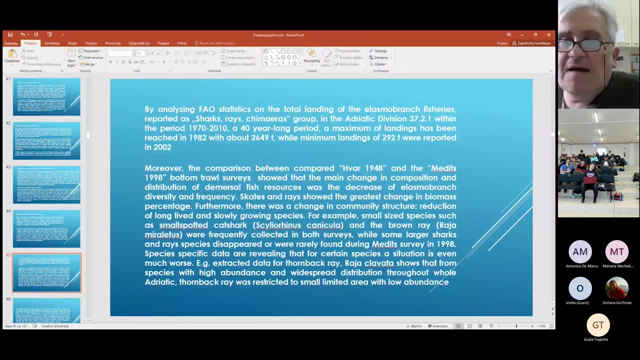 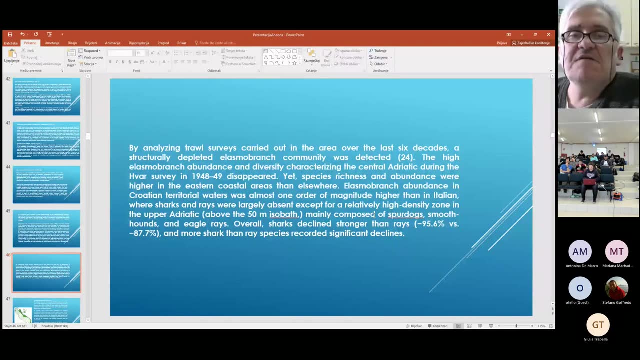 the whole Adriatic. Tornback ray Raya clavata was now restricted to small, limited area with low, low evidence. If we try to analyze troll surveys carried out in the area over the last six decades, the structurally depleted Elasmobranchs community was detected. 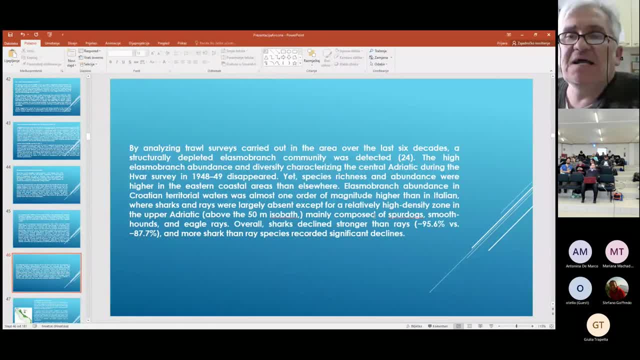 The high Elasmobranch evidence and diversity characterizing the central Adriatic during the Hvar survey in 1984-1949 disappeared Practically. species richness and evidence were higher in the area Eastern coastal areas than elsewhere. Elasmobranch evidence in Croatian territorial waters was almost one order of magnitude higher than in Italy. 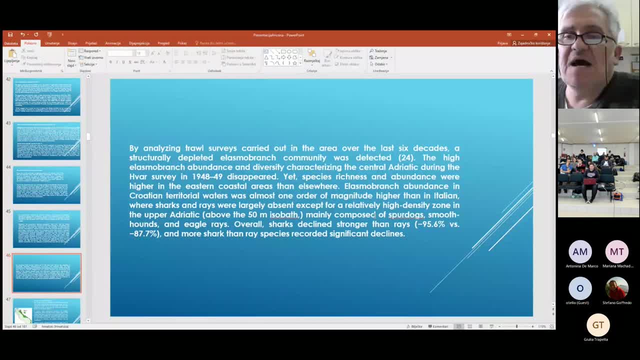 The sharks and rays were largely absent, except for a relatively high density zone. in the upper part of the Adriatic, about 50 meters is about mainly composed of spur dogs, smooth house and eagle rays. Overall, sharks declined stronger than rays And more sharks. 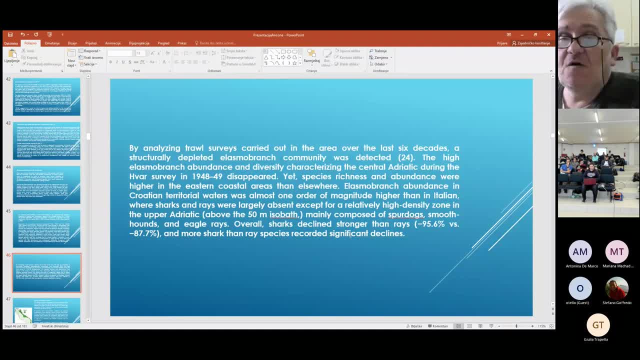 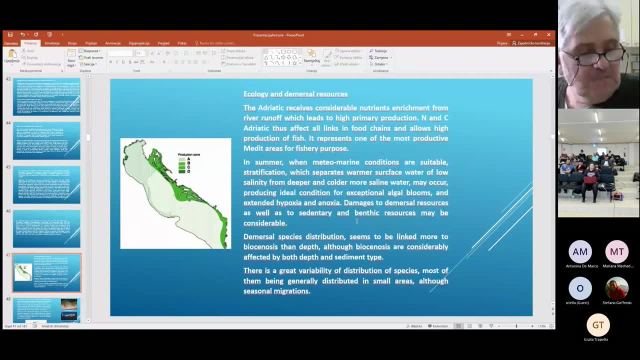 Then race species recorded significant, recorded significant declines. OK, The few words about the ecology and the nursery sources. The Adriatic: the Adriatic receives considerable nutrients enrichment from the river runoff which leads to high primary production. The northern and central Adriatic does affect all all links in food chains and allows high production of fish. 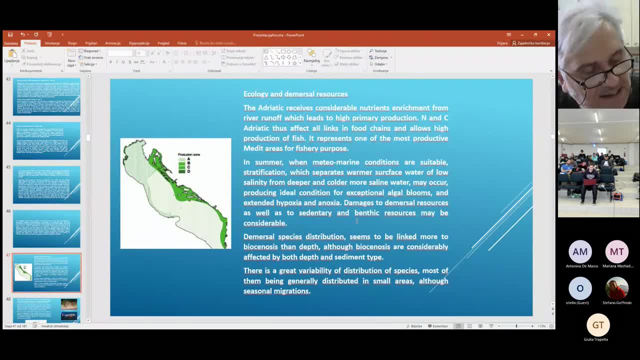 As a matter of fact, the Adriatic Sea represents one of the most productive Mediterranean areas for fishery purpose In summer. During summer, when metamarine conditions are suitable- for example high temperatures, extended period of calm sea, fresh water inflow, inflow stratification- 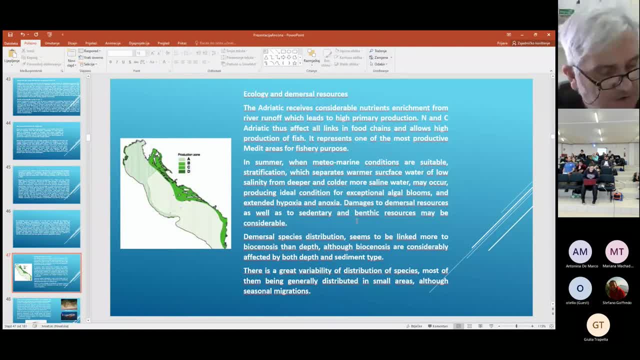 Suitable stratification which separates warmer surface water of low salinity from deeper and colder, more saline water may occur, producing either condition For exceptional algal blooms and extended hypoxia and anoxia. Damages to the mercer resources, as well as to the sedentary and benthic resources, may be considerable. The mercer, species distributions seems to be linked more to biosynosis than depth, although biosynosis are considerably affected by both depth and sediment type. There is a great variability of distribution Of species, most of them being generally distributed in small areas. Although seasonal migrations, Many of the species complete their biological cycle throughout, Throughout of the whole basin, with the reproduction area localized along the Italian side, For example to Gurnard, common catfish or Croatian coast, For example solar, The cruids of many species aggregate along western coast in summer. 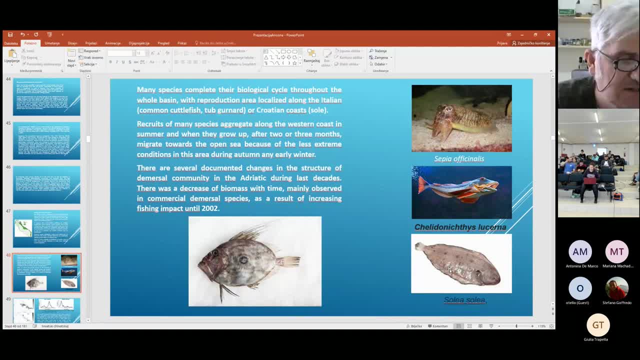 And, when they grow up, After two or three months, migrate towards the open sea because of the less extreme conditions in this area during autumn and early, early winter. On the other hand, there are several documented changes in the structure Of the mercer community in the Adriatic during last decades. 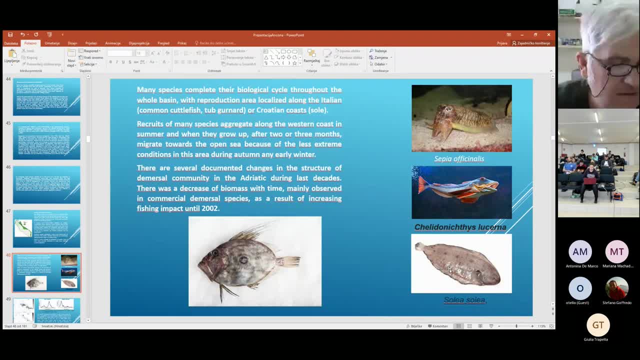 There was a decrease of biomass With time, mainly observed in commercial demand species as a result of increasing fishing impact until 2002.. Moreover, from the comparison of the two trove survey carried out in 1948 and in 1998, the decrease of Elasmo branch importance, diversity and occurrence was observed. 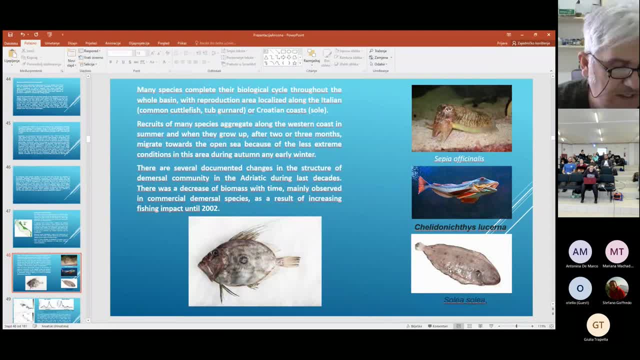 Some boni fish replaced Elasmo branch at the top of the catches. However, some differences were found in the relative occurrence and evidence by Elasmo branch species. Small sized species such as Celerin huscanicola, small spotted cat shark and the brown array Raya miralatus were frequently collected, while other species. 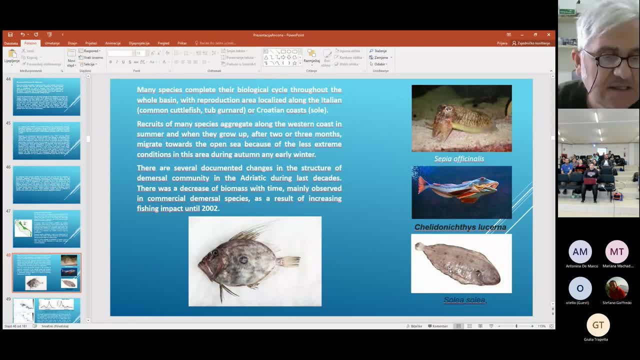 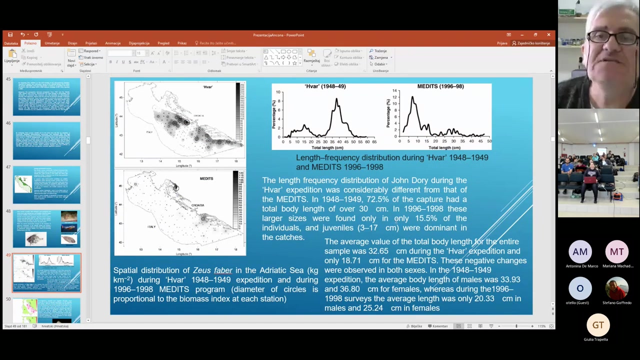 Bigger shark species, for example, And other species Disappear or rarely found. Life history parameters of the species could explain the different reaction of Elasmo branch to to fishery. Okay, You can see here The length, frequency Distribution. 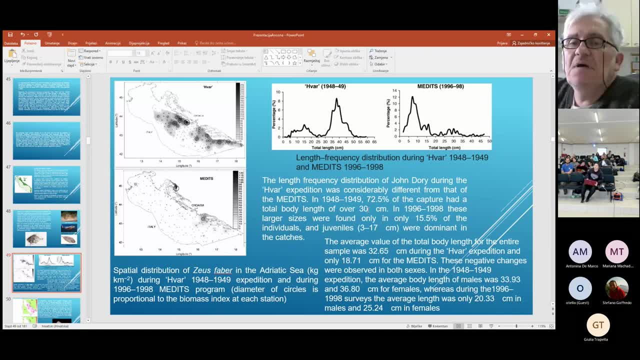 During Quar expedition And the meditz For John Dory. It is Zeus Zeus Faber, for example, And During the Quar expedition The distribution was considerably different From that of the meditz In during Quar expedition. 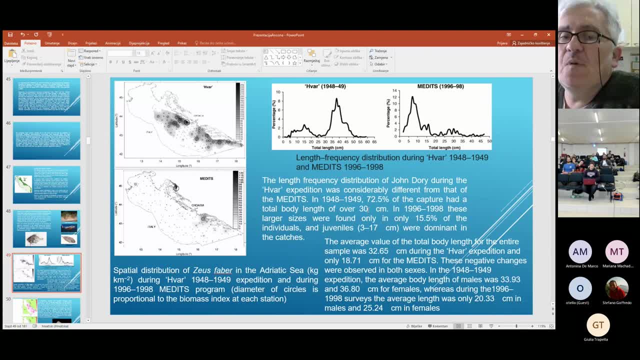 72.5% Percent of the capture had a total body length of over 30 centimeters In 1996, 1998.. These larger size were found only in 15.5% of the individuals And juveniles. Where From three to 17 centimeters were dominant in the cages. The average Value of the total body length for the entire sample was 32.7065.. Sorry Centimeters during the Quar expeditions And only 18.71 centimeter for the meditz. 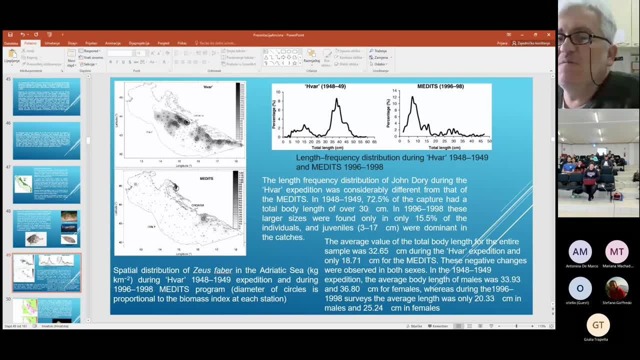 These negative changes were observed in both sexes And In 40. 19.. During the Quar expedition, The average body length of males was 33.93. And 36.84 females, Whereas during the 1996 and 1998 surveys. 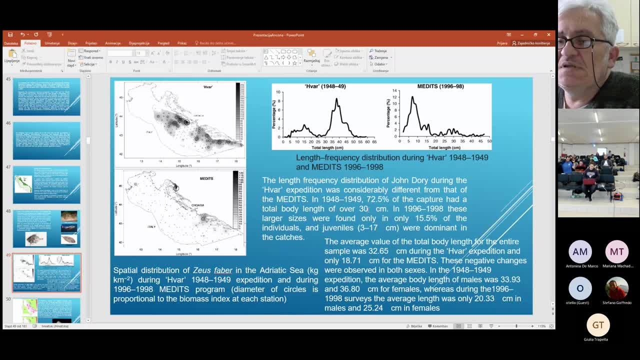 The average length was only 20.33 centimeter And For males and 25.24. Centimeters in females. So you can see here The drastic, Drastic decrease In Length. frequency distribution In Special distribution. 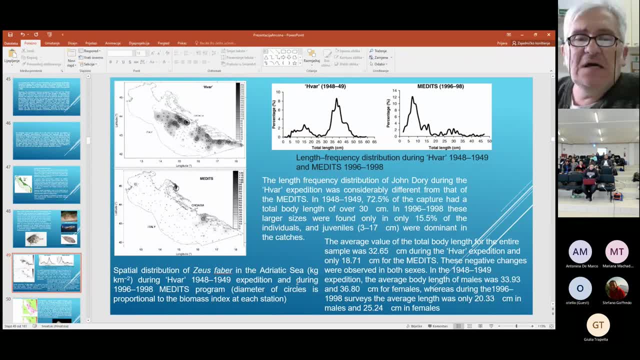 And And And Biomass index at each stations. You can see here During the Quar expedition, Special distribution With points And you see now So much reduced, So much reduced. Special distribution, And And And. 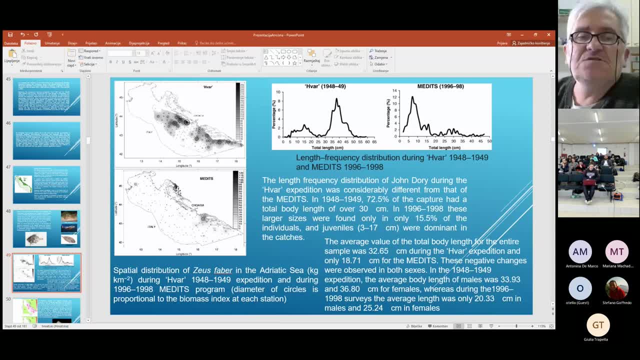 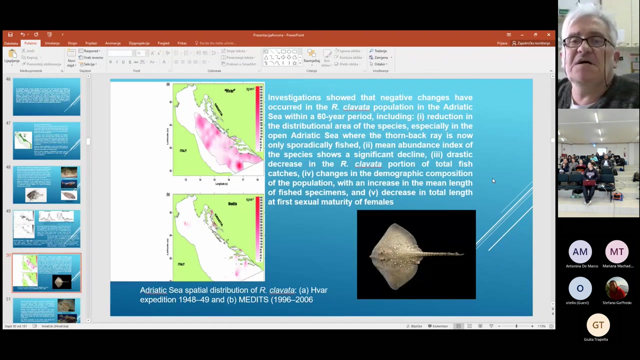 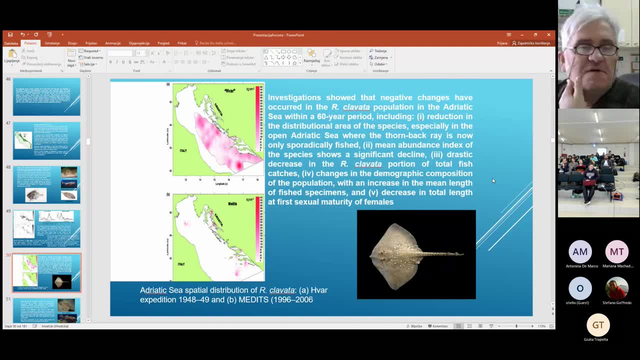 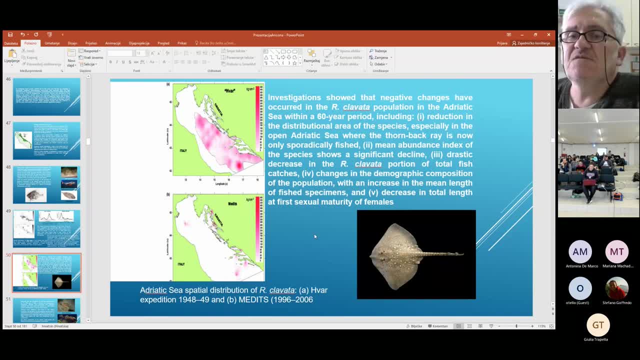 and including also mean evidence index of the species, which shows a significant decline and thus drastic decrease in rata-vata portion of the total catches. Also, it was observed now huge changes in the demographic composition of the population, with an increase of the mean length of fish specimens and decrease in total length at first. sexual maturity of females. 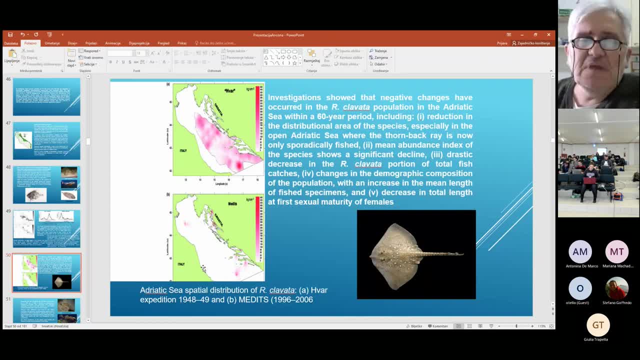 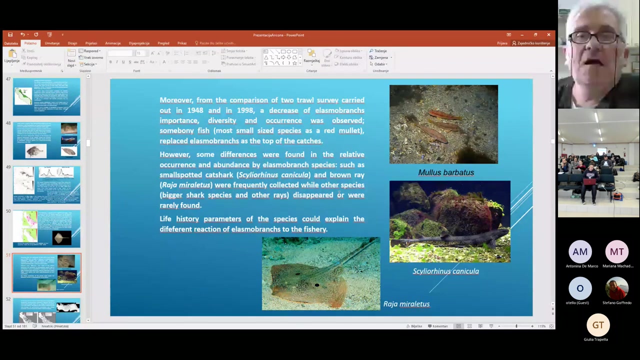 You can see here on this picture according to special distribution of rayacravata during the Juar practically virgin stock expedition in 1948 and 1949 and medits during this period of 1996-2006. You can see completely reduction of the special distribution of, for example, of rayacravata. 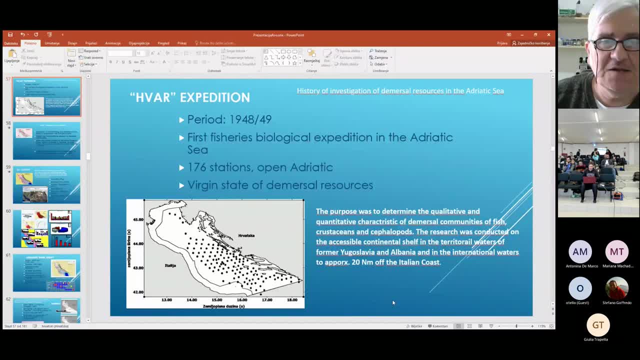 OK, I, somehow, I, I, I read you, You used some things And now I would like to say a few words about the, let's say, history, some kind of history of investigation of the Merza resources in the Adriatic. 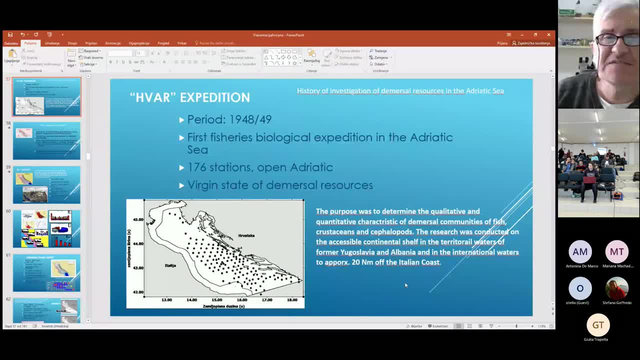 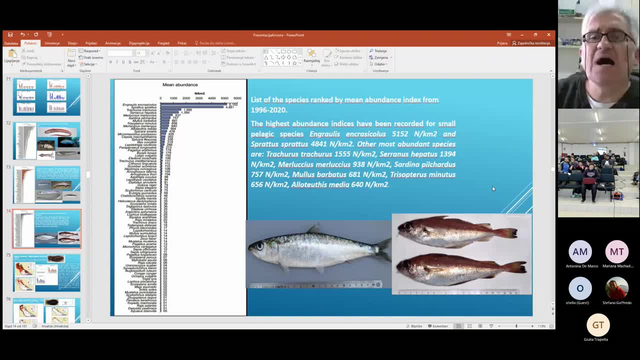 So it is sometimes very good to know what kind of expeditions and type of investigation you know And the highest evidence indices have been recorded for. again for the pelagic, small pelagic species and grauris and crassicholus and the spratus bradus. 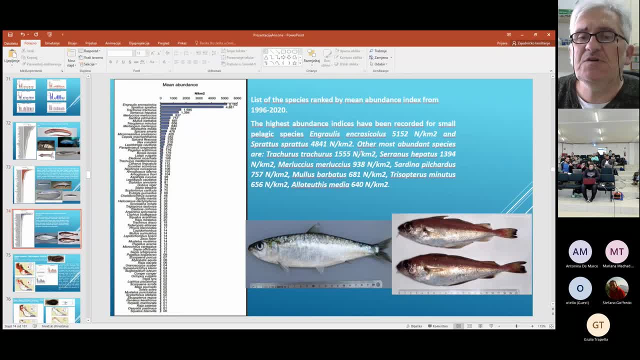 And another species. another most evident species are trachurus trachurus serranus, hepatus, merlutius, merlutius sardinia, pirhadus, mulus barbatus, trisopterus minutus and Alothéotis media. 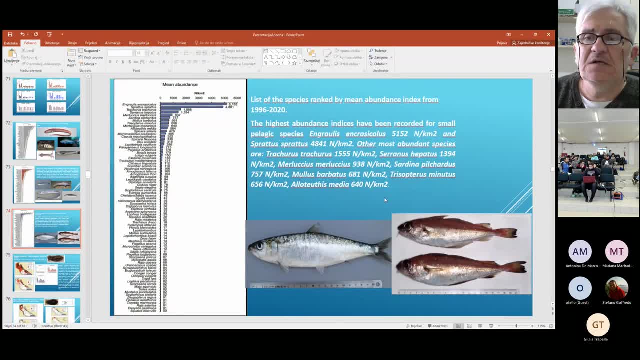 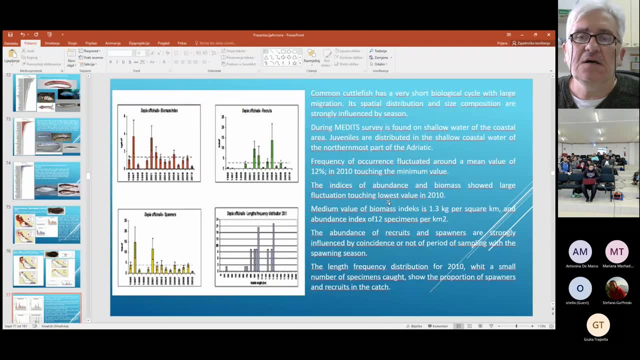 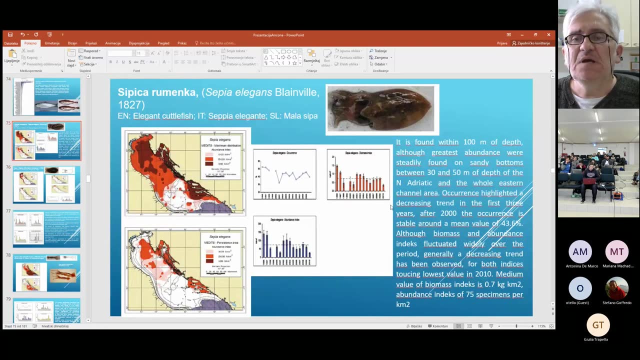 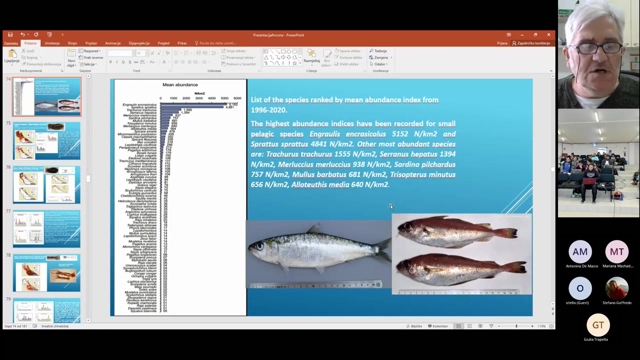 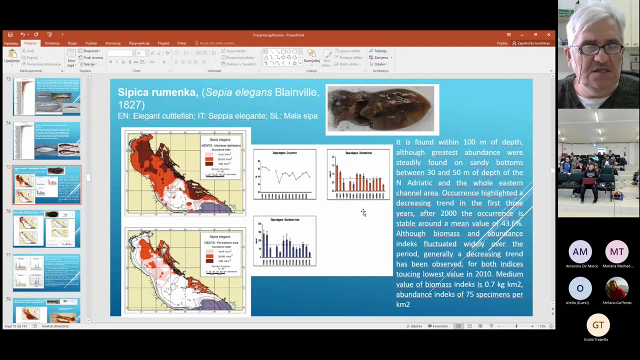 And I will show you example: what you can find in results. Practically, those are the results for each species which are included in this book. So practically, I will show you example And so practically, it is divided in the parts. 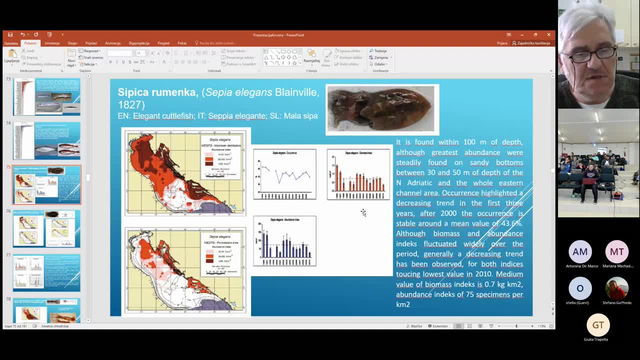 for example, cephalopoda. Then you have fishes and then crabs, for example, And it is all divided and results are looking like this. I will show you for some species, just to introduce you, if you want to. 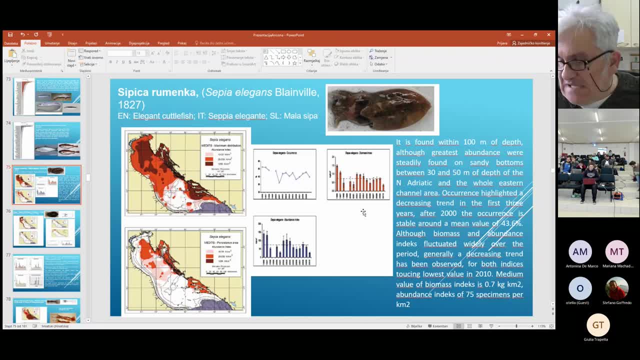 In detail, if your maybe. subject will be in the future the Mercer resources. So why not to see in this kind of a book some kind of monography? practically You can see how the results are presented for each species according to the types of presentation for this Medici book. 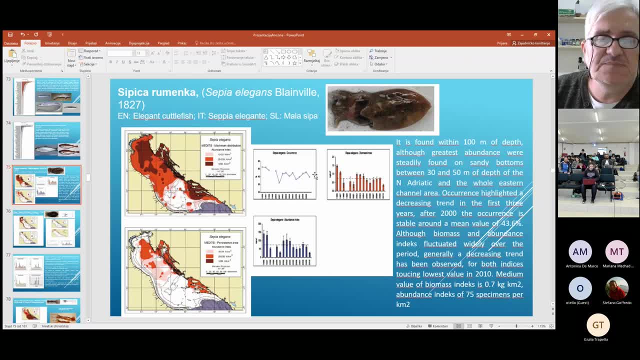 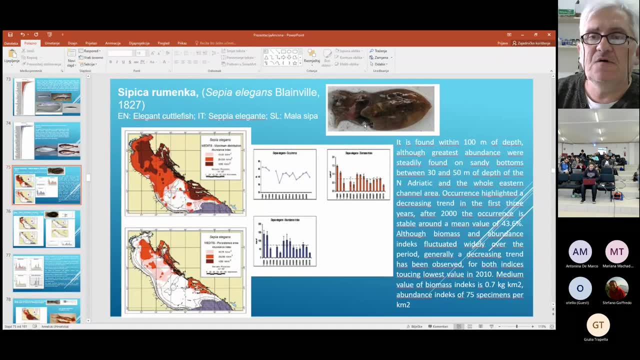 It's a project or Medici expedition, So it is presented by the photo and of species. This is in sepia elegans and the name of the in English, Italian and Slovenian, And this is the title is in Croatian. 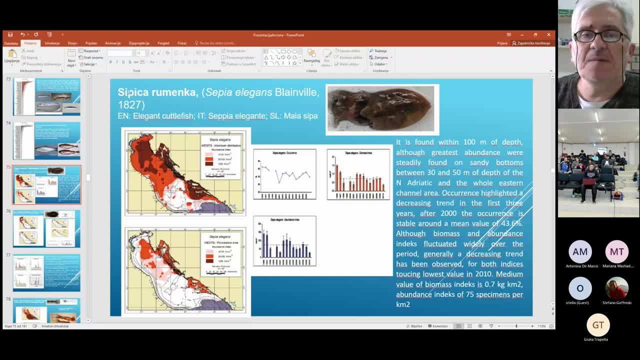 So practically you have here an example for the sepia elegans. It is elegant cuttlefish. sepia elegante in Slovenian mala sipa in Croatian sipica romeka. So you have data about the maximum distribution. 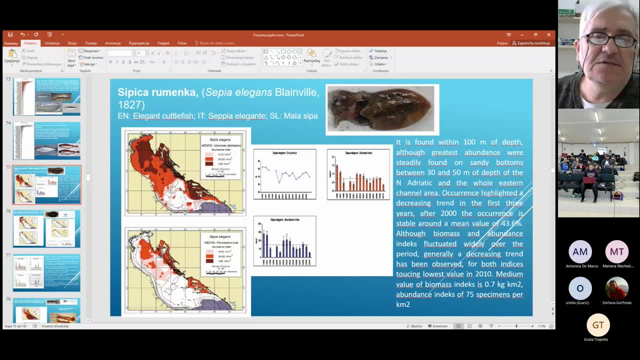 You see here, for example, this red color showing distribution of the sepia elegans. You see here, for example, this red color showing distribution of the sepia elegans of this species, with the with the number of of the specimens, practically evidence index. 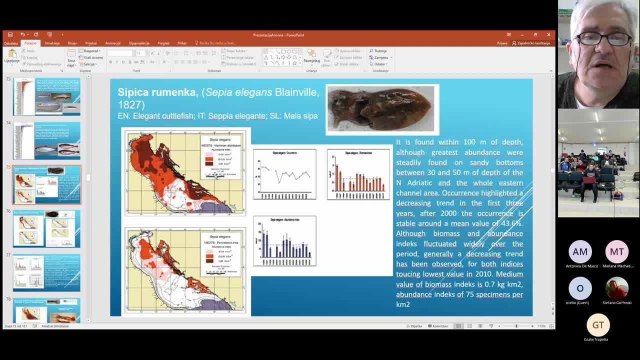 for each. this is a part, for example, where it is the most evident- see here- and then you have a persistence area evidence index, also of sepia, and then diagrams, that where you can see data about the biomass index, about the, the evidence index, and for example, it is this type of. 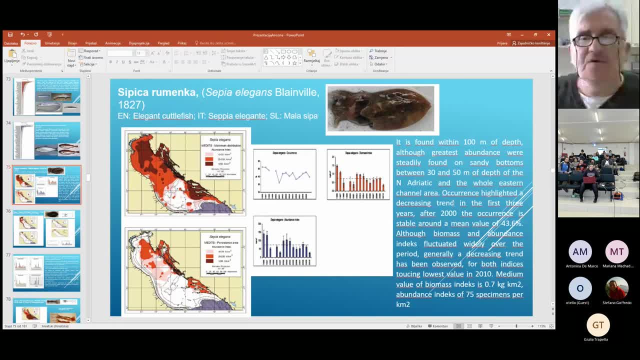 of species is is, for example, a few words are written about each each species. for example, it is found within 100 meter of depth, although greatest evidence were steadily found on sandy bottoms between the bottom of the sepia and the bottom of the sepia and the bottom of the sepia. 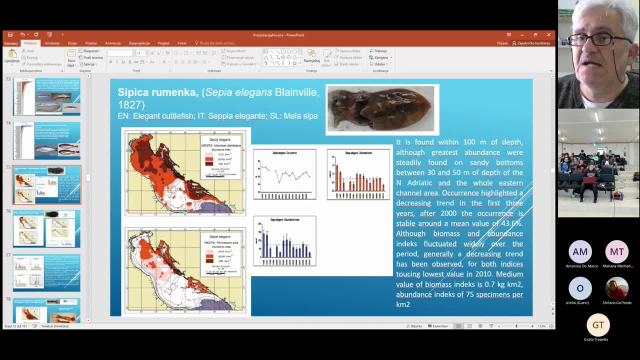 in 30 and 50 meter of depth in the north part of the adiatic and the whole eastern channel area. occurrence highlighted the decreasing trend in the first three years after 2000. the occurrence is stable around the mean value of 43.6 percent, although biomass and evidence index fluctuated. 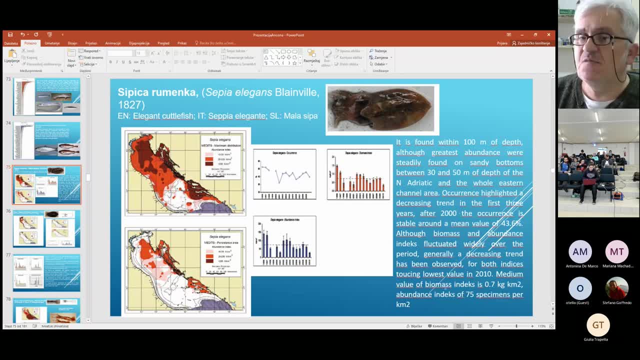 widely over the period. generally the grazing trend has been observed for both indices, touching the lowest value in 2000 and 10. and you have here the data about the median value: of biomass indexes was 0.7 kilo per kilometer square and evidence index was 75 specimens per kilometer square. so practically you. 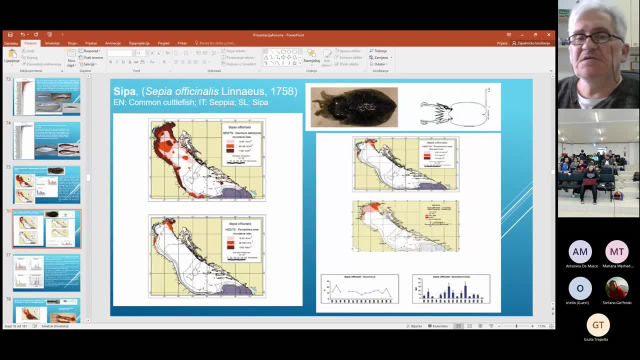 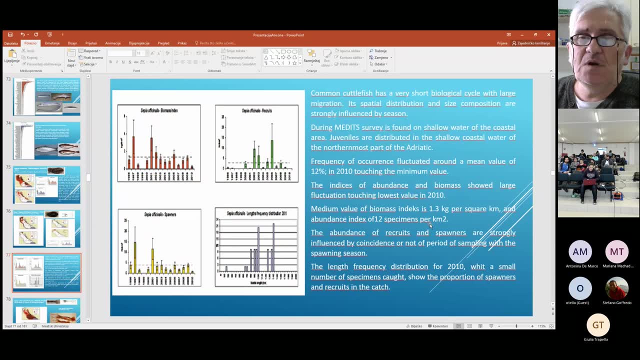 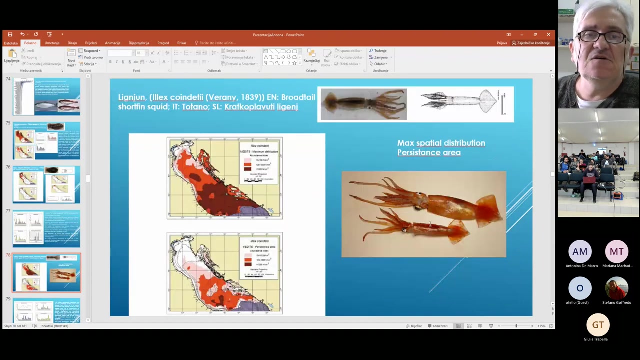 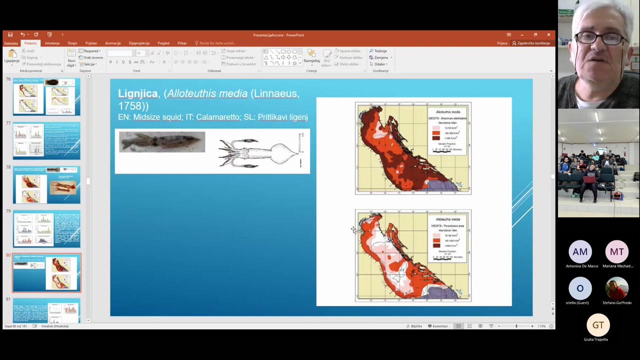 have another very important species, sepia, of its analysis. again, the procedure is the same, and a few words about the biomass index, uh, the indices of evidence and biomass about the fluctuation, length, frequency, distribution, and another is ilex coindetti, etc. etc. i would not uh losing time, practically when you have this in. 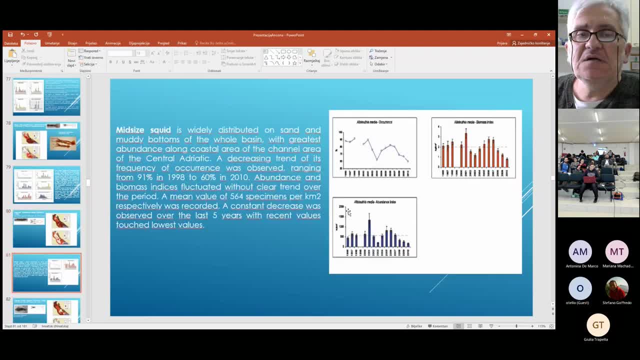 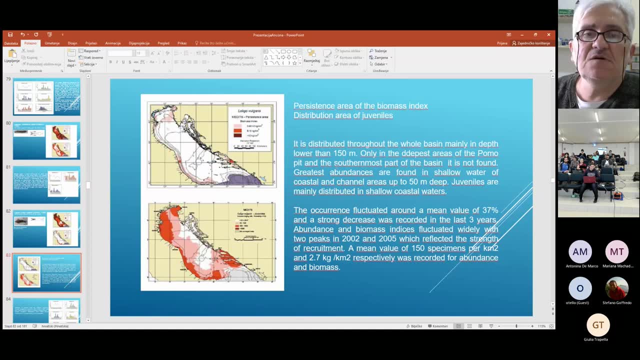 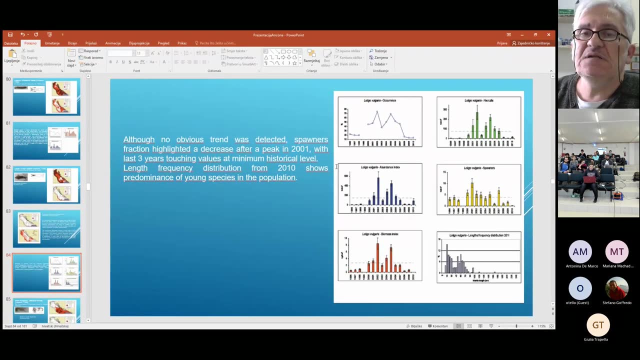 this book. so i just try to show you uh the procedure, uh how is uh written? you have here, for example, distribution area of juveniles for oligo vulgaris. i think that it is connected also with the, the most important species which were in the catches in. 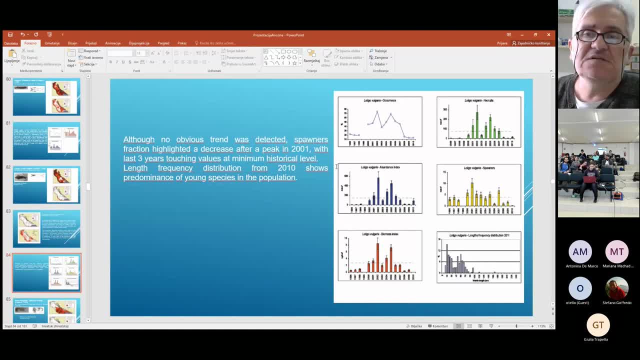 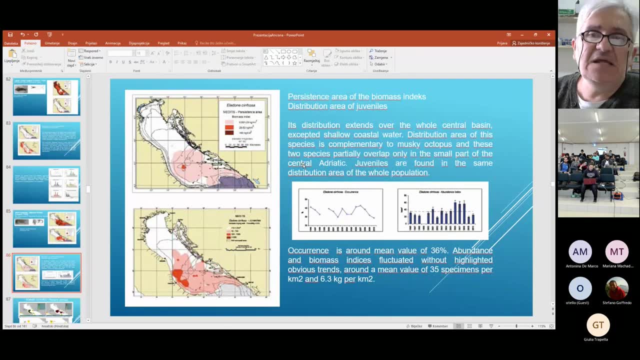 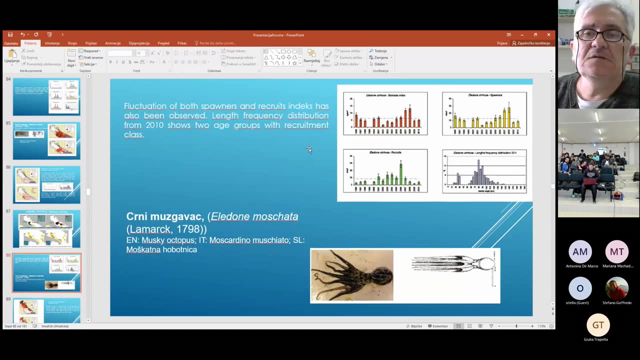 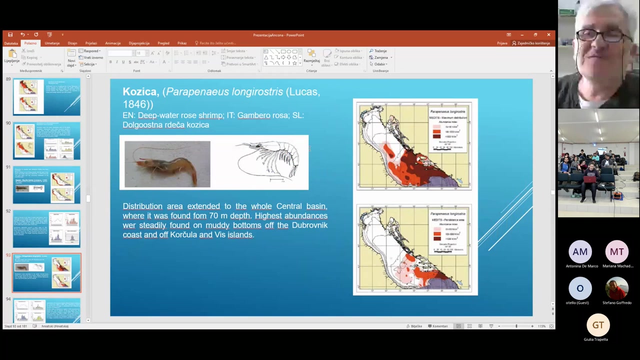 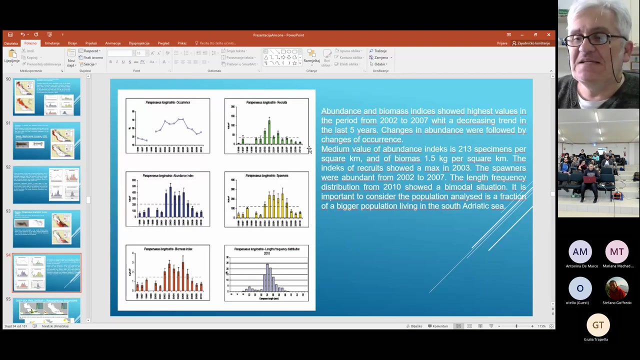 in troll, troll, catches and uh, according to the manager, resources which were most important for the adriatic. and you have all the data, let's say very recent data, according to, to, to the importance, uh, so i, i, i really don't want to um, squeeze students with this- uh, all these data. so who wants to get more info? i think that it will be, he will. 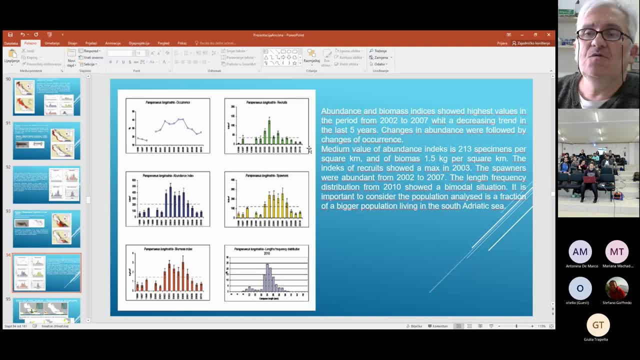 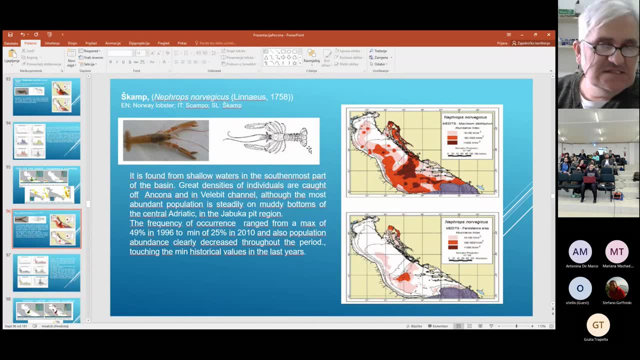 be a or she will be able to to to to see this uh in in this book. uh, i will send all necessary uh information for the students to to to stefano and he will get all the data about about the most important uh literature which is important for the students. all necessary data. 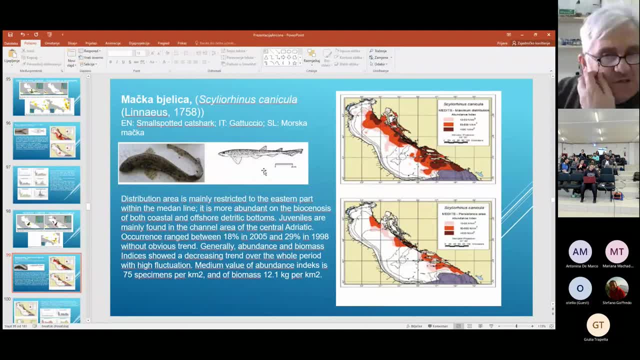 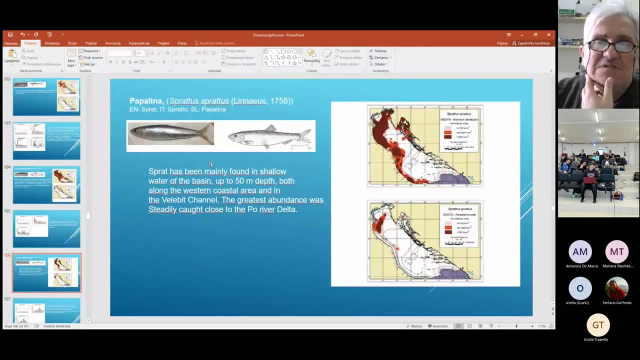 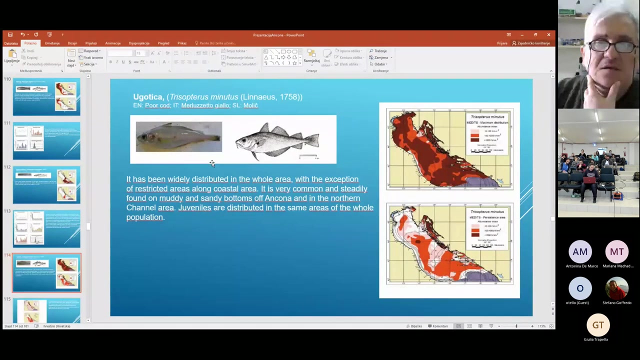 I will send the presentation. So who will need it and who will try to be much more inside could ask Stefano for this presentation in general, but I said that it is mostly connected with this book, which I will send again. new info about this book. 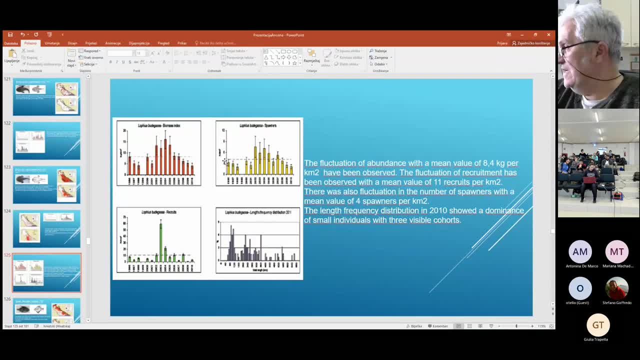 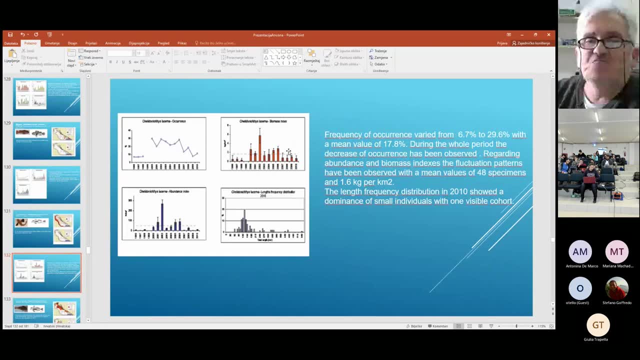 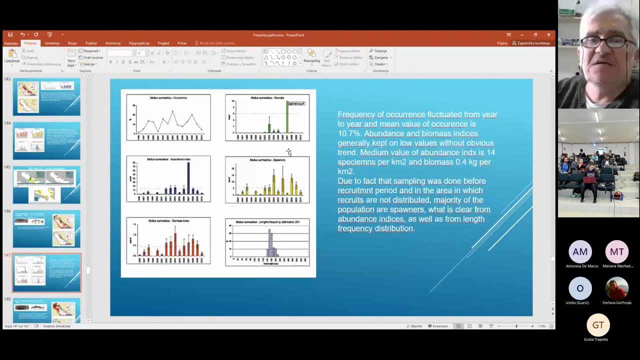 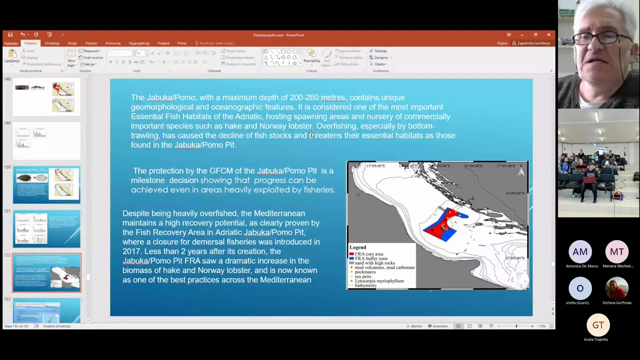 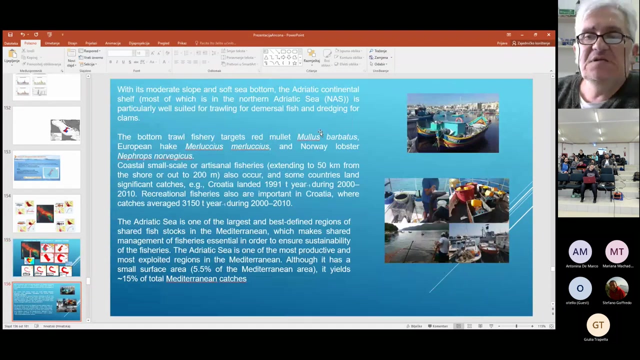 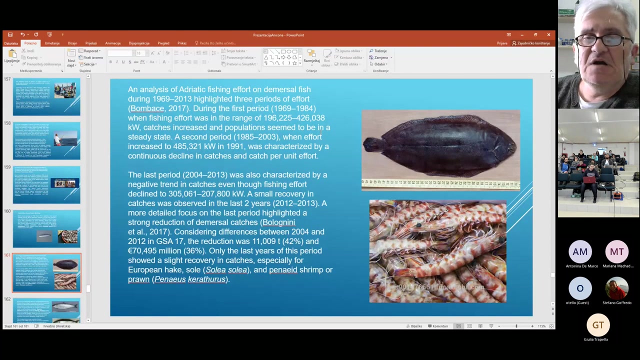 So, practically, I would like to, in general, to finish this presentation, I could only ask you, if you are interested, to show me all with, let's say, more info about this, new data about the changes in ichthyofauna which are connected with the processes I already said. 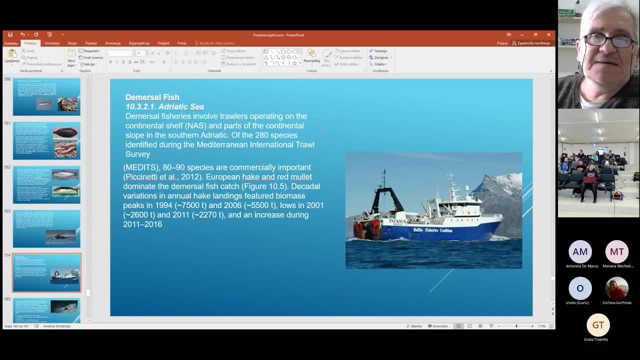 with meridionalization, tropicalization, with the Lessepsian migration. Yeah, I was the member of the team CSM center. This is the center of this commission for the Mediterranean Sea. He's in Monaco and president And I think the main director of this institution is Frederic Briand. 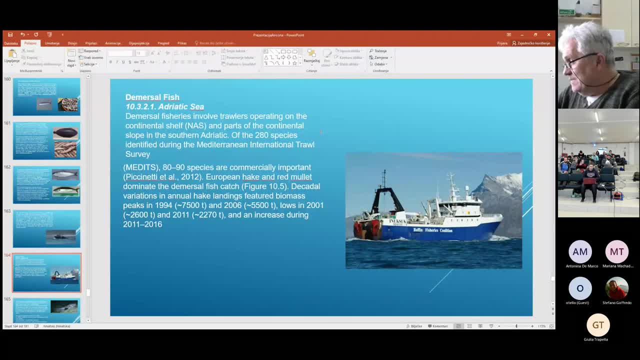 And in general the boss is Prince Albert, who is the main chief, even though Frederic Briand is the boss of the station in Monaco, And we prepared a very interesting atlas of new species, And this is the second edition for the Mediterranean Sea. 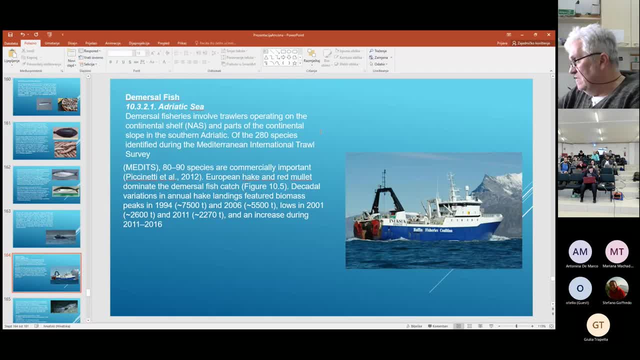 including all the changes which happened, which happened with start from the opening of the Suez Channel until today. So, practically if someone is interested in such type of info or to see the book, I think that it is possible to find it in Fano. 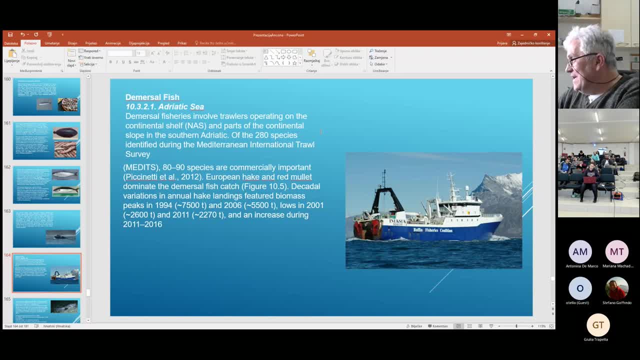 I for sure know that who bought it? because one of the authors, as like as me, was Ernesto Azzurro, my great friend, which was, I think, now working, I think, in Ancona. I'm not so sure, but previously he worked in Livorno, I think. 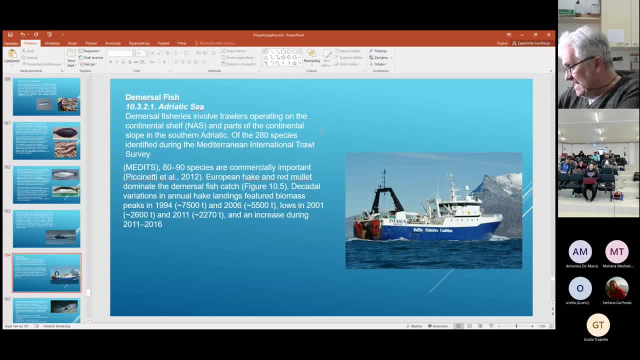 And we prepared such a nice atlas And with all the new data about the new elements of the Mediterranean. OK, at this moment I will finish. I hope that I know that sometimes it is boring to hear all these numerical data. I try to escape all these graphs etc. 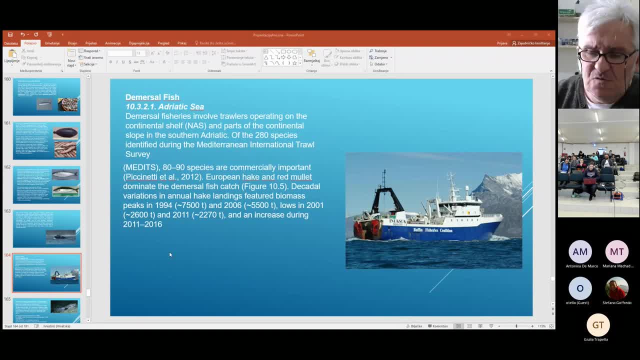 And try to, by voice, to present you, Because sometimes you are able to much more concentrate on the pictures and you are losing the voice. I think that the voice is very important And what you need to remember it. You need to remember it. 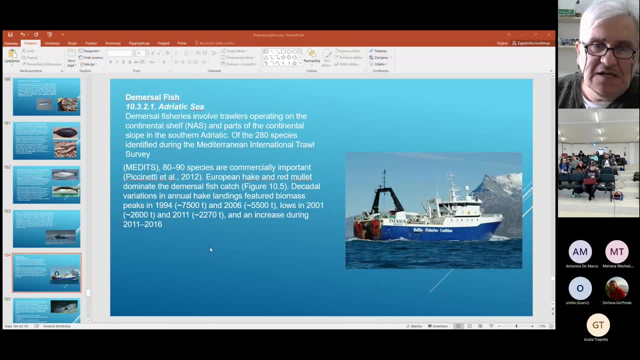 The difference in troll catches between southern and the north, central and the northern part. You see, you must remember what are the main target species in means of pelagic resources, in means of the mercer resources, What are the differences between types of fishing gear? from practically, 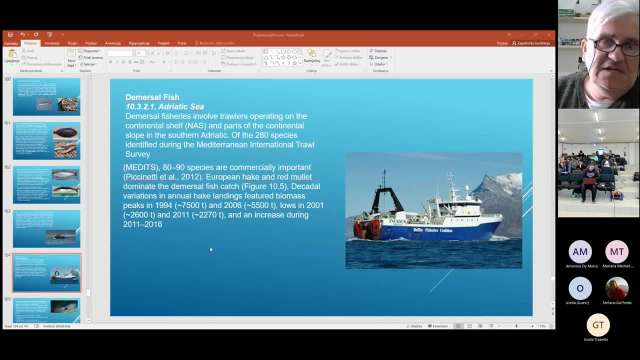 from Croatia and from Italy. These two countries are, in general, the dividing the resources of of of Adriatic Sea. So if you have any question, whatever And remark- I would like to know much more- Please send it to my email address. 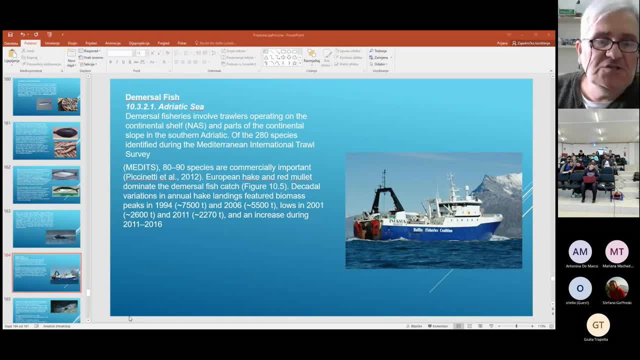 I think that Stefano will give it to you. Then I will be in contact with Stefano And I will send him all these presentations And even though, if you want, I will publish papers in the most respectable journals which are connected with general Adriatic fauna. 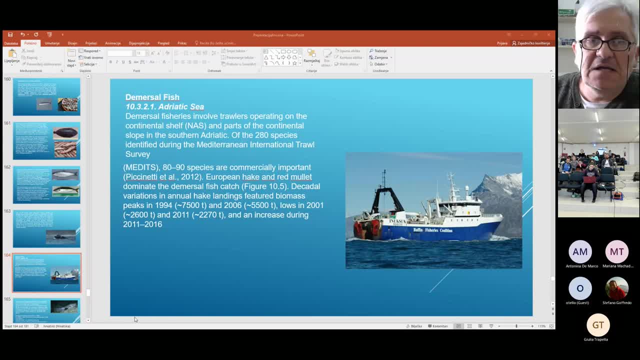 I will be glad to send to you if you are interested. And not just Adriatic. We published also a nice paper where we check all the record with fish species for the Mediterranean Sea. That was all from me. Thank you for your attention. 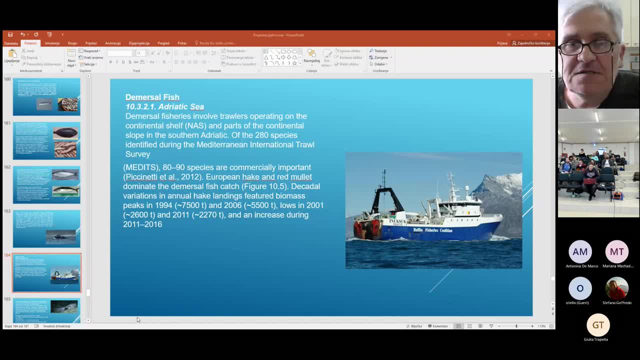 And thank you for your patience to heard my boring voice. Thank you, Jakob. Thank you very much for the broad view on fishery problem in the Med, in the Adriatic, And I guess there may be some question. but I would like to start with my question. 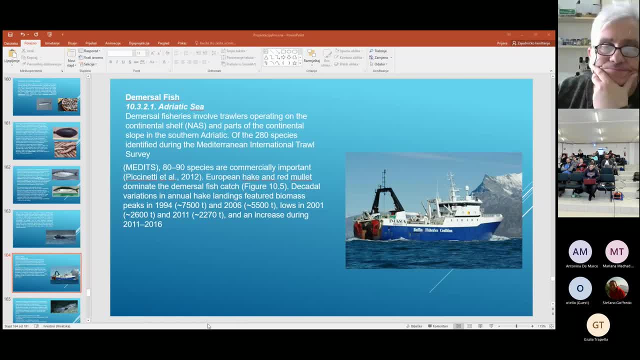 I would like to take over the students, But I have two questions. The first one is about the large oscillation in biomass that you show, for example sardinas or anchovies. There's a kind of order of magnitude among the top and down. 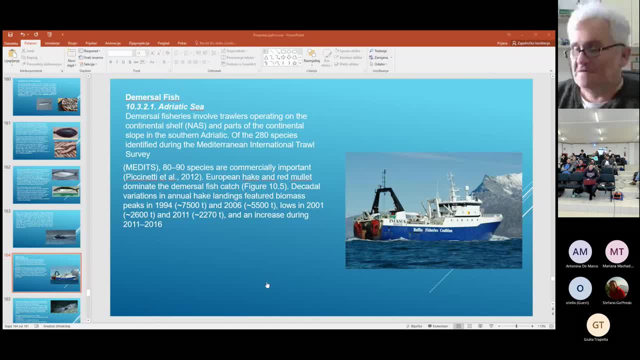 up and down. So are these? What is your explanation? Are these natural fluctuations or there's something else? That's the first question. The second one, on my premise that I'm not an expert in this field, of course you know already everyone. 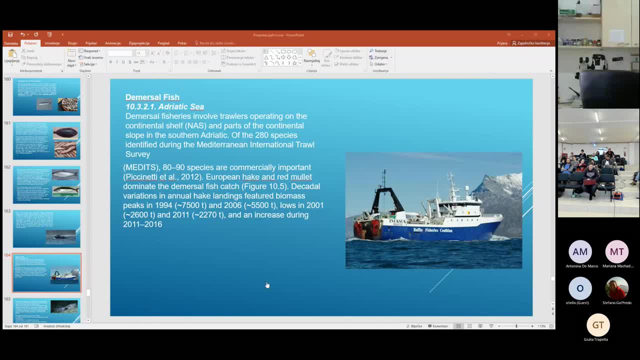 The second one is: are all these data from this survey, for example the one that you show that are in this book that actually is available in this institute we have here- are somehow now also digitalized? I mean, are public people can download the raw data I'm talking about? 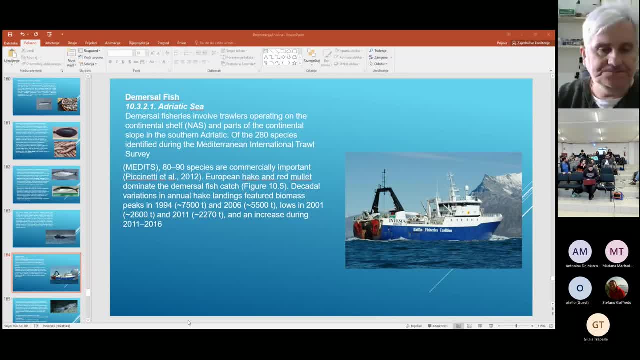 and make statistics and elaboration. Thank you, Those are the two questions. OK, First, I will try to answer it on the OK First. I will try to answer it on the second because it is published by. I'm not sure it is available. 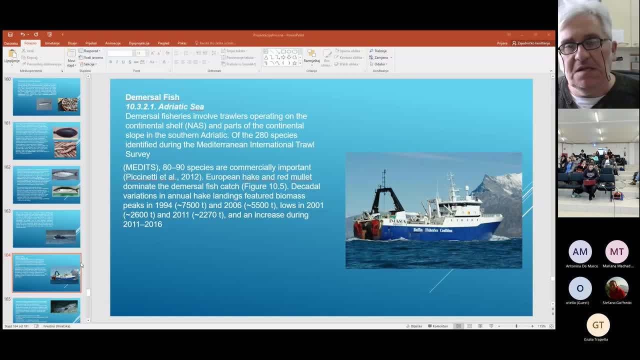 but I hope that it is available in FAN, or even though you might call it. This book was for sure, published and the main author was Corrado Piccinetto, So practically I'm sure that this type of book was available at the library of laboratory in Fano. 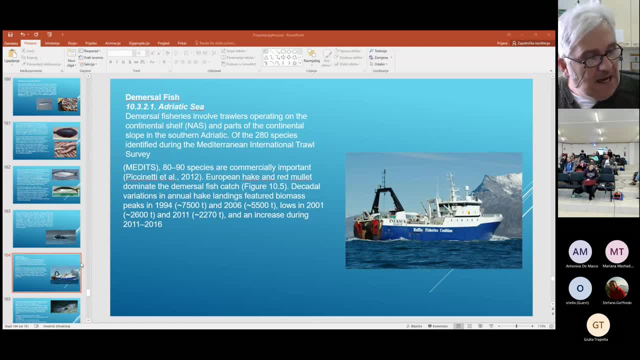 and also in laboratory of Angola. for sure, I will send you. This is the monograph series number five, published in 2012,, and it has 220 pages. So this is, I think, available. If it's not, I will send it to my library department. 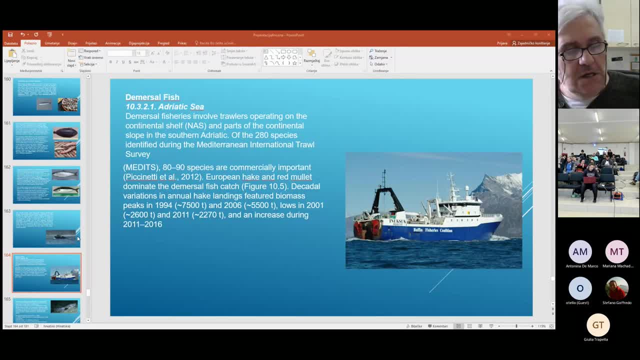 to send it to you. I think that there is, I think 100 copies are available in the institute of this book and I hope that it will be available for the students, for sure, because the main author is Corrado Piccinetto. 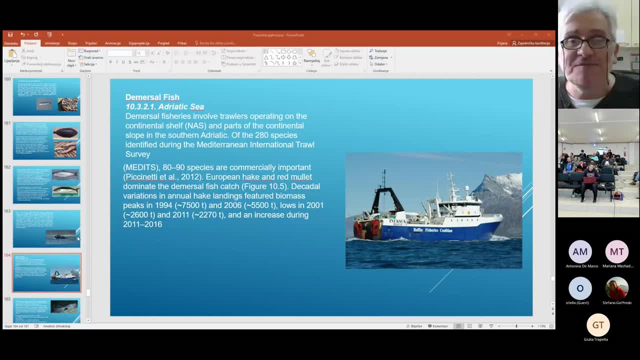 Yes, That is the reason, And another one is Chiara Manfredi, and two other ones are Nedo Vrgocevic, who was the director of the institute in Split, and Juan Marchetta is from the institute in Slovenia and Ljubljana. 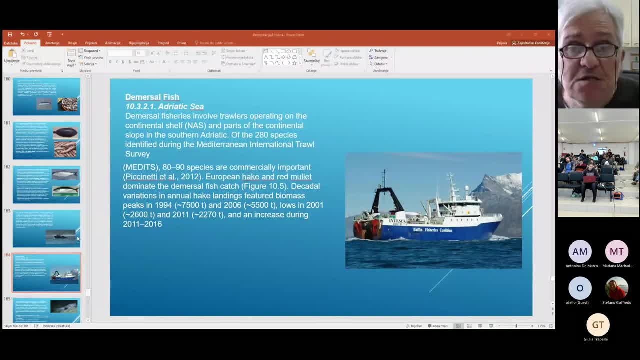 So for sure, this will be available. If not, please you need to tell me and I will send copies, or let's say hard copy for you to be available to the students and you, of course. And the fourth one was connected. 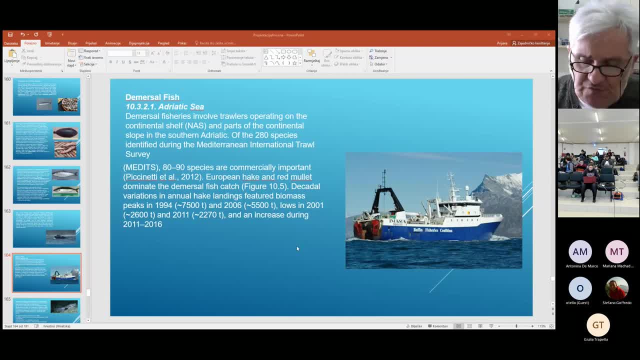 with the huge fluctuations of small pelagic. When I started, I will always go back to the history. When I started to work, I was in the department for, and my boss was the professor and he tried to learn me and to push me. 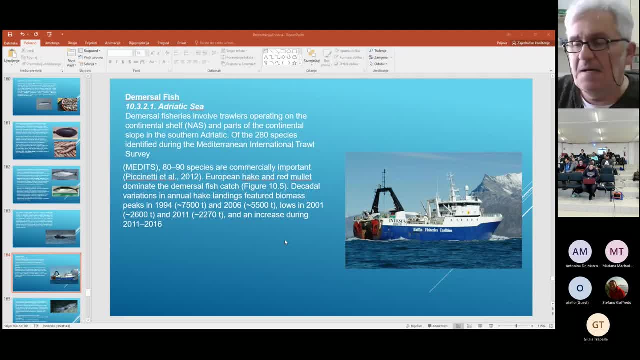 to think much more globally And if you see, in the past there was a huge In general, it was a huge discrepancies and huge fluctuations of small pelagics, including sardine and angio. I'm much more connected with the sardine. 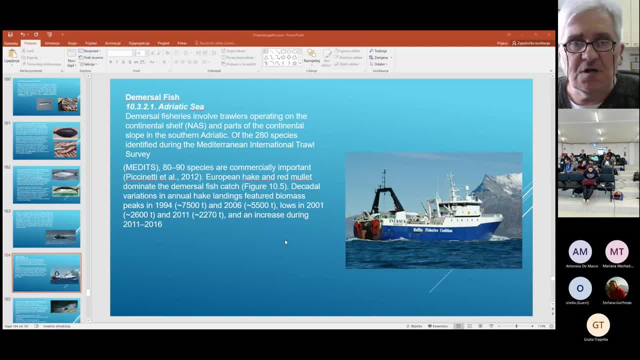 because my master degree thesis- not doctoral, but my master degree thesis- was connected with the sardine And I also tried to find how old are the sardine and tried to establish the old, How much is old in days, And I was in that time. 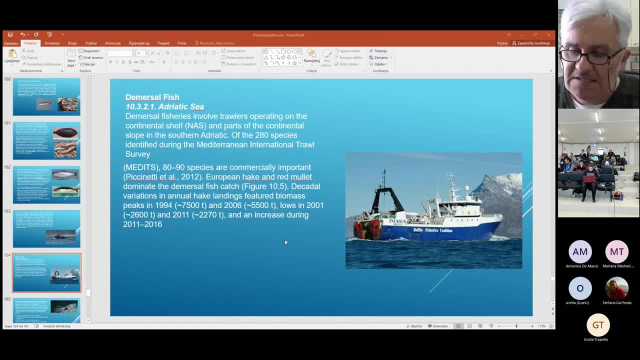 a young one and I worked on the field and tried to collect sardine And when I picked it, with a special constructed type of gear nearby, I lived in Castella Bay and I started to collect and I tried to collect. 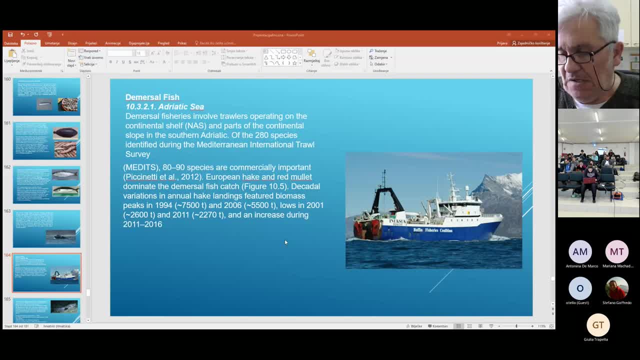 the larvae of the sardine, together with the otolith, which were too small And I need to use very special needles to extract such small otoliths from the larvae, And I tried to collect and to see how much old are such larvae. 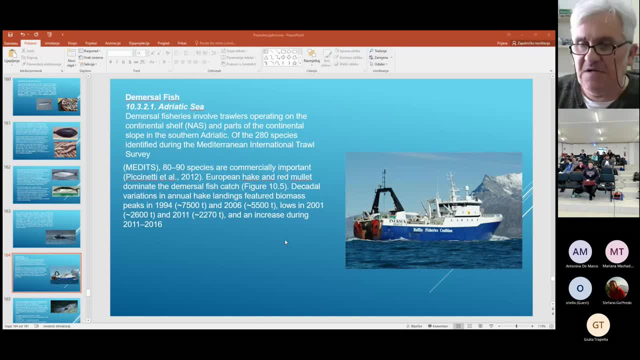 And when I get the data about the days- how much is old- I practically get everything. And in the history such fluctuations were observed in Dalmatia, in the part of Croatia where the capital is Split. My again father was also. 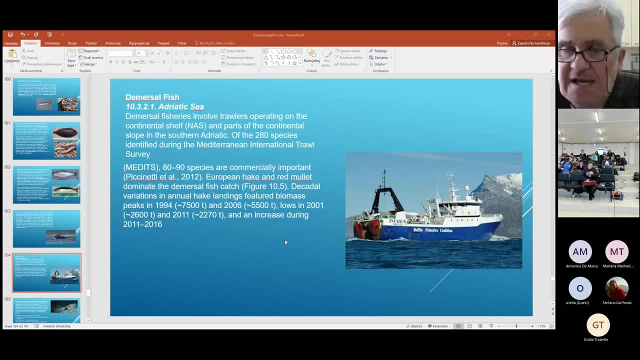 the fisherman and he tried to collect small pelagic again And there was a huge situations that in some kind of period in the 30s, in 30s, 1930, where, let's say, practically disappeared sardine. 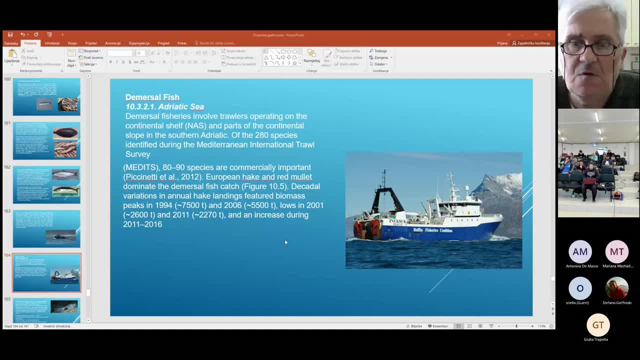 And that was the main catch of the people who lived near the sea, The men, especially on the islands. And in that time another species occurred, like some kind of replacement, was the sardinella aurica. This sardine, you know. 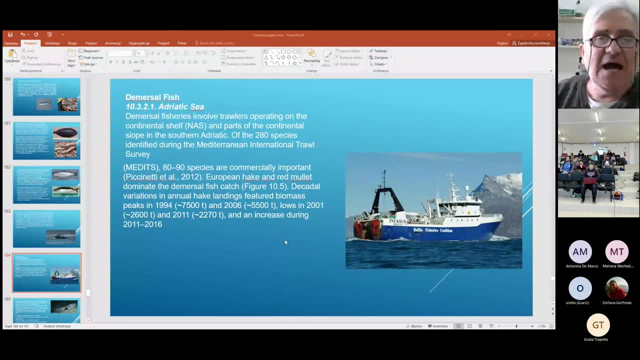 And there was a huge period of hungriness. because people were hungry. Why? Because there were not sardines And during that time it was also a disease in vineyards: Paranospera- Do you know what is Paranospera? 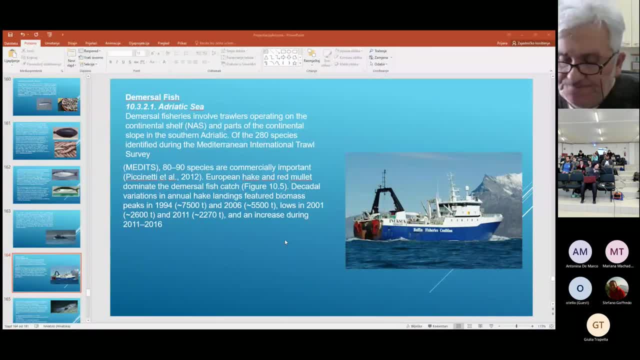 It was the kind of disease of flu And then practically people, especially from the islands, were in period of Second World War it's coming And in that time a lot of people went out from Dalmatia and trying to go. 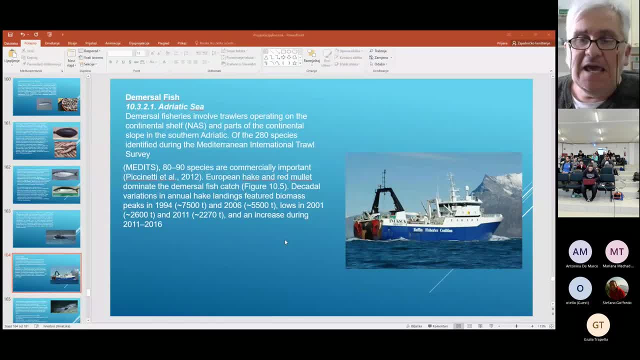 and find where is the sardine again. And they started. they went to Lampedusa, where it was. at that time it was the peak of the evidence of sardine And they started to catch, catch and it was a nice period. 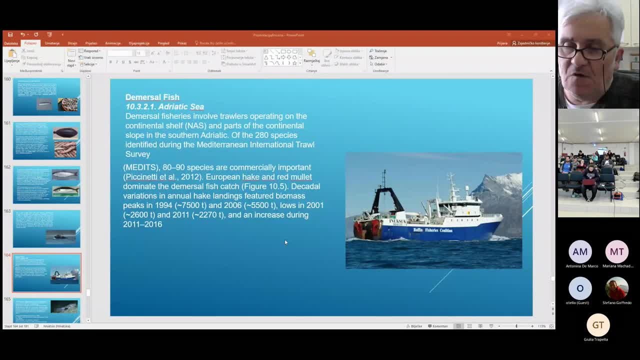 Then again, at the time of the that time, Lampedusa started sardinella to decline after four or five years And sardinella became again in the patches. So come back. And that was connected with a huge number. 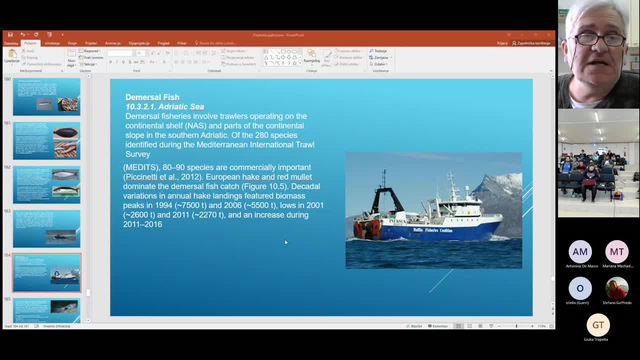 of parameters. I started to learn that the eruptions, the eruptions on the sun, could affect, could affect the biomass of small pelagics in all the oceans of the planet Earth. So practically environmental factors. all the evidence, and because small pelagics 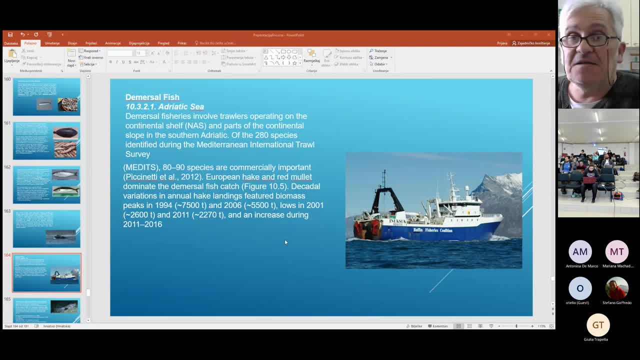 are exposed to huge fluctuations. I think my theory that it will never disappear means that you will never catch again, But fluctuations will happen according to some periods. But now Adriatic, the Mediterranean Sea, is exposed to huge impact of fishing gears And according to, 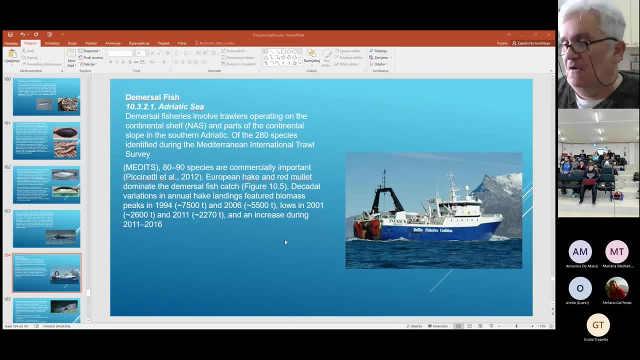 environmental factors which have changed according to, for example, what I say, eruptions on the sun. everything is mixed and everything could impact the evidence of small pelagics. So no fear in general, let's say No fear for the small pelagics. 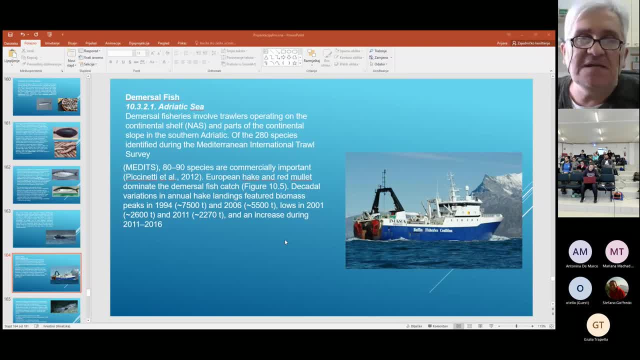 but how much will be available of biomass that will contribute? Okay, Here I explained in a way I'm not so good in, let's say, for this type of explanations. I'm not so good in English. to explain it much more precise: 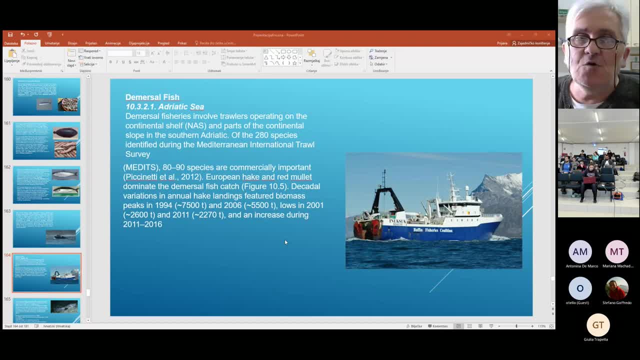 But in general it is much more a huge problem with the other resources because you know, for example, pelagic brands are has some kind of very low of reproduction. For example, two or three live specimens will be available per year, For example. 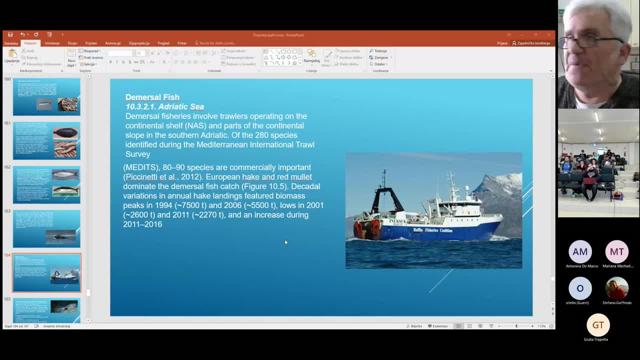 and the impact of the huge throes, especially from our side. I know it very well. the huge impact of the of the throes are enormous And this is the problem: Practically elastomer brands do not have time to recover the. 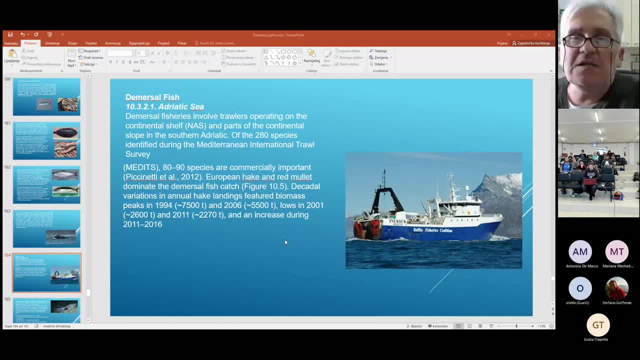 the, the, their population And, for me, man resources are much more dangerous in created than pelagics. Very simple, In very simple words. Okay, Thank you, Giacomo. Are there input from the room? No input from from the. 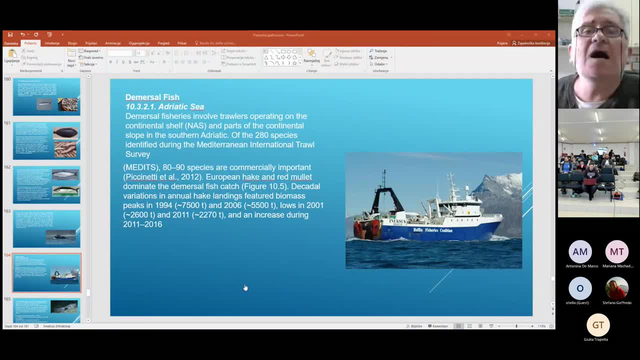 from the, from the room. i'm asking the students: okay, okay, okay. so, jacob, thank you very much for your presentation. uh, you will send us, uh to me, the powerpoint, powerpoint, the info about the, the information, this file. okay, okay, that's no problem, i will. 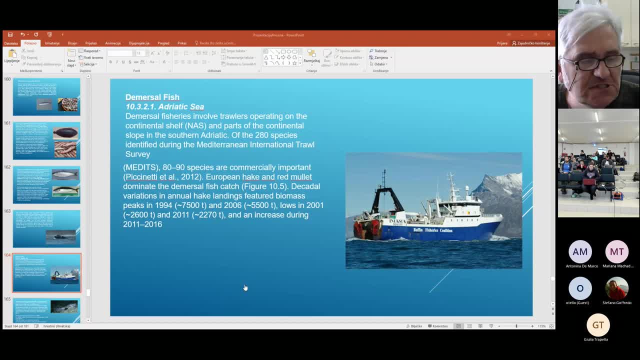 send the pro the file also presentation which is connected with the with the impact of new species into the adriatic in general, because it is very important for for me if one or two species established a population in the adriatic he could not speak about the more the problems which are. 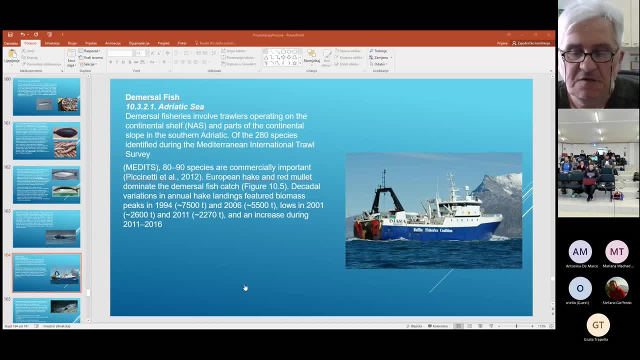 not presented, which are now actual. for example, could not speak about the impact of, for example- i don't know- resources on pelagic resources. he could speak only about one thing: about the terrorist news and their effect on the fauna on the adriatic sea. do you know what i'm talking about? 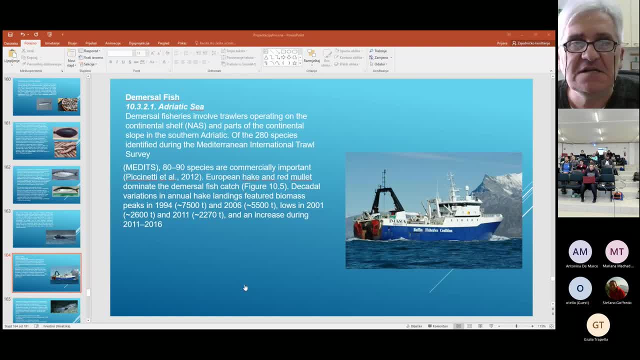 because i know that now my friends and researchers from israel, lebanon and cyprus, especially in greece. they are only speaking about now, nowadays, only about one species. all other problems disappear: how to kill this type of species, how to extract it from the marine.